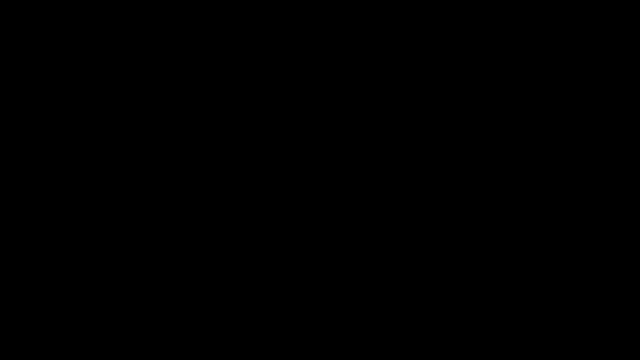 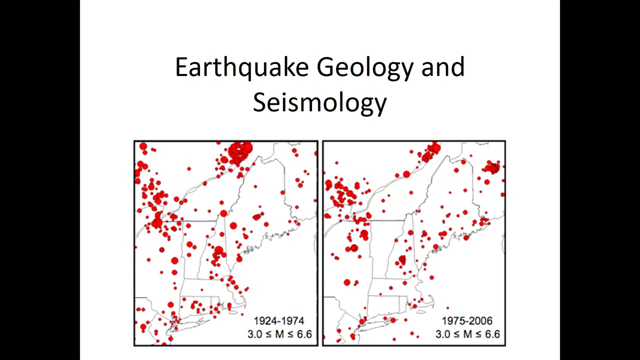 Welcome to the third lecture in our Natural Disasters course, in which we will be discussing earthquake geology and seismology. On the maps we see in this first slide, we have what we can all recognize as New England and part of New York. The red dots correspond to locations. 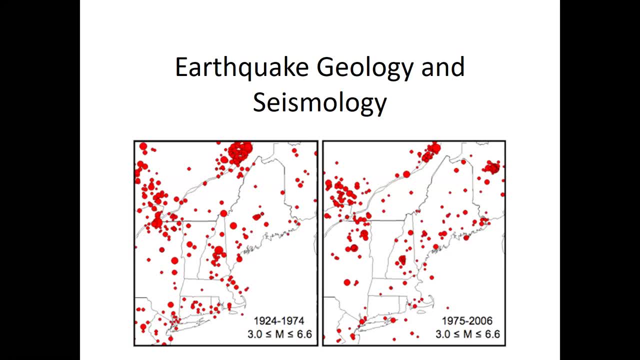 of earthquakes and the size of the red dot. its diameter is scaled to the size of the earthquake, the magnitude of the earthquake. We have two different figures: the one on the left showing those earthquakes that occurred between the years 1924 and 1974, and the figure 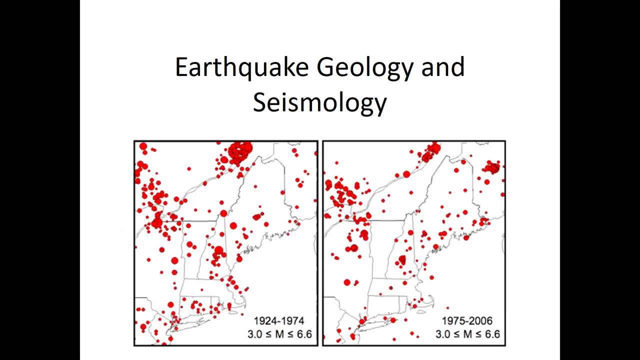 on the right showing how many earthquakes occurred in initial notification. Another: those that occurred between the years of 1975 and 2006.. Most people don't think of New England as having earthquakes, but it does, just not very long, large ones, and so it doesn't have the 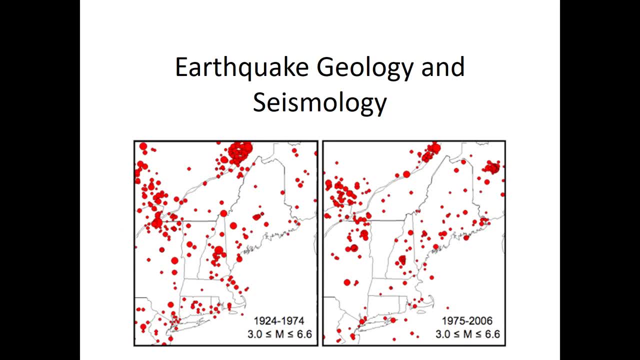 level of infamy or notoriety that the west coast of the United States does, but it does have earthquakes, and sometimes it does have fairly large earthquakes- nothing that's extremely devastating, but enough to make its presence known. I kind of wanted to start with this slide. 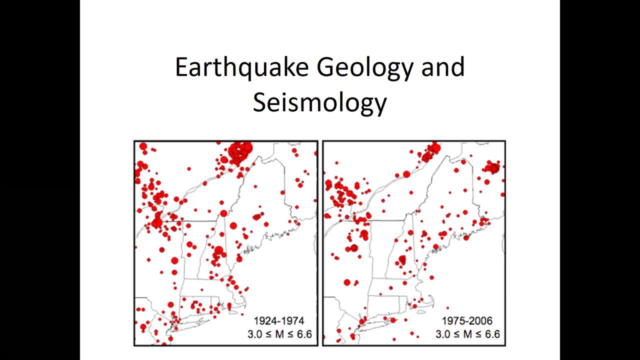 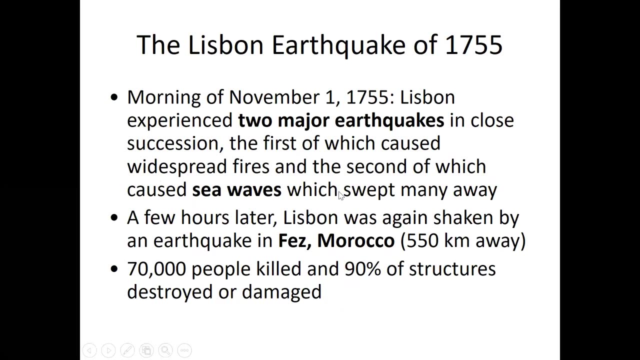 to show that earthquakes do occur almost everywhere on earth. They are not a phenomenon that is relegated to certain sections of the planet, as some may think. So an example of a very around, so an example of a very devastating earthquake was the Lisbon earthquake of 1755.. So on the morning of November 1st, 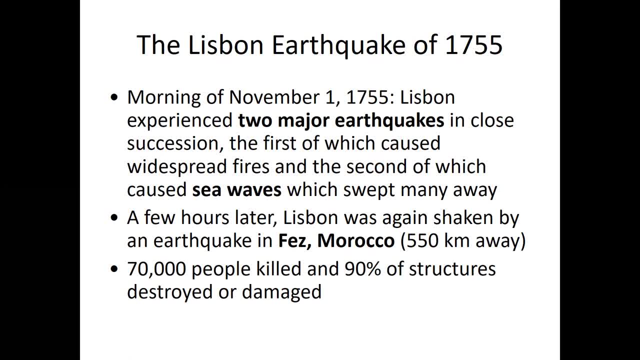 which, in the Catholic Church, November 1st is a holy day of obligation. It's All Saints Day, where the faithful attend mass, And so on. that morning, the Catholics of Portugal- which there are a lot of Catholics in Portugal- were all attending mass. 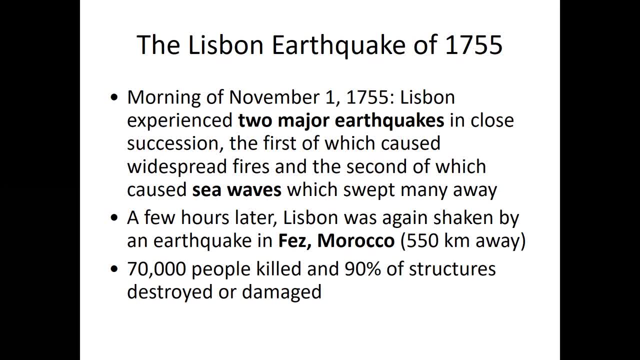 And there was two large earthquakes in close succession, And so you can imagine a lot of these stone structures, churches. they did not fare very well during the earthquakes and they failed. There was also widespread flooding, There were fires, And the second earthquake caused sea waves which we'll learn are actually. 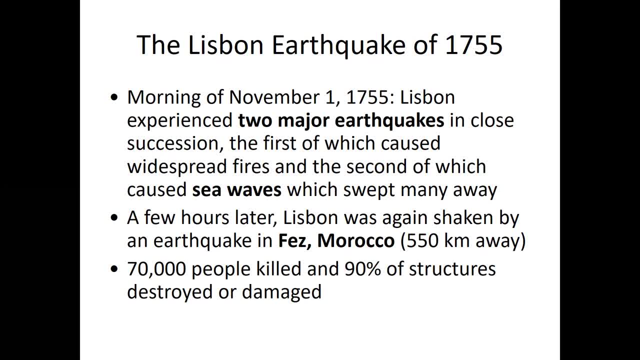 called tsunami that swept many people away. A few hours later, Lisbon was shaken again by an earthquake in Morocco- Fez, Morocco- And after all was said and done, about 70,000 people were killed and 90% of the structures were destroyed or damaged. Now the 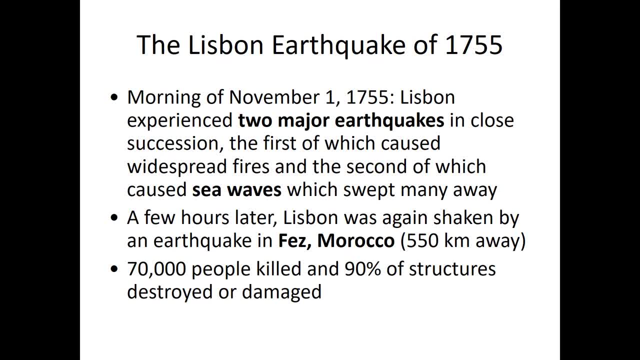 the really tough part about this event is after the earthquake, to at least after the first one. to escape the danger of the collapsing buildings and the fire, people went to the coastline, which made sense. However, the sea waves that were induced by the second earthquake 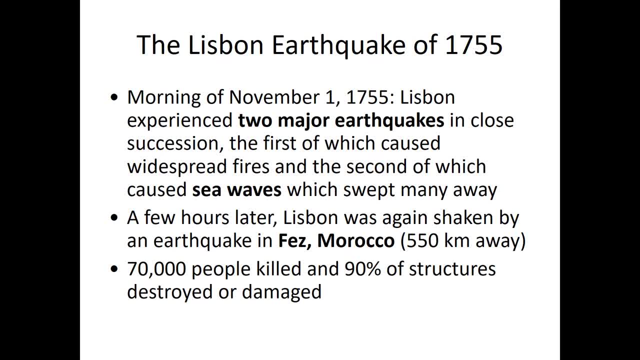 came and swept them away while along the coastline. So it's very unfortunate And I enter- I start with this because an event like this likely would not happen today. At least it should not happen today, Because we know better. we know what type of structures to build in regions that have a high 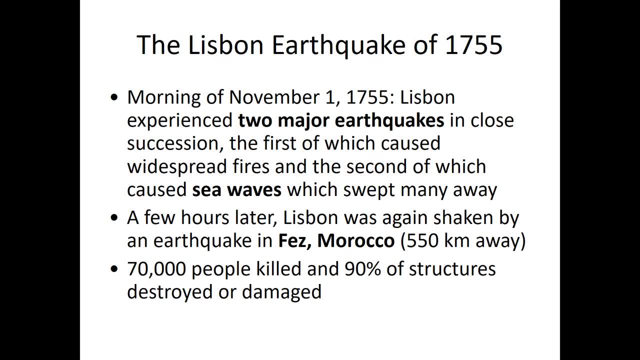 large earthquake hazard And we know the the peripheral hazards of earthquakes, such as tsunami as well. So people would not understand Bourbon limiting. You know that they continued to createLIE, but there's still a Task Force in Morocco. we're gonna do it to try spreadsheet factor to determine which areas are chosen to attack. 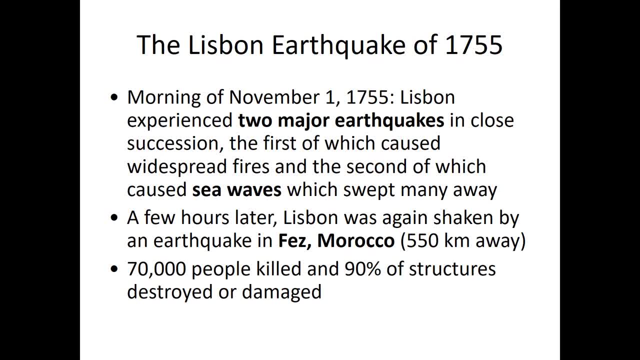 what just make sense for them- I'm not sure who, And so we did some sort of revelation to that: not go should not go to the coastline, at least if they're properly educated. So something like this in 1755, these were deaths due to natural disasters, due to ignorance, which hopefully 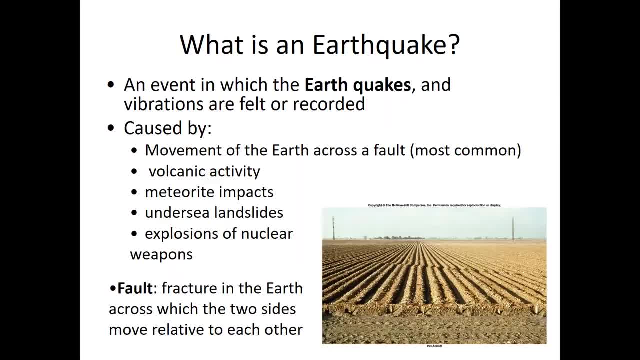 are avoidable should be avoided today. So what is an earthquake? An earthquake is an event in which the earthquakes, as its name may suggest, and vibrations are felt or recorded in the process of an earthquake. So earthquakes can be caused by several phenomena. The most common is the movement. 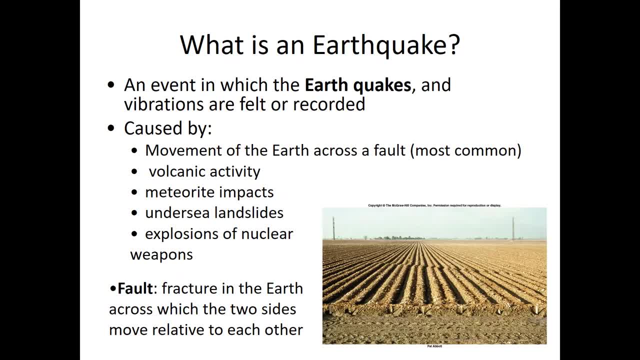 of earth across a fault. which a fault, as we'll discuss, at the very bottom. it's a fracture in the earth's surface, or not necessarily just in the surface, but in the rock near the surface. So volcanic activity could cause earthquakes, meteorite impacts, undersea landslides and 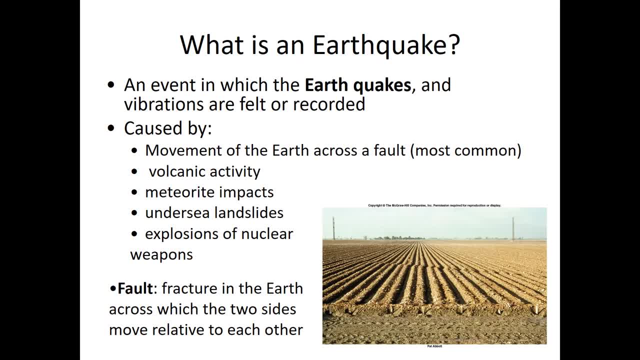 explosions of nuclear weapons And the most common earthquakes, as we've said, are in the surface. So, we said, occur along faults, And faults are fractures in the outer layer of the earth, the lithosphere in which the rock slides along. these fractures, these faults, 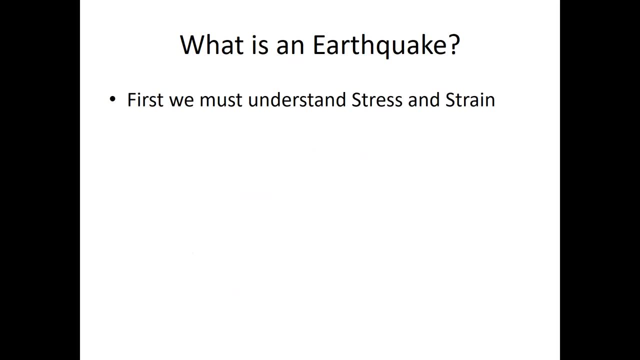 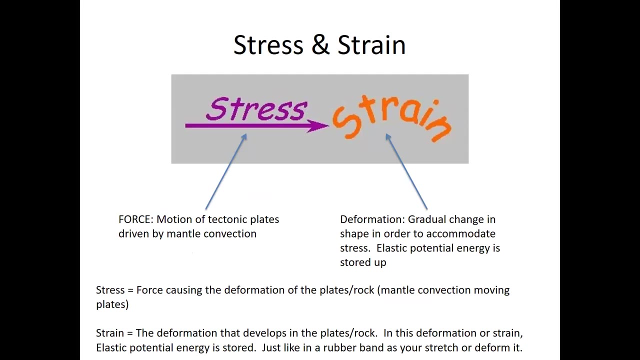 So to understand why earthquakes occur along faults, we first must understand the concepts of stress and strain. You may have heard of these words before, maybe in different contexts, But stress and strain are terms in physics and engineering. Stress is a force basically applied in particular. 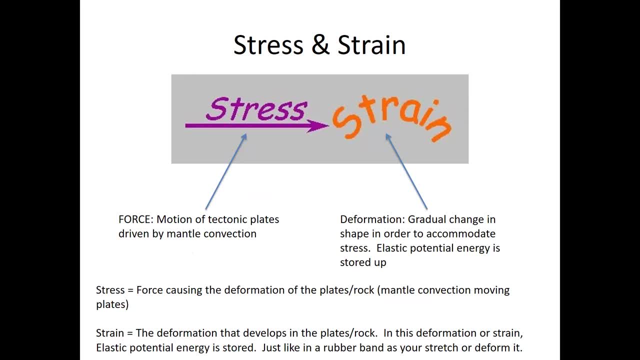 a force applied to an area, But it's a force And in this situation, a case of earthquakes, a force is being generated by the motion of the tectonic plates, And those tectonic plates are being moved by the mantle convecting beneath them And the motion of these plates results. 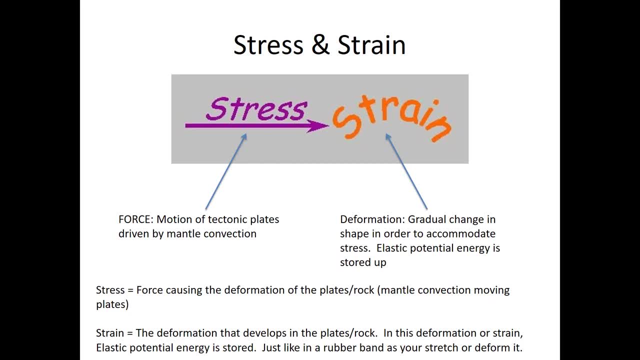 which generates the stress, results in what's known as strain. Strain is a deformation or a change in shape. So strain is a gradual change in shape in order to accommodate the stress. And we said there's different ways in which materials can deform. 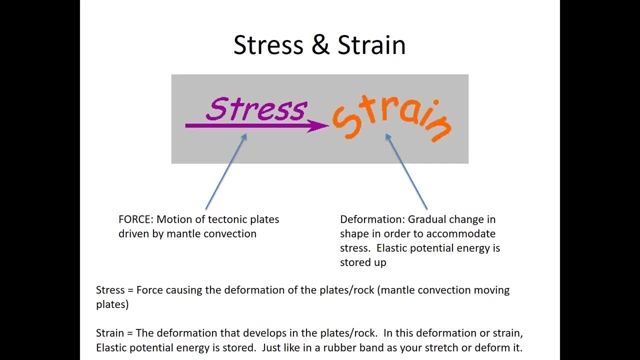 There is elastic, ductile and brittle. If the material undergoes elastic deformation, then as it deforms, as strain accumulates or as it deforms, energy in the form of elastic potential, energy is stored in the material. So stress, as we said, stress in this situation is the force causing the deformation of the plate. 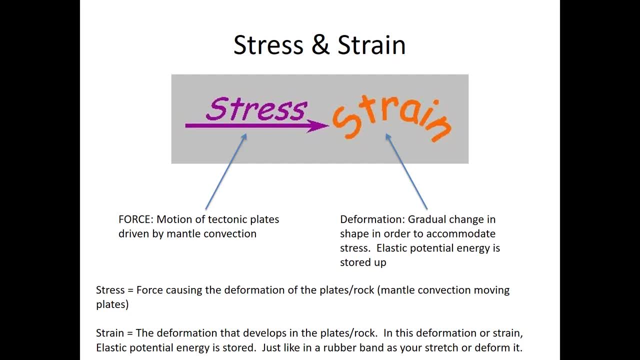 Slash rock, which is ultimately comes from the mantle convecting, And the strain is the deformation develops in the plate, slash rock- And in this deformation or strain, elastic potential energy is stored. So think of when you stretch a rubber band, you are applying a stress to it. 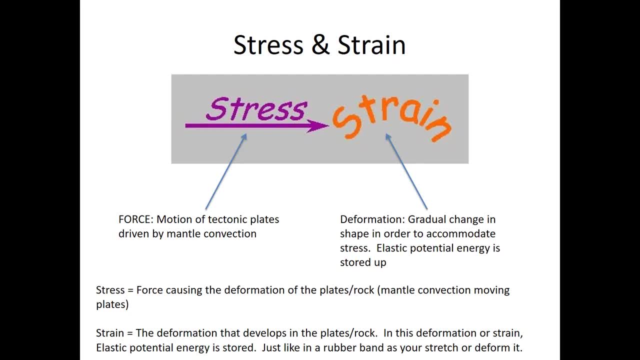 You are stretching it, You're applying a force and stretching it. That's the stress. Well, as a result, the rubber band accumulates a strain, It deforms, It stretches And because that strain or deformation is elastic, elastic potential, energy is stored in it. 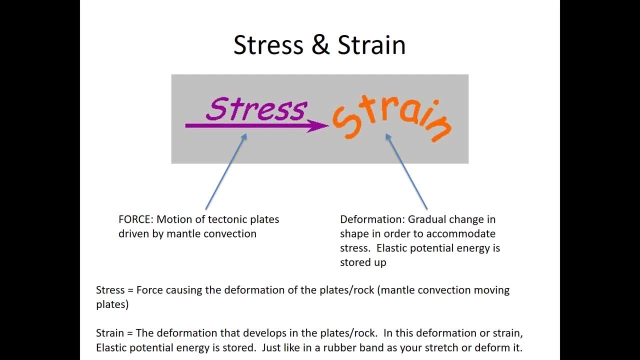 And if you let go of that rubber band, that energy is released and it snaps back. And I think of a slingshot. You put a projectile and a slingshot and you pull it back. You are applying a stress to the rubber band. 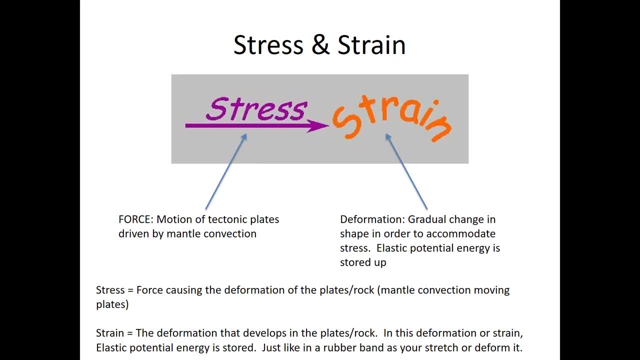 The rubber band goes to deformation And elastic strain. It stores energy, elastic potential energy. You let go of it, The elastic potential energy is released. So that stored energy is released In the case of a slingshot, it's transferred into the projectile and it launches the projectile. 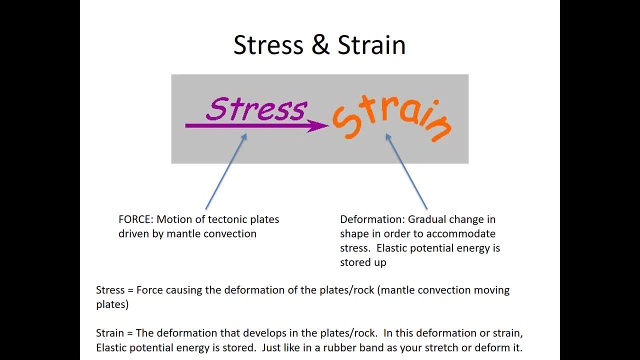 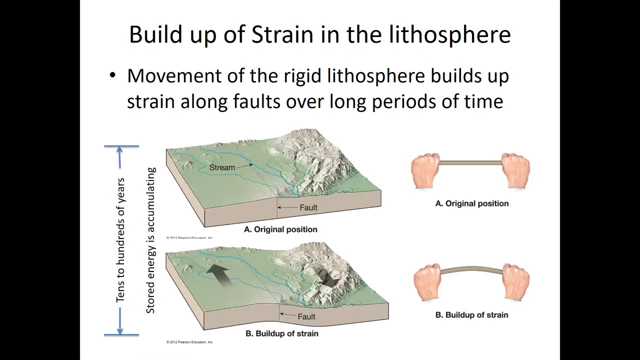 So whenever stress deforms an object and the object undergoes elastic deformation or elastic strain, energy is stored up in it. That's very important, The fact that energy is stored in it, So as the plates they're moving. At the plate boundaries, which we find faults, the plates are moving in different directions. 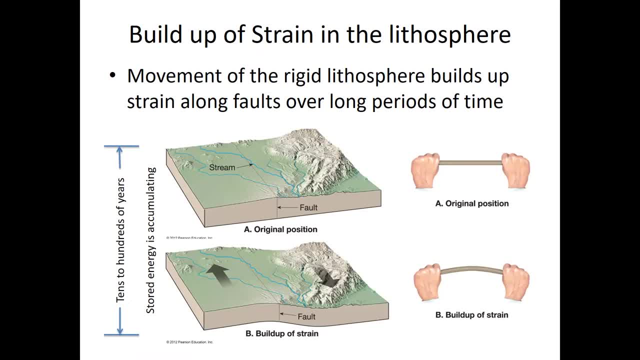 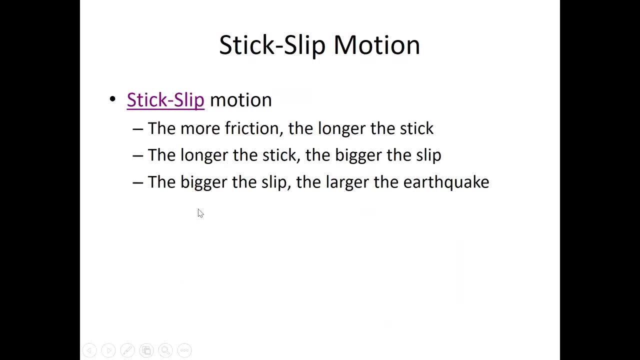 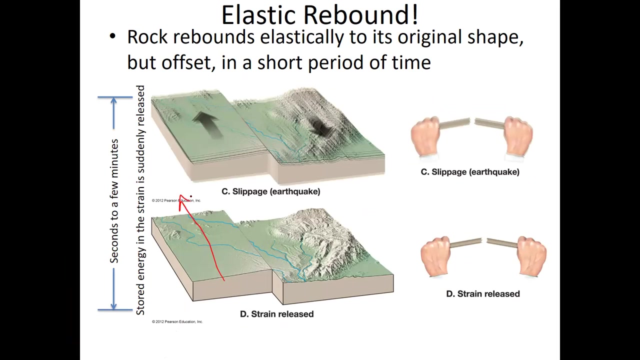 And because the plates are moving in different directions, the rock deforms around the fault. So, as you can see here, this rock is moving. Oh, My pen doesn't seem to be working. This rock is moving this way while this rock. oh, I'm on the wrong slide. 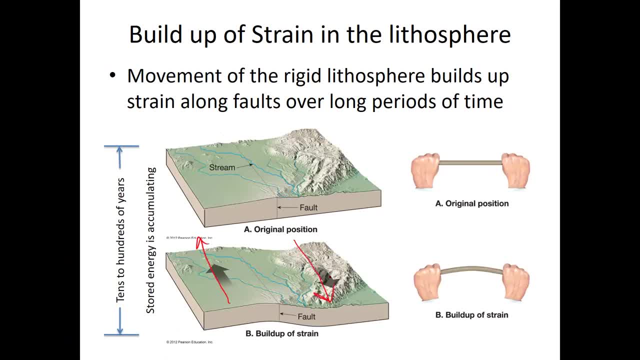 This rock is moving this way. while this rock is moving this way, And you can see how this rock was- This rock was originally undeformed. As a result of this motion, the rock is deformed, It changes shape. Now, this process of the stress causing the rock to deform it takes a long time. 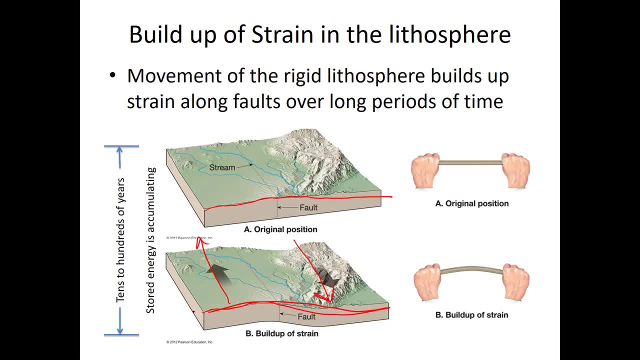 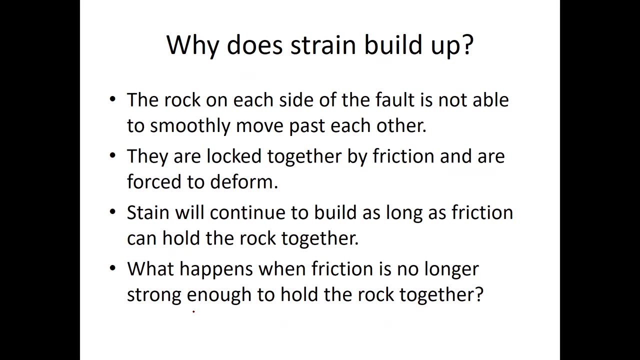 So this phenomenon occurs over the timescale of tens to hundreds of years. As the rock slowly deforms, it is storing elastic potential energy. But why does the rock deform and why is this strain allowed to build up? Why does the rock just not simply slide past each other along the fault? 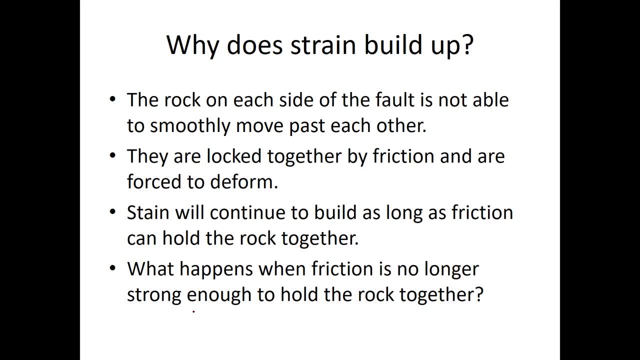 Well, the rock is not able to slide along the fault because the two sides of the fault, the rock on both sides of the fault, are locked together by friction, And that friction, which is a force, holds the two faces of the fault together, which results in the rock having to deform. 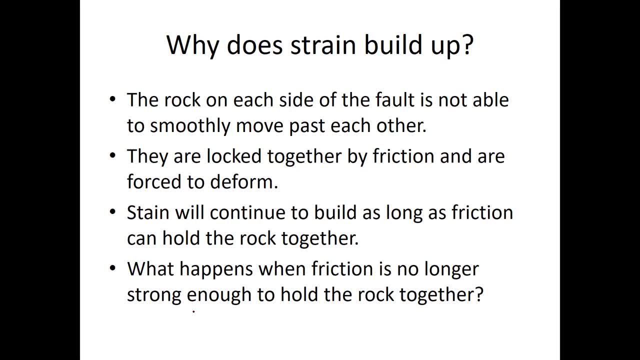 And so strain will continue to build and accumulate, and therefore energy will continue to accumulate as long as friction is strong enough to hold the two faces of the rock together. What do you think happens when the friction is no longer strong enough to hold the rock together along the fault? 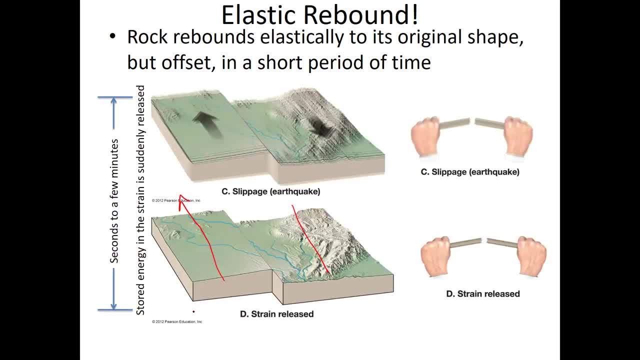 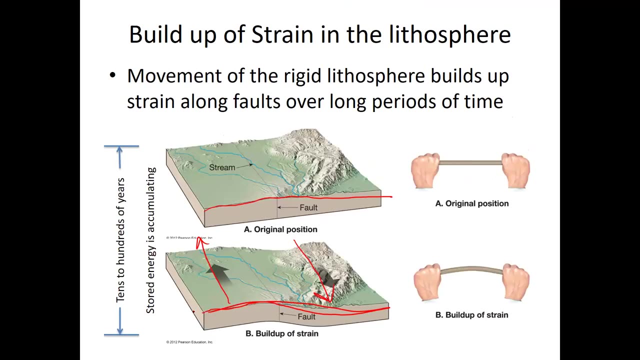 Well, all that energy that has been stored in the form of elastic potential energy is released as the rock quickly and suddenly snaps back to its original shape in a process known as elastic rebound. So the rock gets deformed. So this rock is going to want to snap back this way. 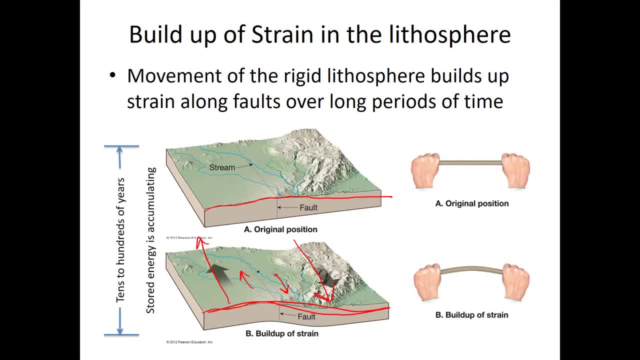 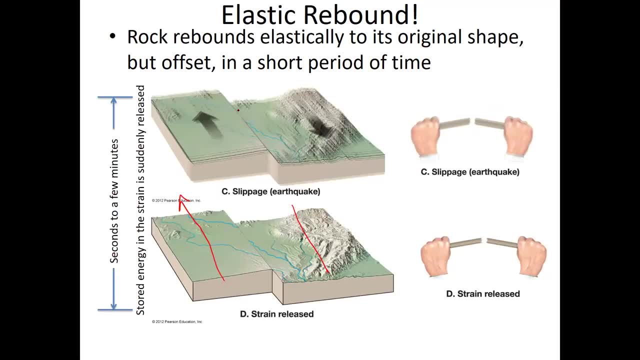 This rock is going to want to snap back that way, And as it does, it returns its original shape. All that stored energy is released, and the energy travels through the earth in the form of vibrations, as we'll learn, known as seismic waves. 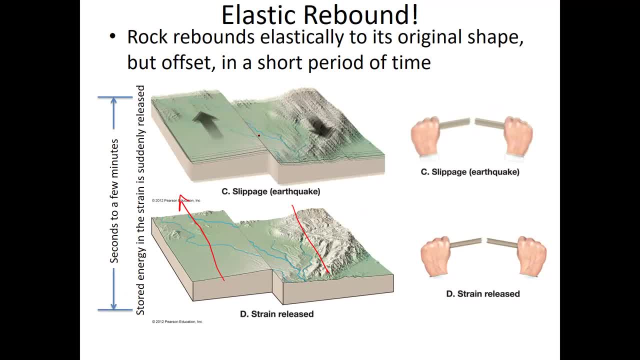 So this is very similar to you stretching a rubber band, And so, And eventually, you stretch it so much that you can no longer hold it with your fingers. It slips through your fingers. Friction between your fingers and rubber bands is no longer strong enough to hold it in between your fingers. 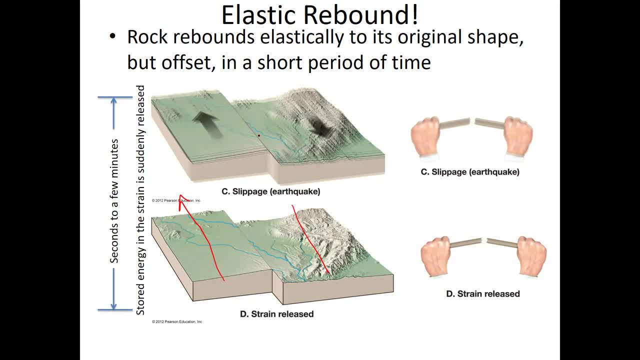 It slips out and snaps back, And so, where the process for the rock to deform and accumulate all that energy took tens to hundreds of years, this process of elastic rebound, where the fault slips and the rock returns this original shape and all that stored elastic potential energy is released. 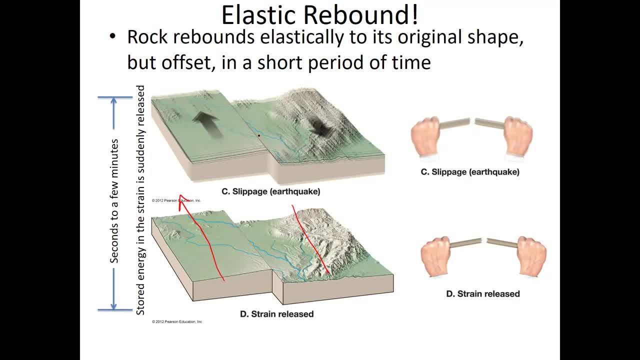 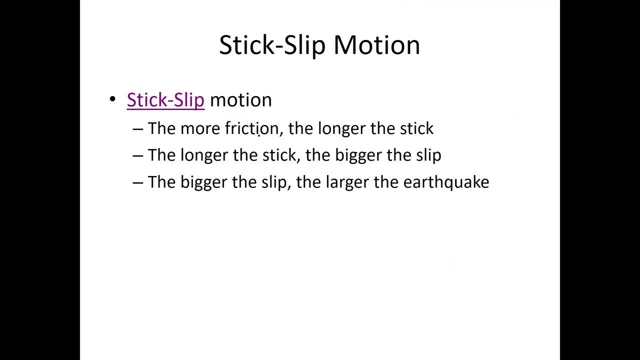 that process takes seconds to a few minutes, And so it took a very long time to store all the energy. The energy, all the energy is released in a very short period of time, resulting in an earthquake. So this process is called stick-slip motion, because the fault is stuck together due to friction. 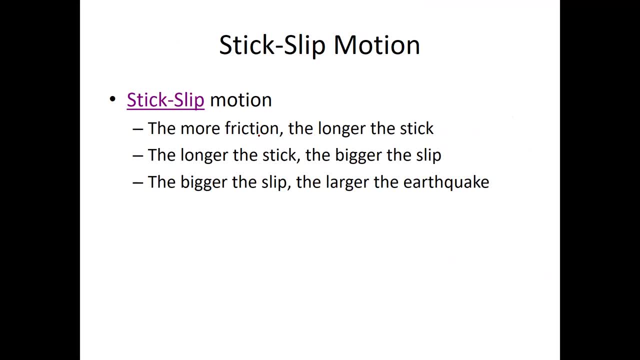 and eventually it slips. And then, once the slip is over, then the process repeats itself. The thing is, if they're the, How frequently the fault slips determines the size of the earthquake, right? Because if there's a lot of friction in the fault, then the rock won't slip very often. 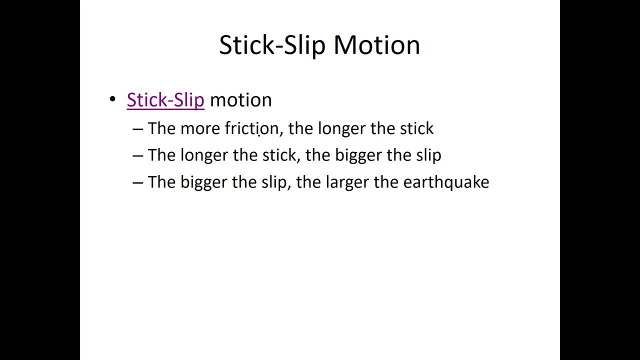 And, as a result, large amounts of energy can accumulate because the rock will undergo a lot of deformation And then, finally, when the rock does slip, there'll be a large amount of energy to be released. So you have very infrequent but large earthquakes. 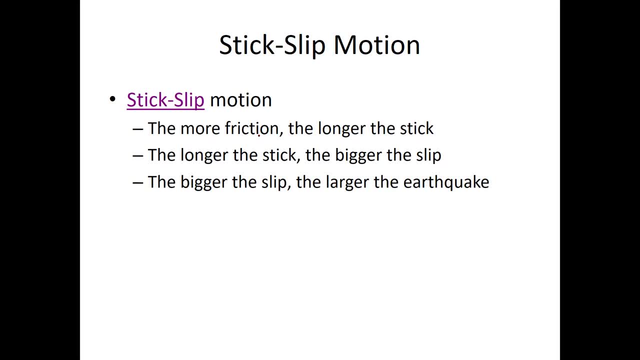 Whereas if there is very little friction in the fault, then the fault ruptures or it slips very frequently. But because it's slipping very frequently, there was not a lot of time for significant amounts of energy to be stored, And so small amounts of energy released. 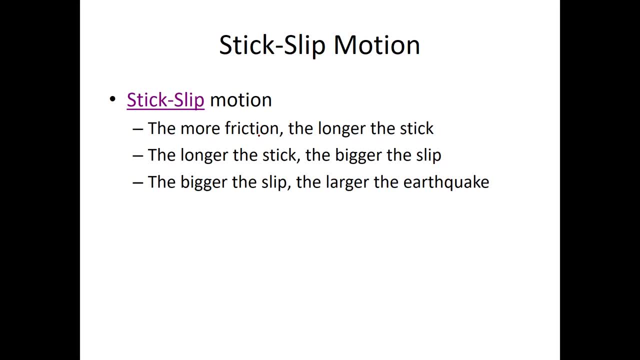 So you have very frequent small earthquakes. So the more friction, the longer the stick. The longer the stick, the bigger the slip. The bigger the slip, the larger the earthquake. Now this video illustrates this motion. So these are blocks resting on the surface. 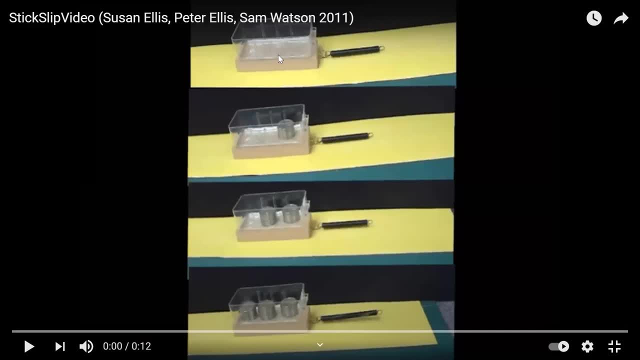 And these blocks are a physical model for this process of stick-slip motion. So where the block is in contact with the surface, that represents the fault. Now there's friction between those two surfaces that wants to hold the block in place. That's the friction and the fault. 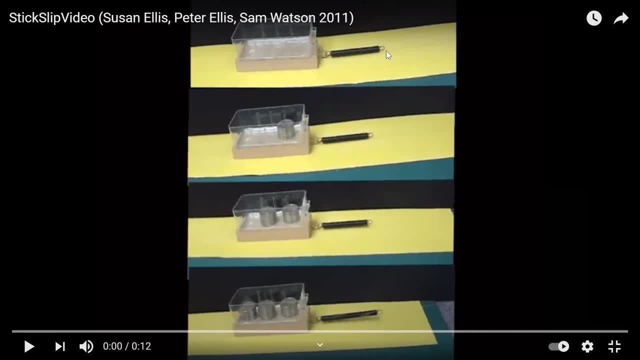 Now, attached to each block is a spring, And attached to each spring is a string. It's hard to see the string, But in each of these the string is going to be pulled at a constant rate. Now the pulling of that string is analogous to the motion in the plates. 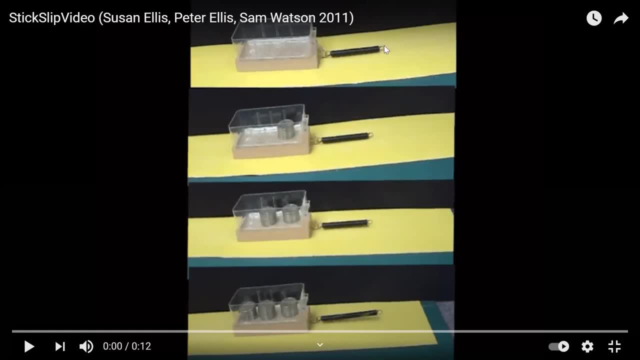 That's the stress. Now, as you pull the string, what happens is friction wants to hold the block in place. So if the block's not going to move but the string is going to be pulled, something has to give, And that is the spring. The spring stretches. That's the deformation, That's the elastic strain. And as the spring stretches, more and more, more energy is being stored in the spring Until, eventually, the friction is not strong enough to hold the block in place anymore and the block slips. 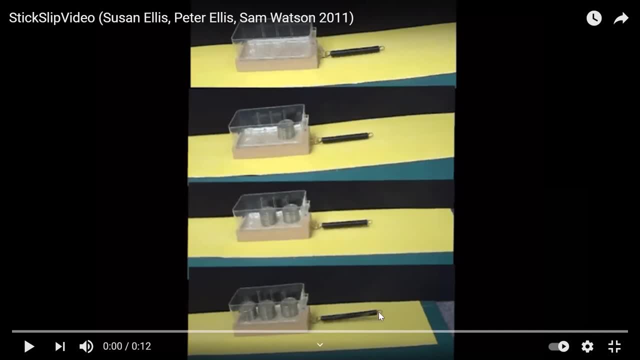 And as it slips, all the energy in the spring is released And it lurches. It just yanks the block forward And that sudden motion of the rock or of the block generates the earthquake. That's the earthquake. So you can see. there's four different blocks. 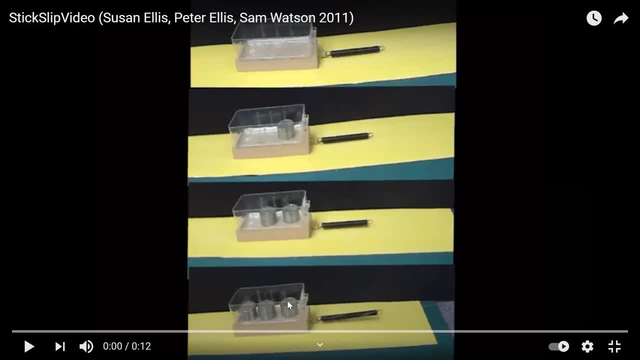 and each of them have a different amount of mass sitting on top of them. That's to vary the amount of friction. So the more mass, the larger the weight, the more friction. So there's the least amount of friction in the top block. 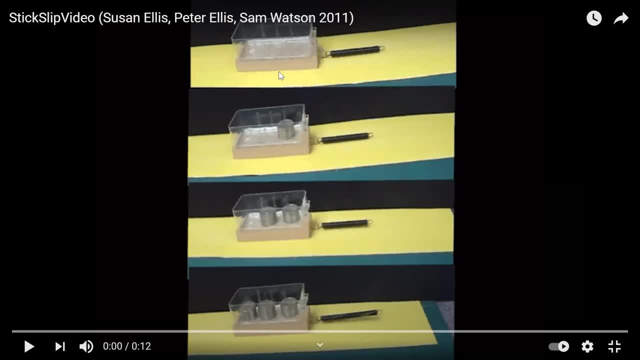 and the most amount of friction in the bottom block. So, like we said in the previous slide, with very little friction we expect very frequent but small slips, the top one- And for the more friction we expect less frequent but larger slips. 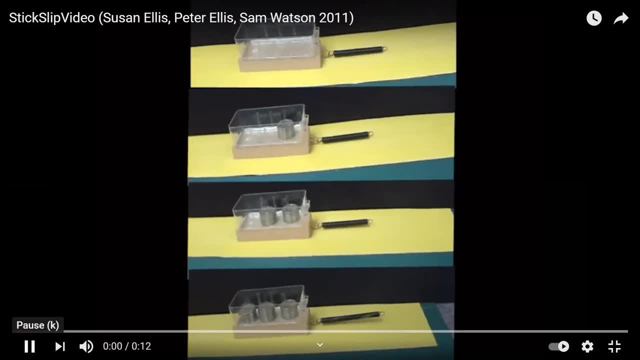 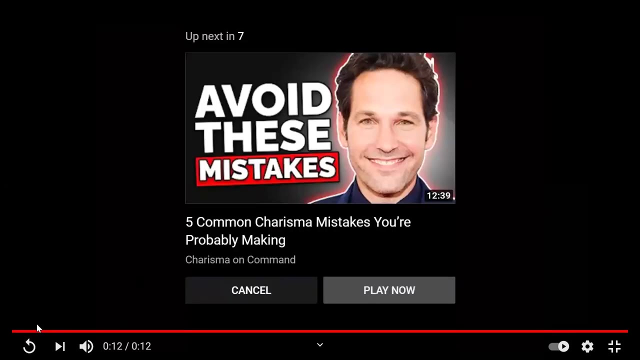 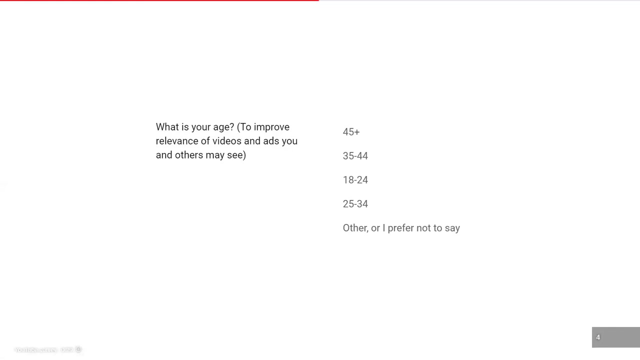 the bottom one. Let's see if that plays out as expected. See very frequent small slips for the top one. The bottom one slips less often. When it does slip, they're larger. I'll watch that one more time If I can get it to replay. 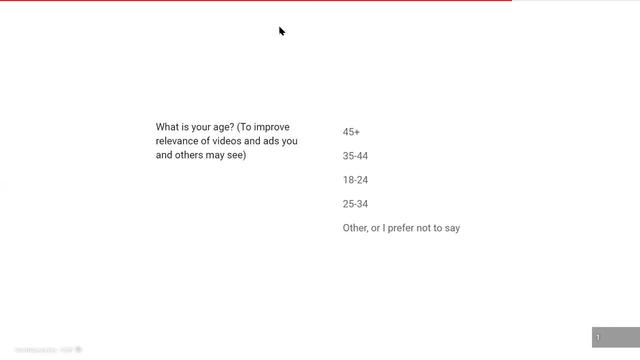 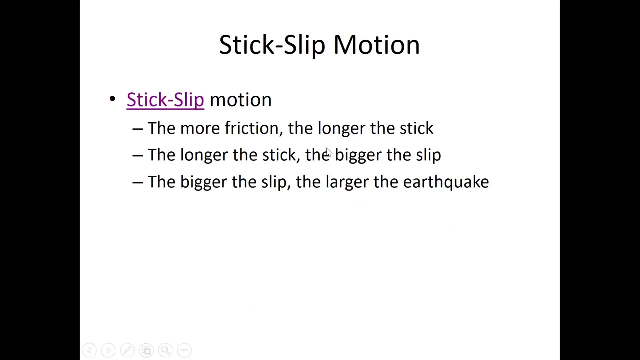 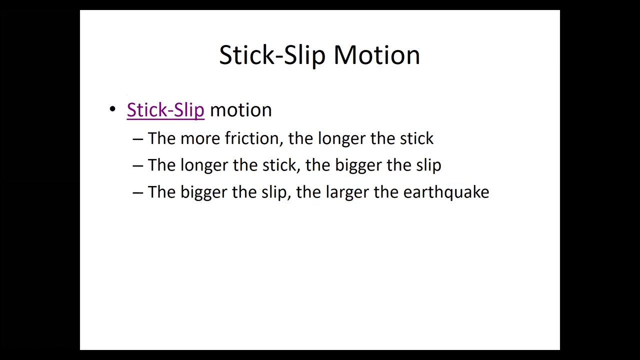 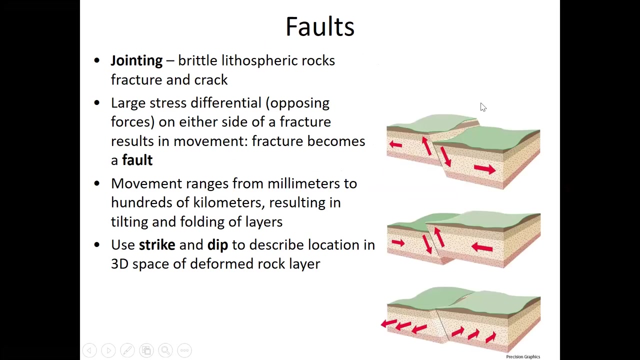 No, I guess not. Okay, Sorry, Just dealing with YouTube. All right, So that's thick slip motion. So, going back to faults. So how was a fault created? A fault was created by a process known as jointing, which is the brittle deformation of lithosphere rocks. 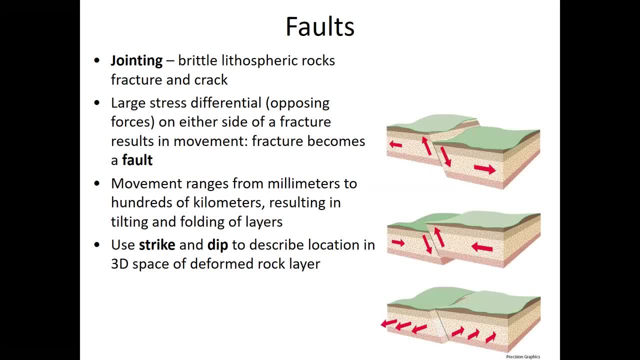 Remember, brittle deformations are when it breaks, it cracks or fractures. So rock is deformed elastically in the lithosphere to a certain point and then it will eventually break, which creates a fault, And so large stress differentials, which is forces in opposing directions. 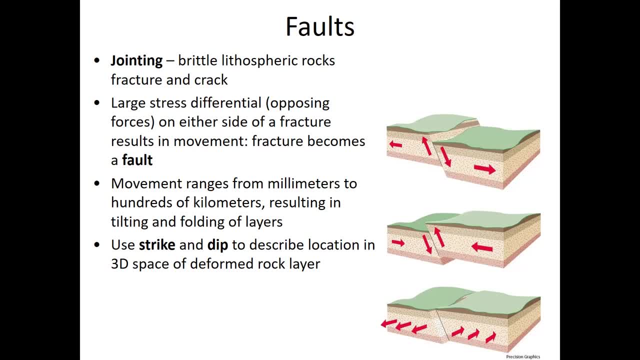 on either side of a fracture or fault results in the movement of rock in different directions along the fault, And so this movement can range from millimeters to hundreds of kilometers, resulting in the tilting or folding of layers. And to orient these faults 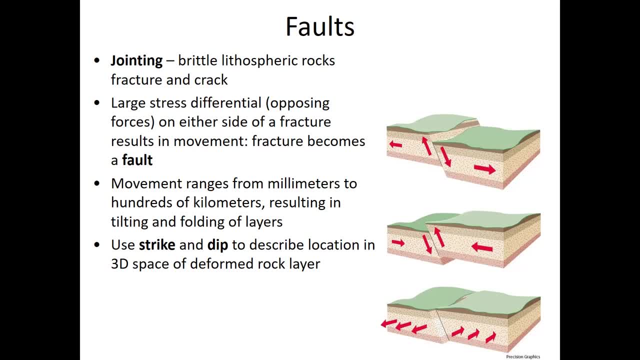 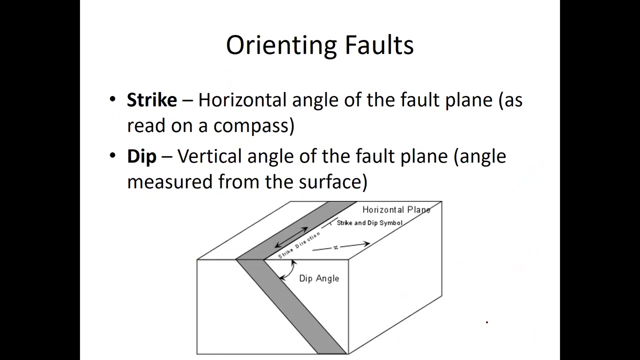 which you can imagine as surfaces or planes beneath the surface. Let's see This is a fault plane here. You can see that plane would extend Back there. We use what's called the strike and the dip angle to orient the fault. So the strike angle is: 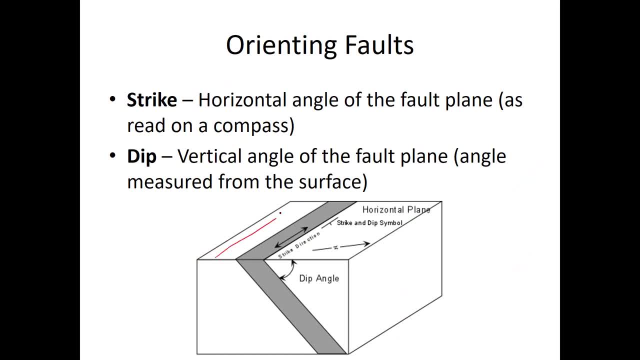 So let's say: this is the surface here And this is the fault plane, This is the fracture right here, this plane And this is the angle of the strike. Let's see A little delay between my pen, my actions. I apologize for that. 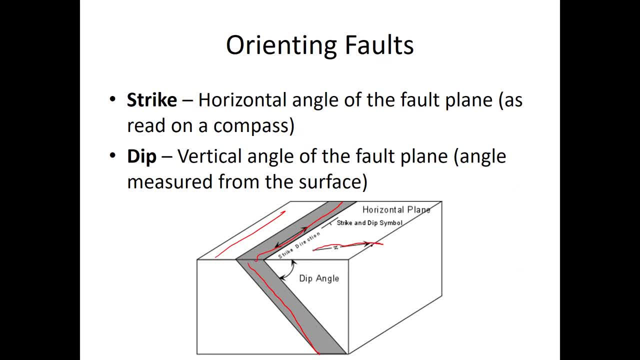 So the strike is the angle between due north and the line where the fault plane intersects the surface, which is this line right here, So this angle right there. So let's say, if this line lined up with due north, the strike would be zero. 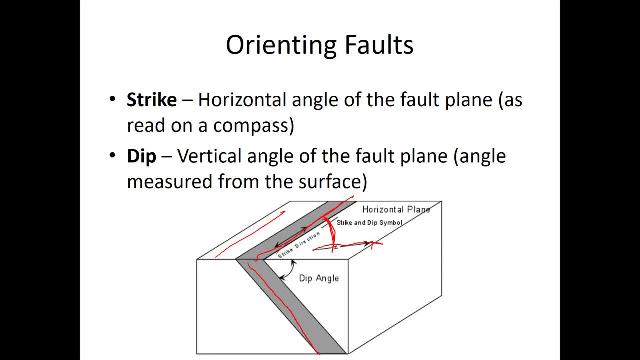 If it was running east-west, the strike would be 90 degrees, Where the dip angle is the angle in which the fault plane makes with the surface, And so it's this angle right here. That's the dip angle. So the dip angle can range anywhere from almost zero. 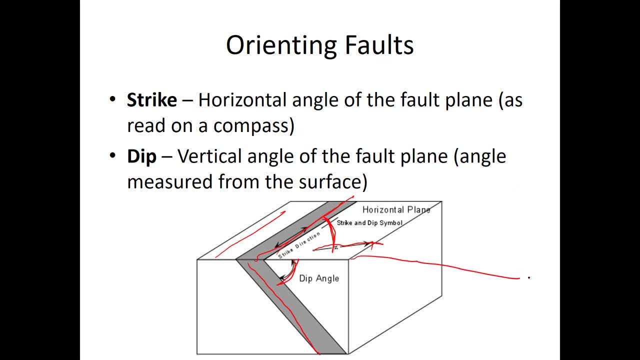 That would be a very shallow dip. Fault plane would go down like that, Or it can go to 90, where the fault plane just goes straight down, straight down like that. So it'd be a 90 degree dip. So the dip angle is the angle measured between: 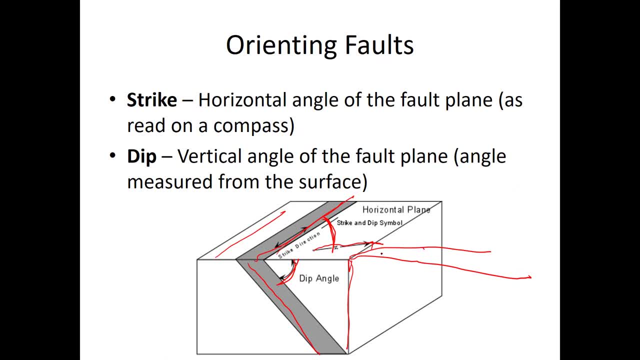 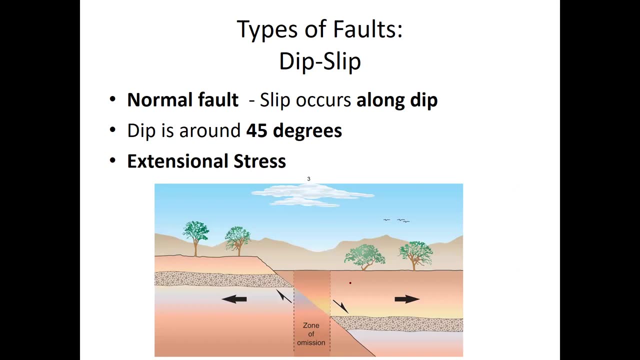 the surface and the fault plane, The angle right there. So the strike and the dip. Now we characterize faults mainly by the type of motion that occurs along them, And there's two main types. There's the first, which is the dip-slip fault. 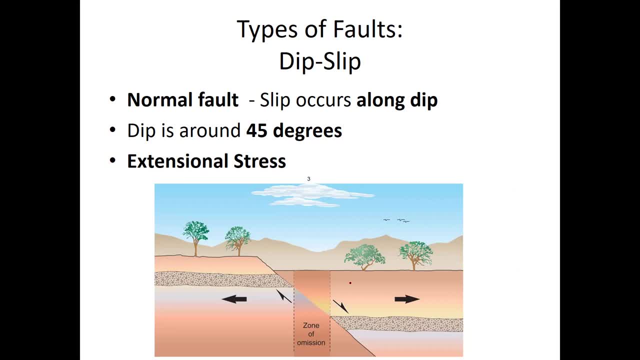 Dip-slip fault, And so these faults have a dip usually around 45 degrees. So you can see how the fault plane is around 45 degree angle beneath the surface, And with dip-slip faults the rock slides up or down, So it's in the direction of the dip. 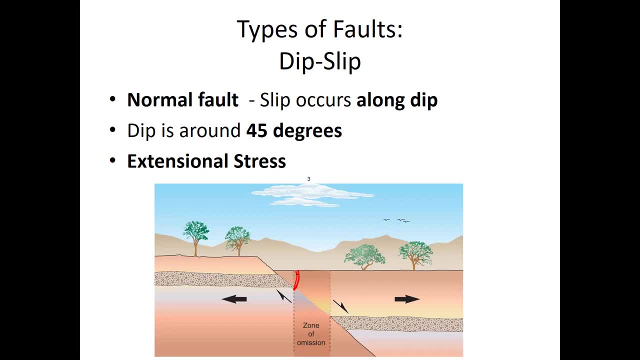 And the first type of dip-slip fault is what's known as a normal fault, And normal fault results from extensional or tensional stress where the rock is being pulled And, as a result of being pulled, the rock below slides up and the rock above slides down. 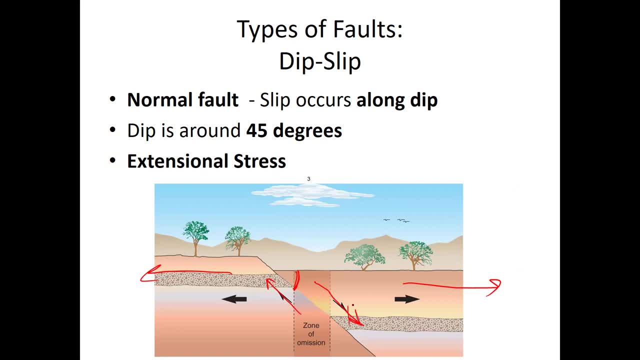 Now we have better names for the rock below and the rock above that make it a little bit more easy to follow, And it's that they- if you can imagine yourself walking down this fault plane- And people did Lost all my drawings, And people did because people used to mine. 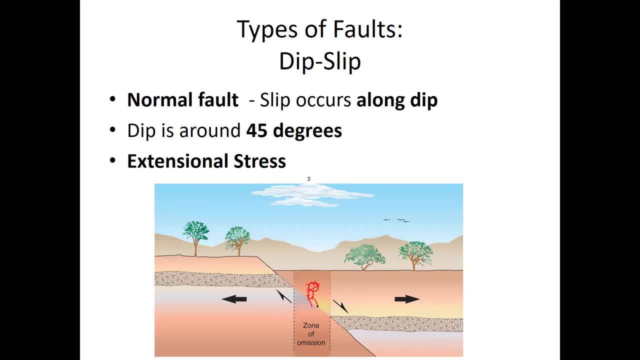 down faults, although they still do, And so the rock that you're walking on is called the foot wall- That's the rock down here, And the rock that's hanging over your head is called a hanging wall, And so I don't know why my pen's 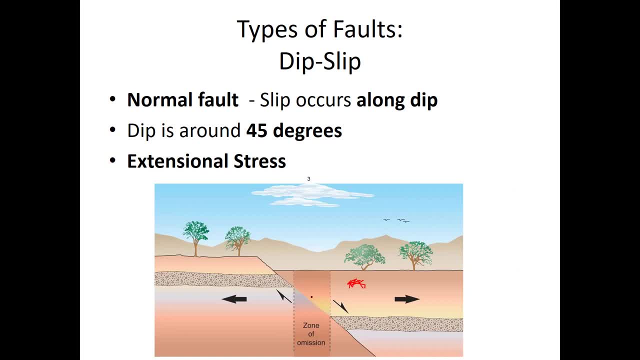 acting all wonky. So in a normal fault the foot wall slides up while the hanging wall slides down, And that's the result of extensional or tensional stress. So we're going to find normal faulting around divergent plate boundaries where the rock is being pulled apart. 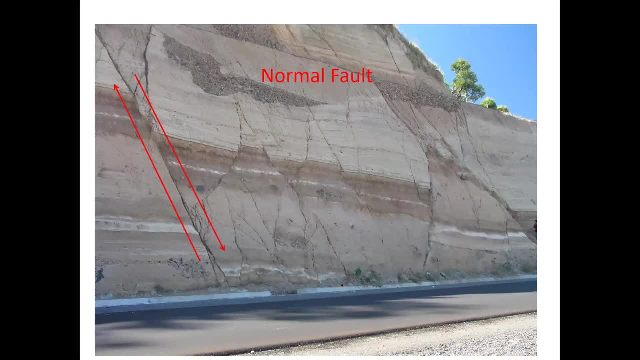 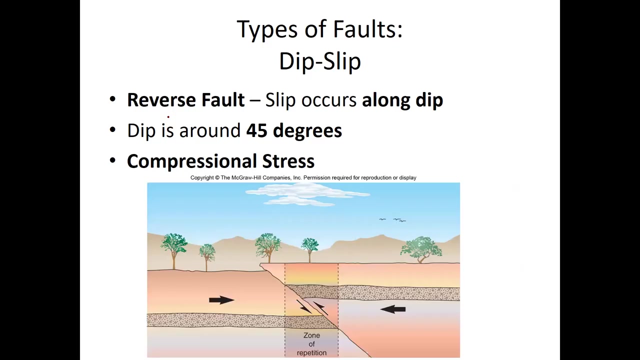 So you can see an example of a normal fault here in this cutout on the roadside. You can tell, because this layer of rock here, how it has been shifted: The foot wall has slid up while the hanging wall has slid down. The other type of dip slip fault. 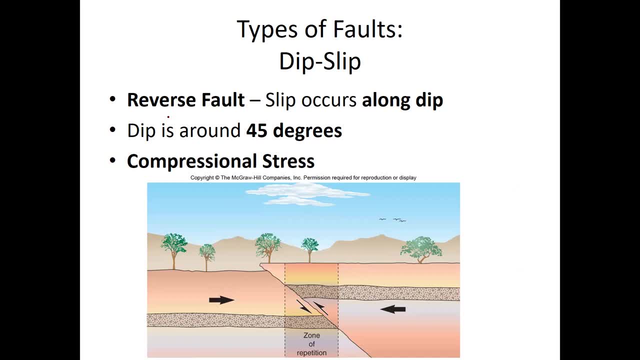 is known as a reverse fault, And a reverse fault occurs under compressional stress, where the rock is being pushed together And the motion of a reverse fault is well the reverse of that of a normal fault. It's where the foot wall slides down. 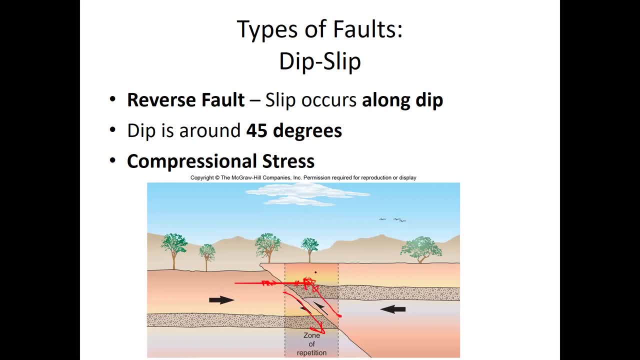 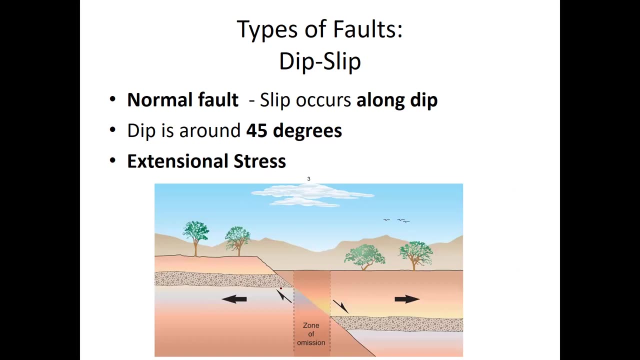 and the hanging wall slides up, And this overall results in a shortening of the rock, while the normal faulting- I forgot to mention- results in an extension or lengthening of the rock, where reverse faulting results in a shortening of the rock. 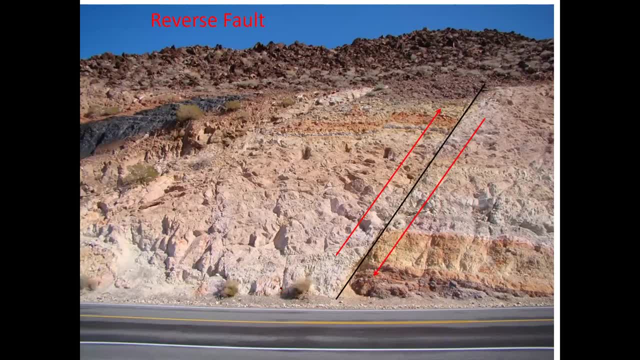 Here you can see an example of a reverse fault. You can see how this layer, this layer, this has been shifted up: hanging wall shifted up or the foot wall slid down. That was not likely one earthquake. That was maybe several earthquakes. 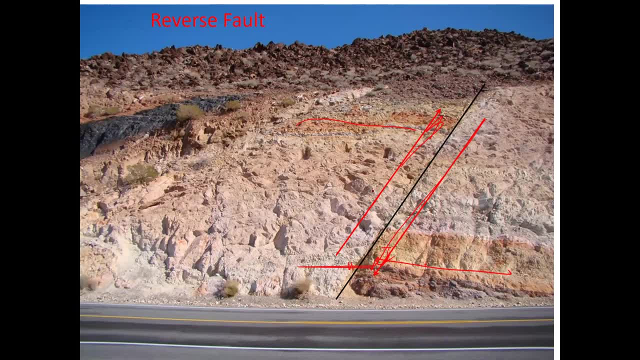 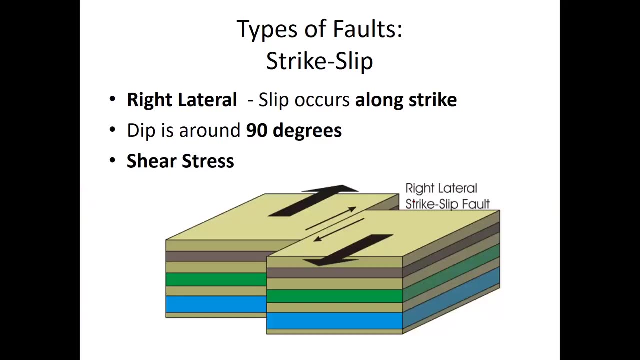 That eventually, you know, these layers probably started, probably started right there And after one earthquake it maybe slid up a little bit, slid down a little bit, another earthquake. So this has probably been many earthquakes to result in this offset in those layers. 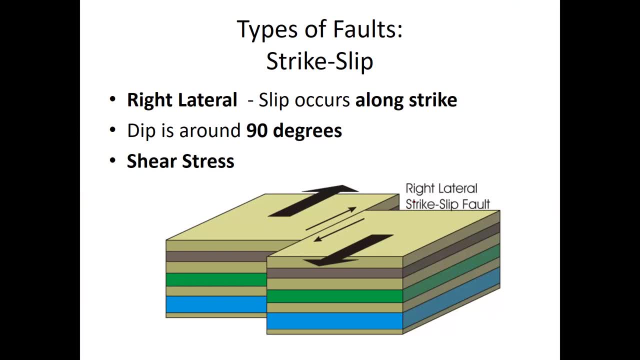 So we have dip slip faults, which include normal faults which result from extension or tension stress, and reverse faults, which result from compressional stress. Forgot to mention that we would expect to find reverse faulting near convergent plate boundaries, where the rock is being pushed together. 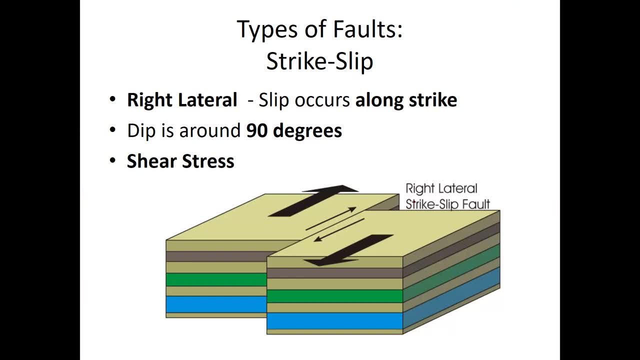 Then we have the other type of fault, which is called a strike slip fault, And a strike slip fault is where the motion is along the strike And, unlike dip slip faults, which tend to have dips around 45 degrees, strike slip faults tend to have dips around 90 degrees. 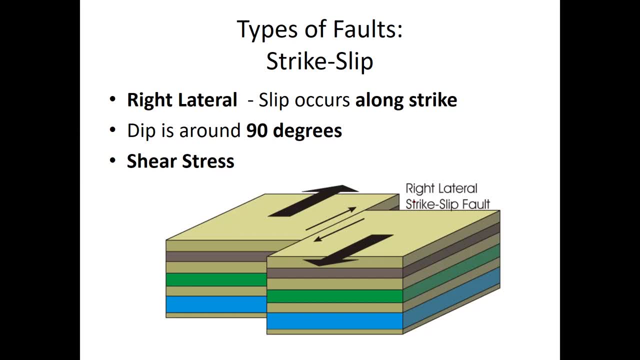 So the fault plane usually goes straight down into the ground, And so strike slip faults are the result of shear stress where the rock is sliding past each other, And so we tend to find these types of faults along transform plate boundaries. Now, this type of strike slip fault, 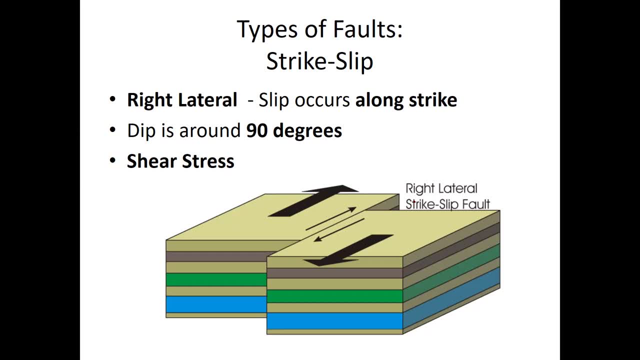 in particular, is called a right lateral, because the right side is moving towards you. So if you imagine yourself standing here with one foot on one side, one foot on the other, one foot on the other, the right side is moving towards you. if you're facing that way, 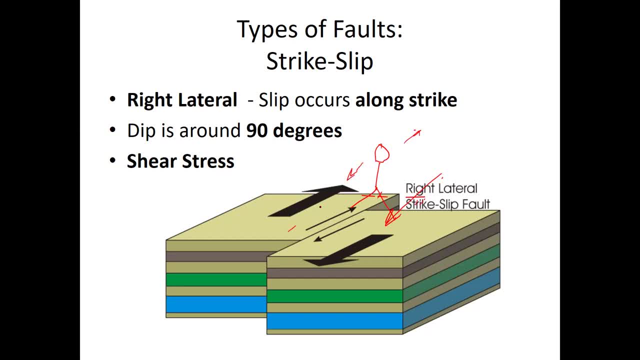 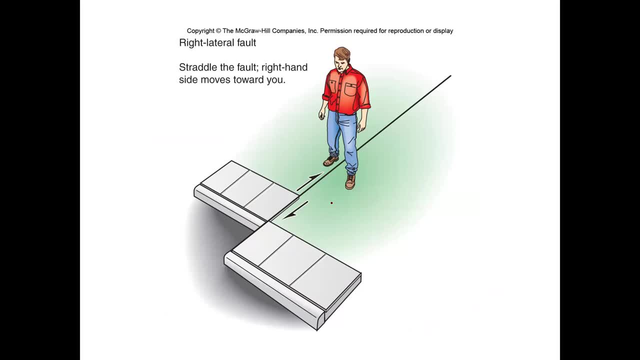 Even if you turned around and you're facing this way, the right side, your right side- still moves toward you, As this person is demonstrating. the rock on their right is moving toward them. The rock on the left is moving away from them. 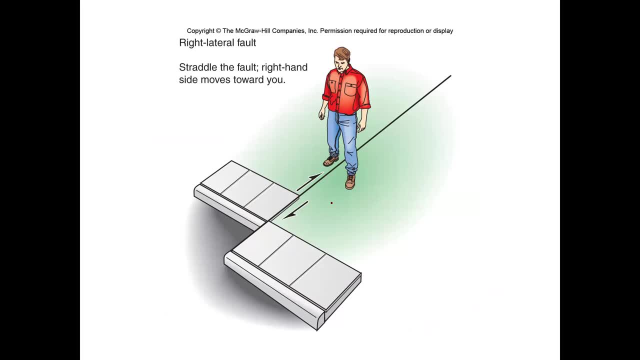 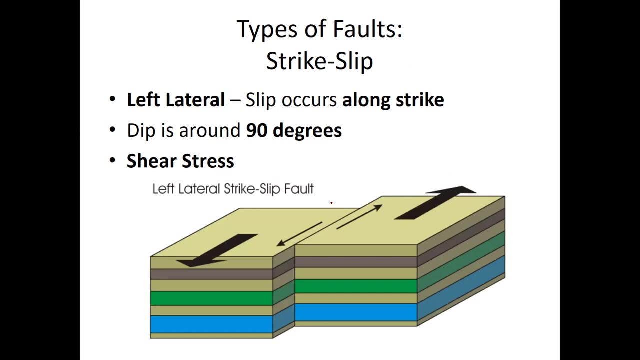 If they would turn around, they would still experience the same thing. The rock on their right is moving towards them, The rock on their left is moving away from them. It's called a right lateral And the other type of strike slip fault is just the opposite sense of motion. 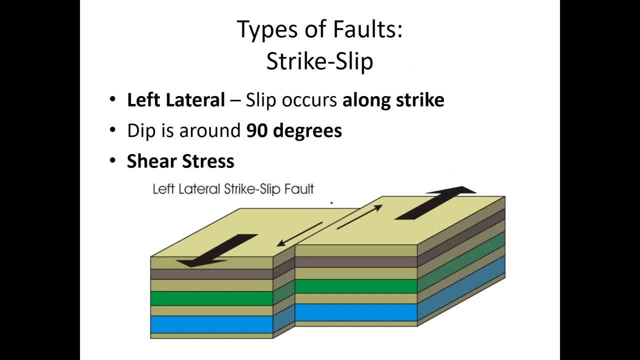 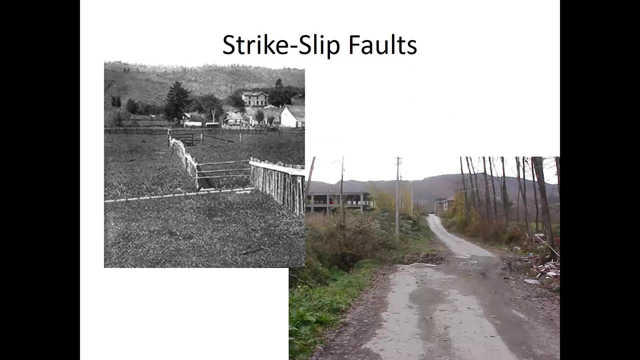 left lateral, where the left side moves towards you and the right side moves away from you. Here's some examples of the offset of rock due to motion along a strike slip fault. So this fence used to be connected and probably ran down through here, and which each subsequent step. 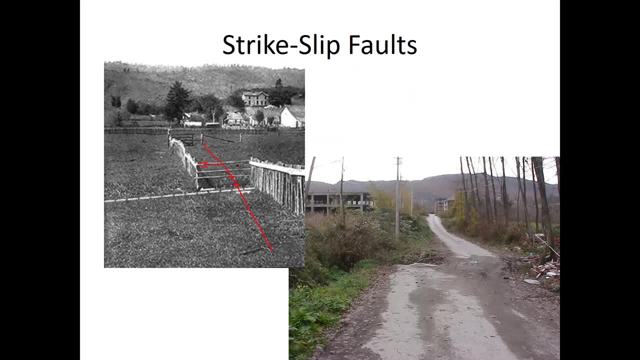 of the earthquake, this moved that way and this on this side moved that way, And so you could see that this is a left lateral fault, because the left side would move towards you, the right side moves away from you, And then here another thing. here is the fault line. 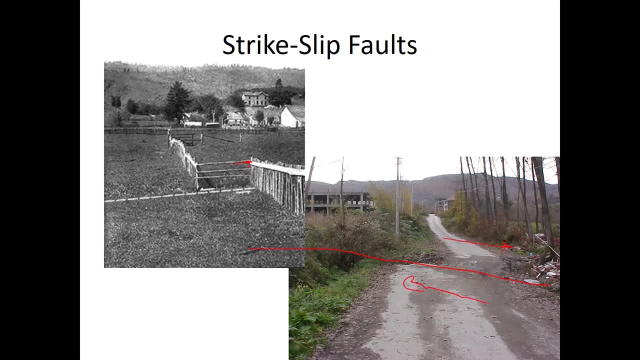 So this side is moving this way. this side is moving this way, So this is a right lateral. Interesting thing is this road was once straight and it was built on the deformed rock going across the fault. Whenever the fault slipped, the rock returned to its original shape. 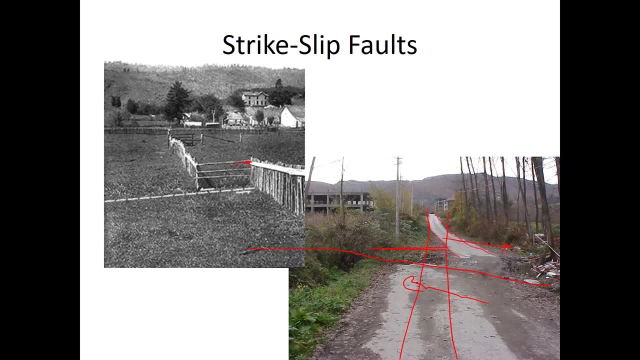 which now results in the road appearing curved. But it's not that the road was originally curved. the road was straight. It was just built on curved or deformed rock. When the earthquake occurred, the rock returned to its original shape, therefore bending the road. 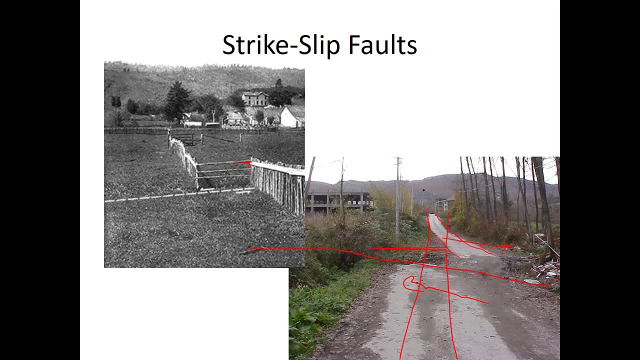 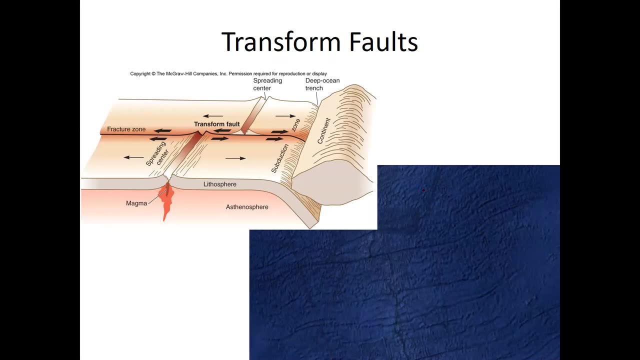 which is really cool to see, And so, as I said, these strike-slip faults typically occur along transform plate boundaries, where the plates slide past each other, And most transform plate boundaries are along our little connecting segments, along divergent plate boundaries on the sea floor. 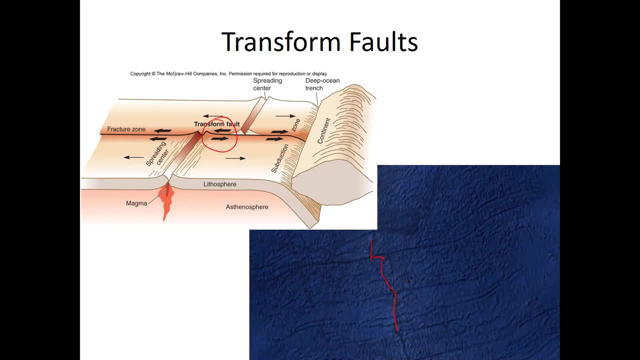 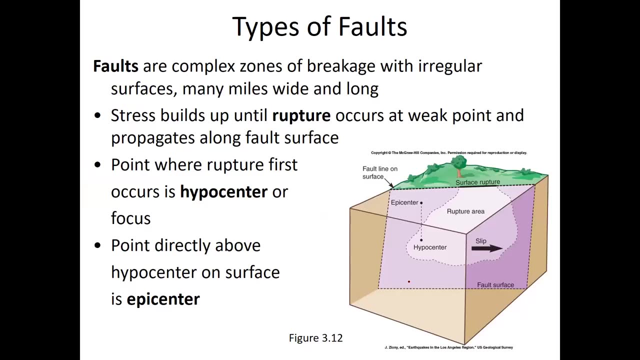 But there are a few transform faults that are on land and are much larger, and they're fairly notorious for earthquakes. So faults are not just these simple cracks that are flat surfaces. They are complex zones of breakage with irregularly shaped surfaces, And they're many miles wide and long. 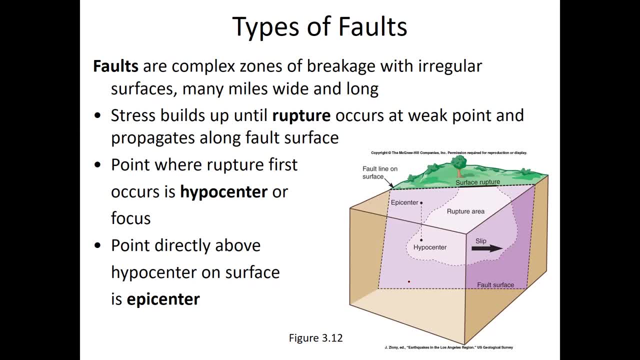 So the stress and strain they build up along the fault until rupture occurs, which rupture is whenever friction is overcome and it begins to slip or slide. And this rupture occurs at the weakest point on the fault, where the friction is the weakest, and then it propagates along the fault surface. 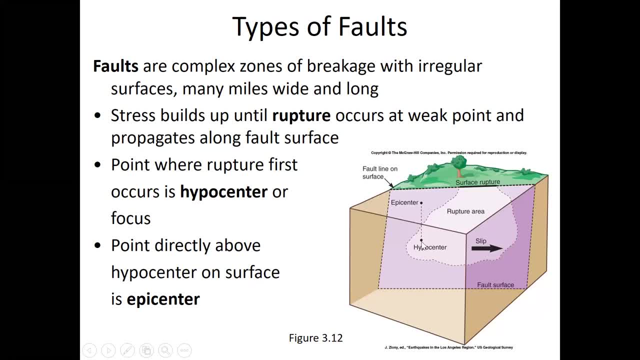 The point along the fault where the rupture occurs is known as the hypocenter. So if we see this figure here, the darker purple shaded plane, that's the fault. The lighter shaded region, that's the area of the fault that slipped, So not the entire fault slips. 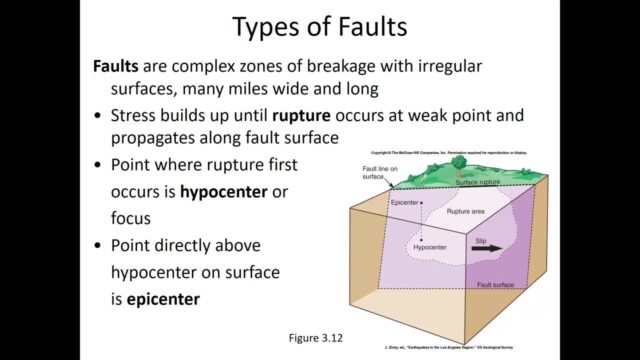 a certain area, region of it, slips. That was the rupture area, And where that rupture initially began is known as the hypocenter, And you see that in this case the ruptured area reaches the surface And so you can see you actually have some offset. 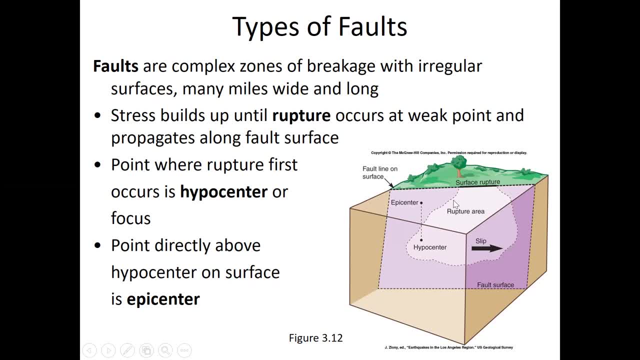 in the ground, at the surface. But that's not necessarily the case for all earthquakes. Sometimes the ruptured area does not make it to the surface, And so there's actually no visible sign of the offset at the surface. So we said the location of where the rupture begins. 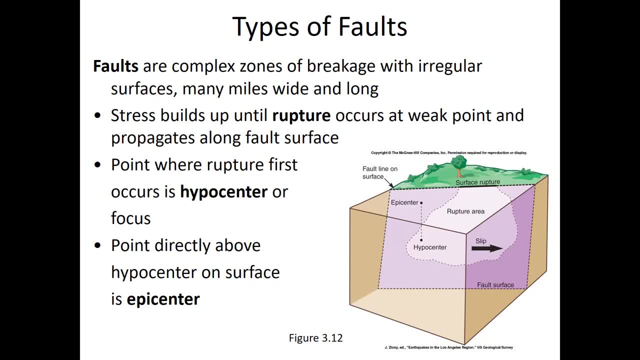 is known as the hypocenter. That is actually what we consider the location of the earthquake. For convenience, we project that location up to the surface. We call that the epicenter of the earthquake. So the epicenter of the earthquake is not actually where the earthquake occurred. 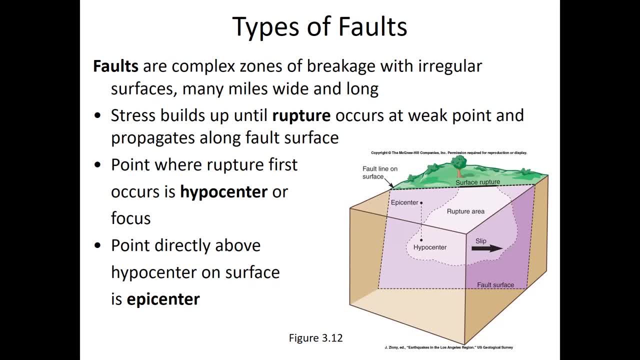 It's the point on Earth's surface directly above where the earthquake occurred. And a quick way to remember the difference between the two is that hypo, like in hypothermic means below, And so hypo center is location below the surface. 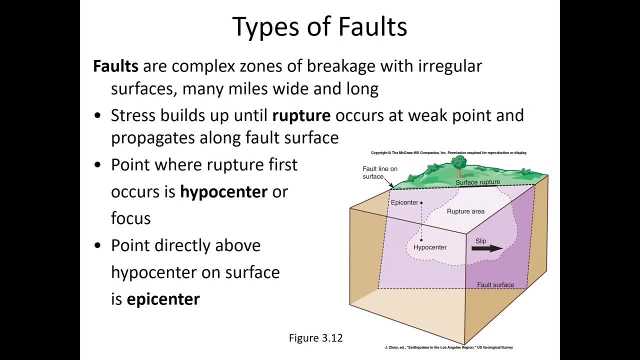 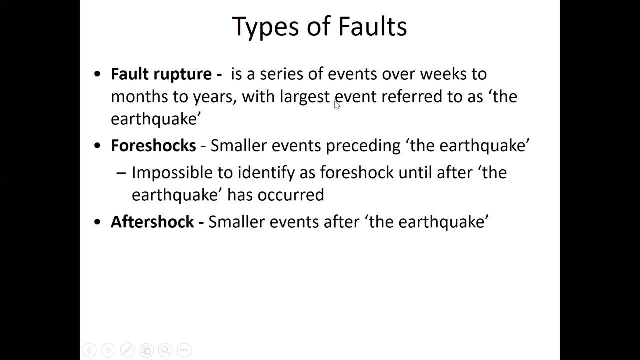 Epi. epi means outside, like your epidermis, your outer layer of skin, And so the epicenter is the location of the earthquake at the surface. So this process of rupture is never a simple one-off event. Rupture actually is a series of events. 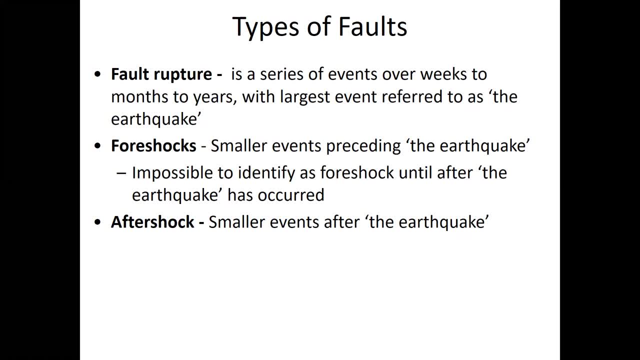 over a particular time period, either a couple weeks or months, even years, where there are multiple slips, with the largest slip being referred to as the earthquake or the main shock. There could be smaller slips or smaller earthquakes that precede a bigger earthquake. of the sequence. 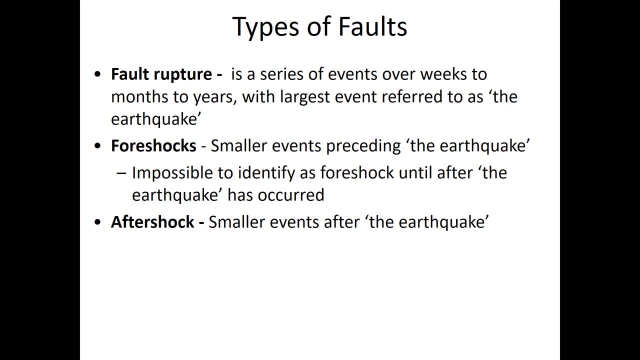 the biggest earthquake of the sequence, the main shock, And those are known as foreshocks. It is impossible to identify an earthquake as a foreshock until a large earthquake has occurred, in which all those preceding earthquakes are then a priori considered to be foreshocks. 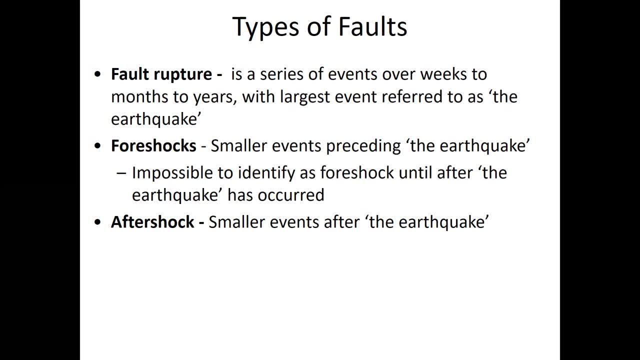 Aftershocks, on the other hand, are easily identified. After a large earthquake, smaller earthquakes occur, and those earthquakes are known as aftershocks. There are not always foreshocks for a large earthquake. Some large earthquakes occur with no smaller earthquakes. 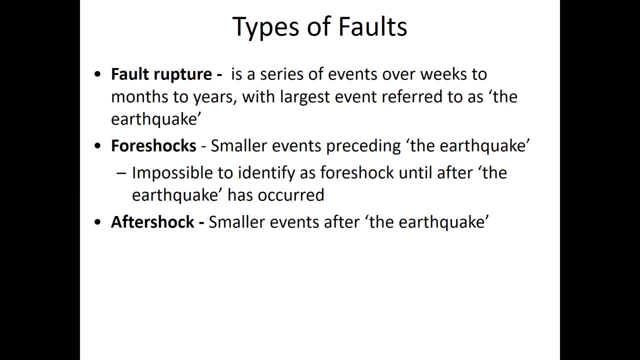 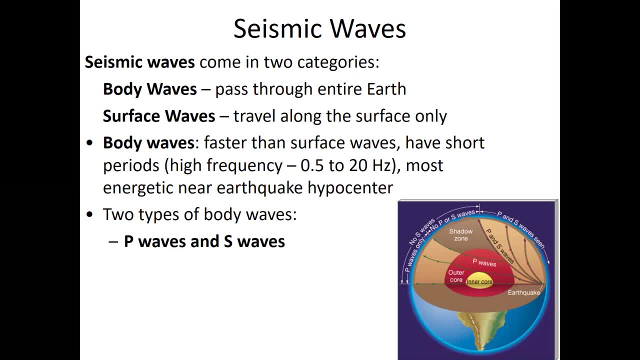 preceding them, But there are almost always aftershocks. So when an earthquake occurs, the stored elastic potential energy is then released and travels through the Earth, along its surface and through its interior, in the form of seismic waves, And there are two primary types. 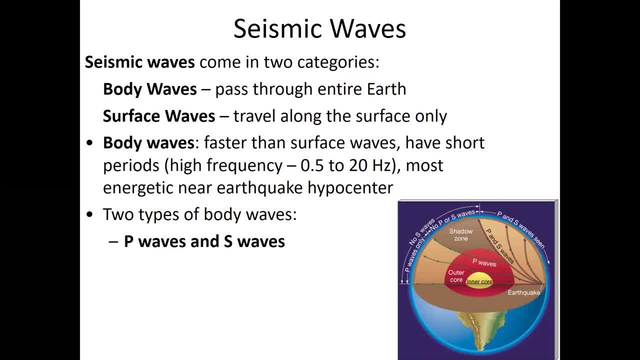 of seismic waves: body waves, those waves that travel through the interior of the planet, and surface waves, those waves that travel along the surface alone. So body waves: they're faster than surface waves and they have short periods, which corresponds to high frequencies. 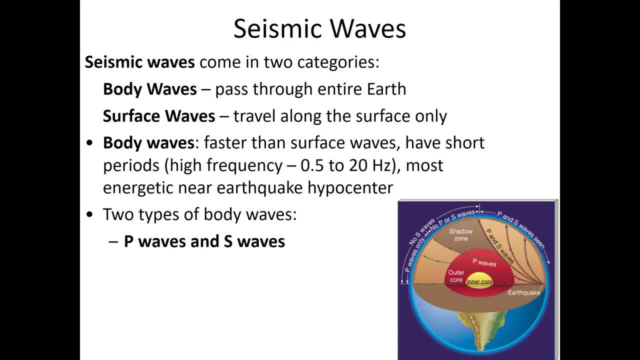 We'll discuss period and frequency later- And they are the most energetic- or you can think of most powerful, if you want to think of it that way- near the hypocenter. And there are two types of body waves: P waves and S waves. 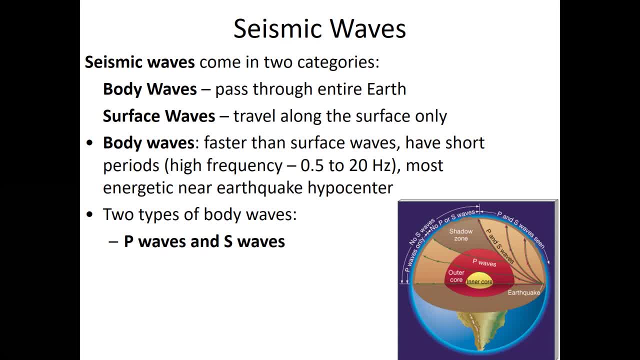 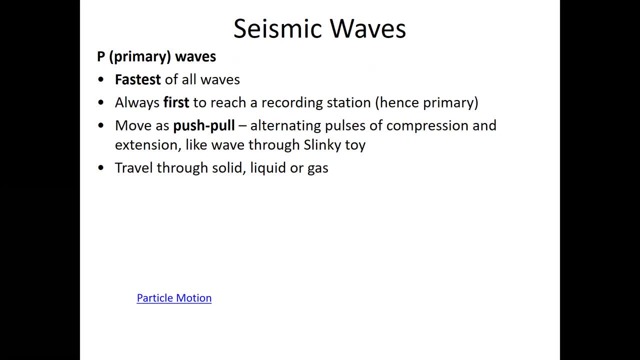 And remember, body waves are those that travel through the body of the planet or the interior of the planet. So the first type of body wave is a P wave. You can think of P for primary. Now it's the fastest of all waves. 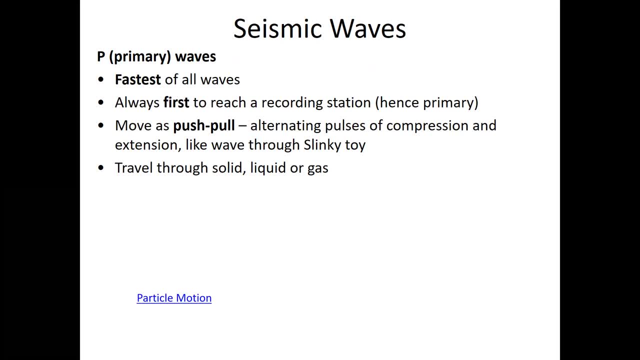 And after an earthquake it is always the first wave to reach any location, hence primary, And they move as a push-pull wave through the rock. It's alternating pulses of compression and extension, like the waves moving through a slinky And because a P wave. 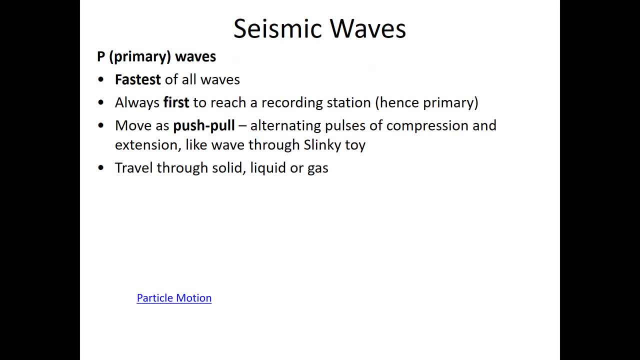 is alternating regions of compressed and extended material. they can travel through any material that can be compressed or expanded, which is all three states of matter: solid, liquid or gas. So P waves are very similar to acoustic sound waves. Actually, if there is a large 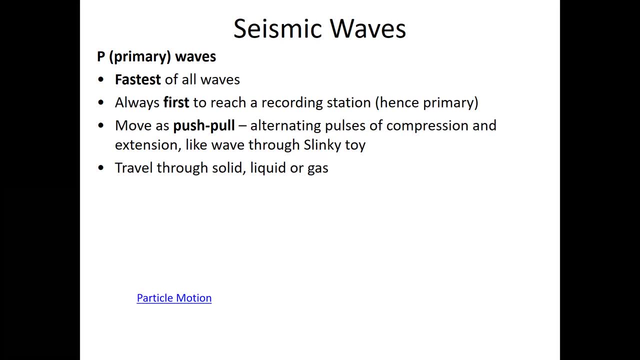 thunderclap, that thunderclap, that sound can actually convert into a P wave. once it hits the ground and begins to travel through, the ground turns into a P wave. So just as sound can travel through solid liquid or gas. 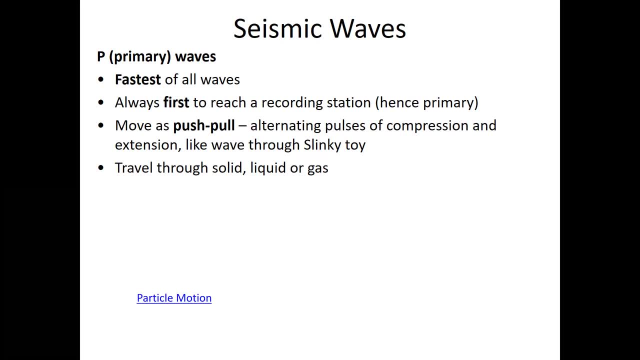 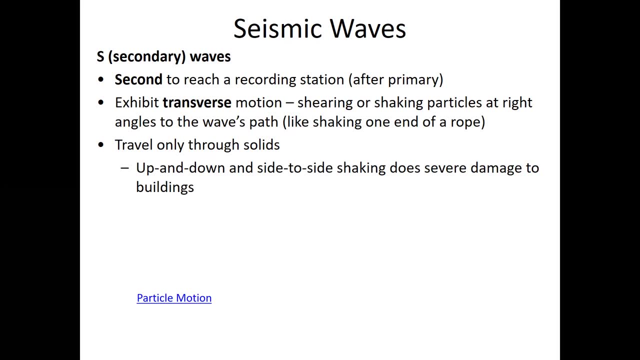 so can P waves. Where the other type of body waves- S waves- think secondary, they are the second wave to reach any location after an earthquake. Unlike P waves, these waves exhibit transverse motion, which is a shearing or shaking of particles at right angles. 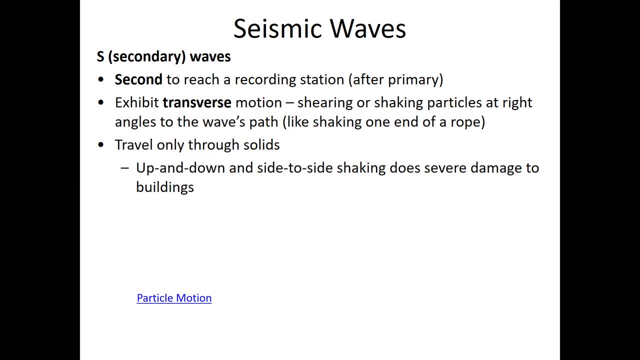 to the wave's direction. So think of a rope. So if you have a rope affixed to one end and you shake one end up and down, what happens is a wave like this travels through the rope. So you can see that the particles 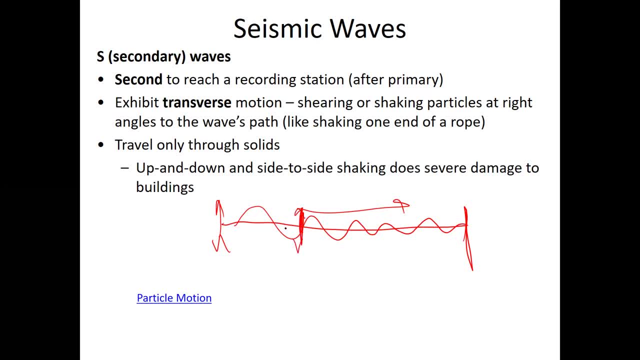 move up and down this way, perpendicular to the direction that the wave is traveling. Now S waves, because they're transverse or shear waves. they can only travel through materials that want to hold a shape, therefore can be sheared. 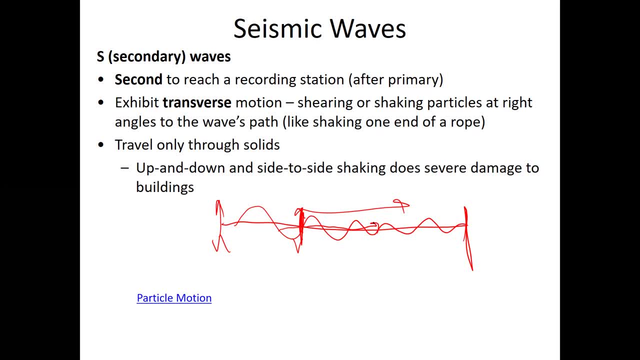 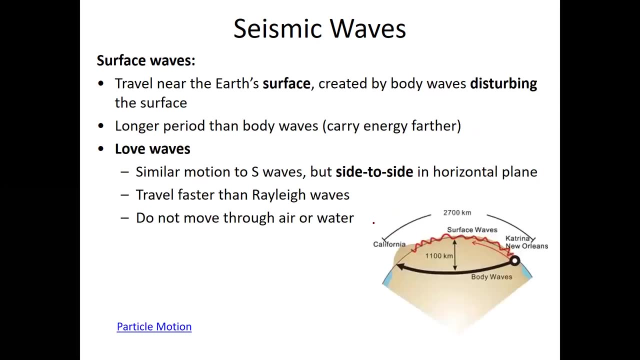 So they can only travel through solids. S waves cannot travel through liquids or gases. So those are the two types of body waves. Then we have surface waves. So surface waves, they travel near Earth's surface and they're created by body waves. 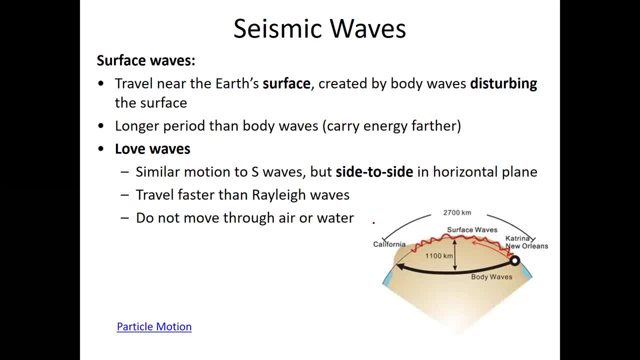 interfering with each other along the surface. It's a type of interference called constructive interference and they create these waves that travel along the surface. So you can think of surface waves as nothing but a bunch of body waves traveling near the surface that are adding together. 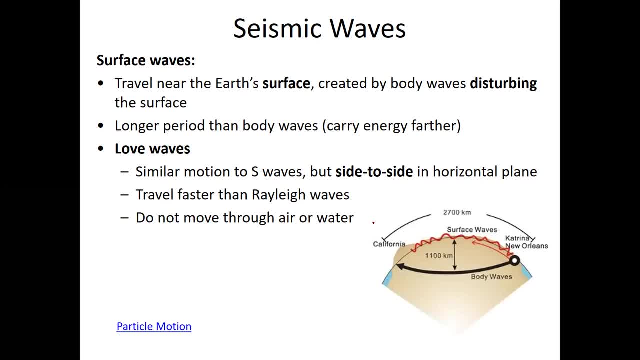 to form these new types of waves. So there's two types of surface waves. The first of the two are called love waves. It's an interesting name for a seismic wave, named after the person that first mathematically showed how they exist in the Earth. 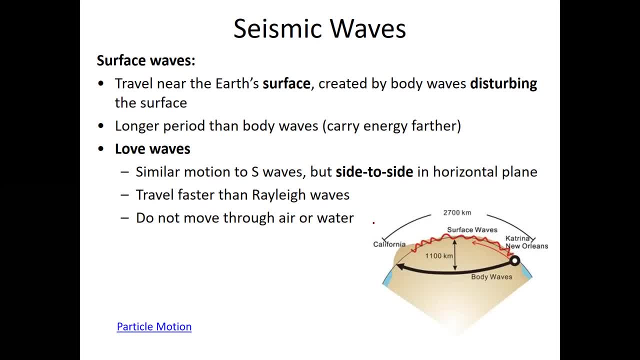 So similar to the motion of the S wave, but they're side to side. So the motion side to side motion in the horizontal plane. So if this was the surface here and a love wave was traveling in this direction, the Earth would shake. 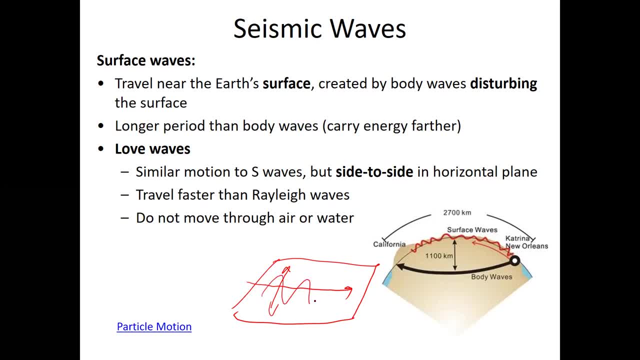 back and forth in that direction, So it would oscillate like that. And so love waves. they travel faster than radio waves, which are the other type of surface waves we're going to discuss, And because love waves are a combination of S waves, 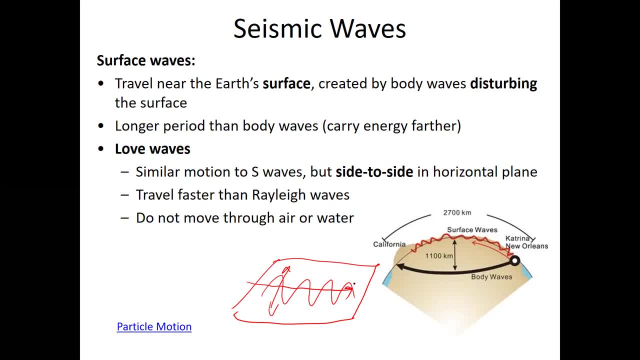 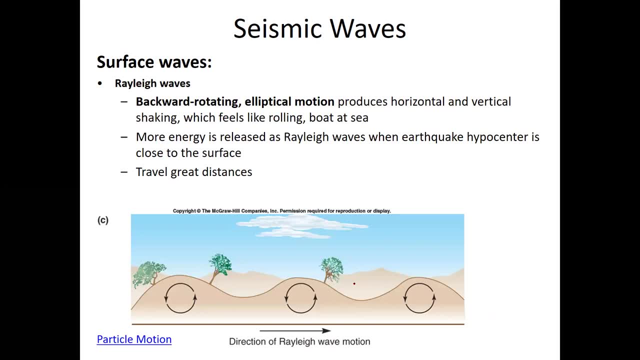 interacting with each other near the surface. they cannot travel through fluids, liquids or gases such as air or water. So, as alluded to, the second type of surface wave is a Rayleigh wave. A Rayleigh wave is is a, so, if this is the direction, 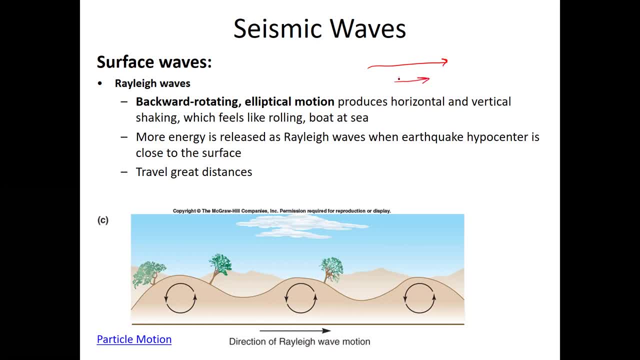 the wave is traveling, we have a P wave which has back and forth motion, combined with a vertically polarized S wave, So up and down motion, And so together that back and forth and up and down creates an elliptical motion. 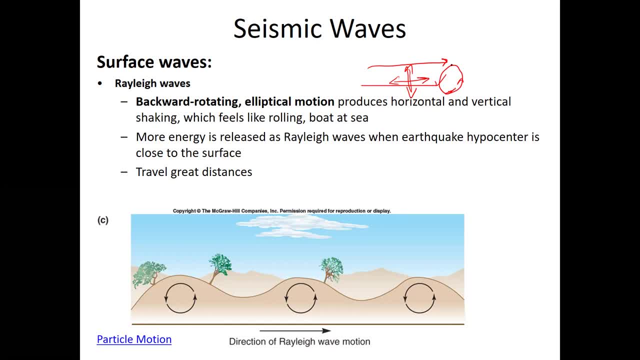 So the particle motion or ground motion of a Rayleigh wave is elliptical motion similar to kind of waves on the surface of the ocean, And so as a Rayleigh wave moves past it kind of feels like you're in a boat that's rolling with the waves. 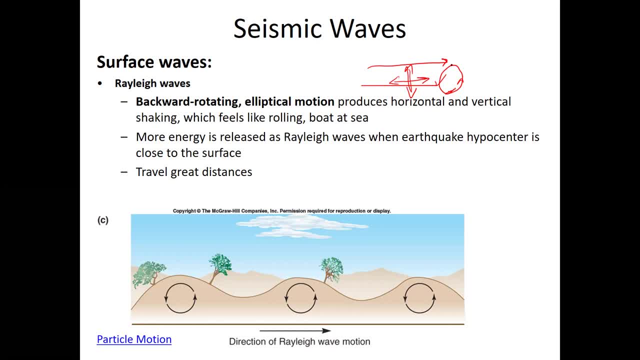 So more energy is released as Rayleigh waves when the earthquake hypocenter is close to the surface. So the Rayleigh waves are stronger the closer they hypocenters to the surface and they can travel great distances, as love waves can. So we mentioned the terms. 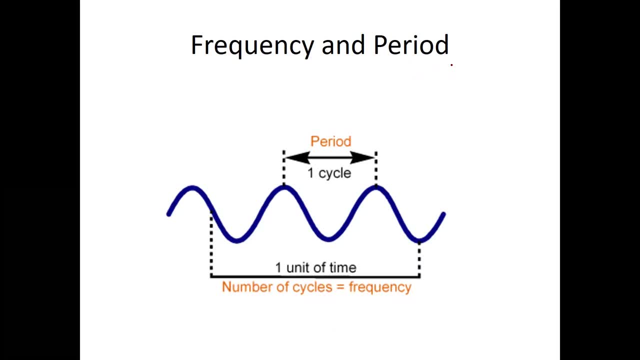 frequency and period before, And I'm sure you've heard of at least frequency and definitely the word period, but maybe in a different context. But they are related to each other And frequency and period are are used to quantify basically how many waves. 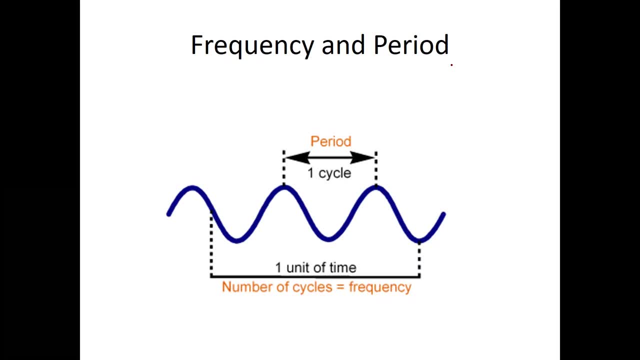 the speed? oh, it's not really the speed, They it's. well, let me just define each of them independently. The frequency of a wave is how many waves pass by a particular point per second. Okay, So if five waves pass by, 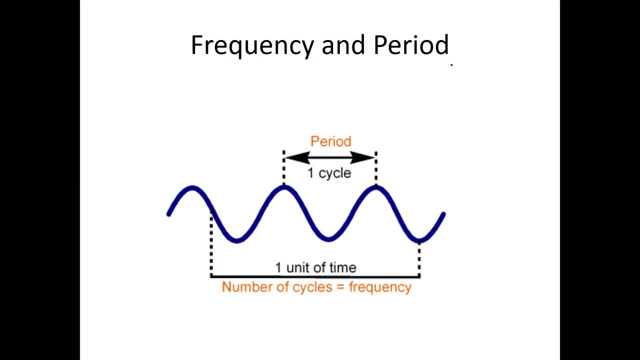 a particular point in one second. that wave is said to have a frequency of five Hertz. Hertz, HZ are the units of frequency And Hertz is one over seconds. That's what a Hertz is, one over seconds, So it's number of waves. 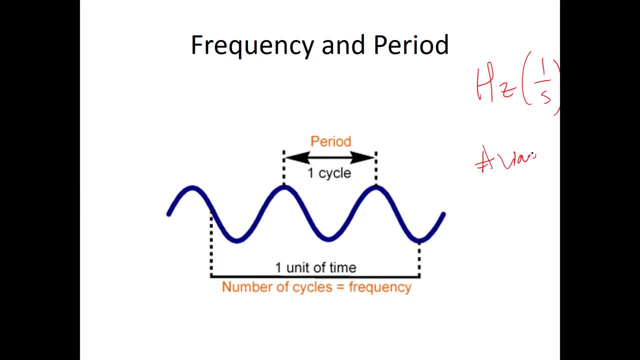 per second, And so it's one over seconds and that's Hertz, Right. So if something occurs at a frequency of one Hertz, that means it's occurring once every second. If something occurs with a frequency of one half Hertz or 0.5 Hertz, 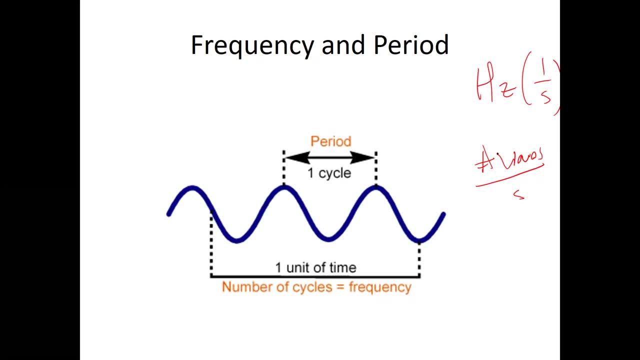 that means it's happening half a time every second And therefore it it makes happens once every two seconds. Something has a frequency of 10 Hertz. it's 10 times per second. Right, Where a period is the amount of time it takes. 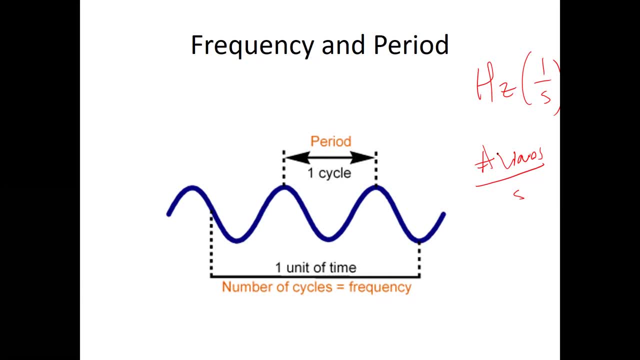 for one wave to pass by. So if it takes a wave 10 seconds to pass by, that is a wave with a period of 10 seconds. So when we say a whole wave, we're talking about one full cycle. So a cycle is. 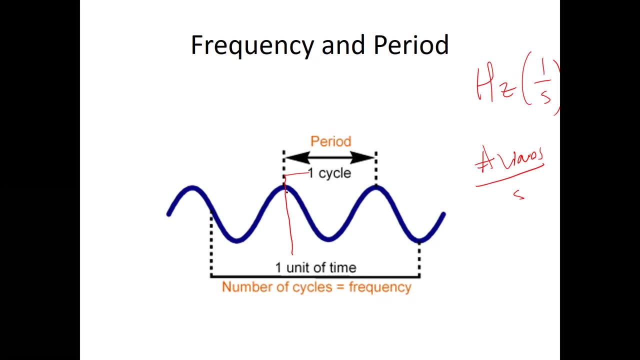 is one full wave, And so we can break a wave into parts. So we have the tops, which are known as crests, and the bottom, which are known as troughs, And so from crest to crest, that's one whole wave cycle. 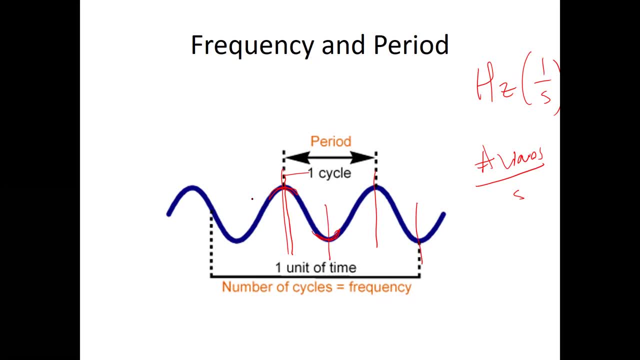 trough to trough, that's one whole wave cycle. Or we can go now going from trough to crest to going from trough to crest- that's one full wave cycle. See, these are all the same same length, right, That's one full wave cycle. 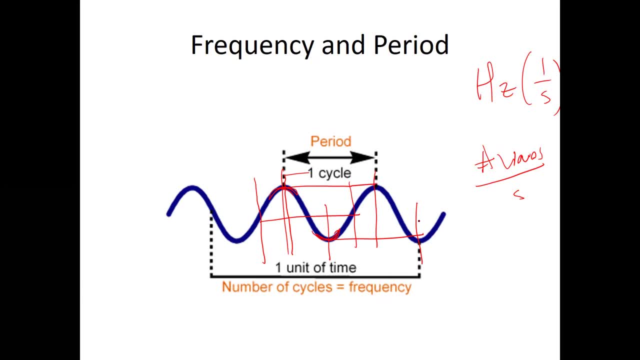 Now the time it takes for one full wave cycle to pass by a fixed point, that is the period, And the number of wave cycles that pass by a particular point in one second is the frequency. So let's say, if a wave has a period, 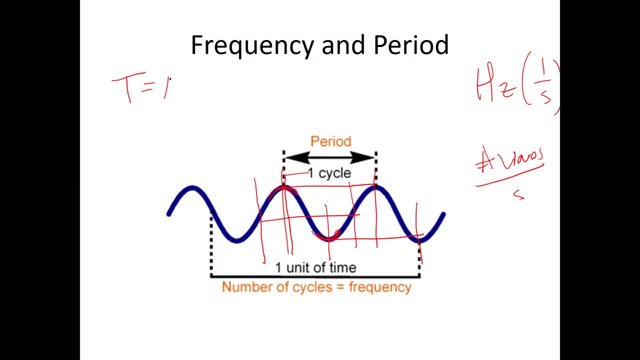 which we use a capital letter, T, to represent a period of 10 seconds. So it takes 10 seconds for one wave to pass by. That's what is the frequency of that. Well, how many waves are passing by in one second? Well, if it takes 10 whole seconds, 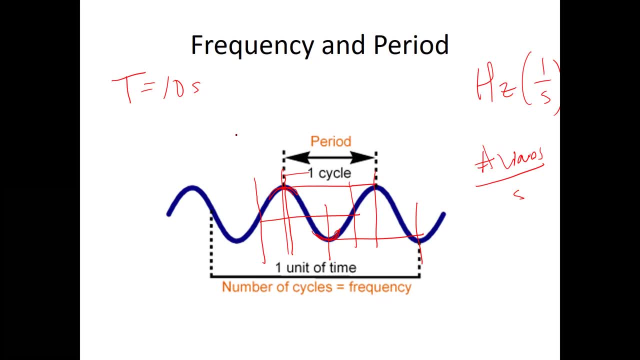 for one wave to pass by after one second. only one tenth of a wave has passed by, So the frequency would be one over 10 hertz. Right where, if the period was two seconds, what would be the frequency? Well, it takes two seconds to pass by. 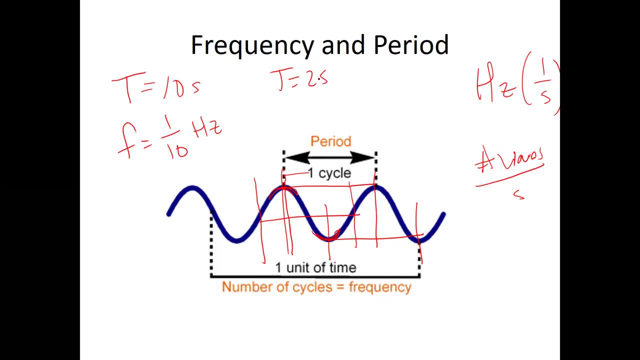 a particular point. a particular point then: how many waves have passed by in one second? Well, only half of a wave. The frequency would be one over two hertz. So if you could see the relationship here, the frequency of a wave is equal to one over its period. 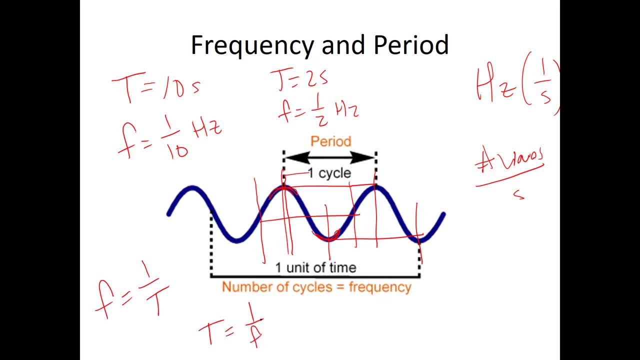 And, conversely, the period of a wave is equal to one over its frequency. So, therefore, if we have a wave that has a frequency of 10 hertz, what is its period? Its period is one over 10 seconds, So it only takes one tenth of a second. 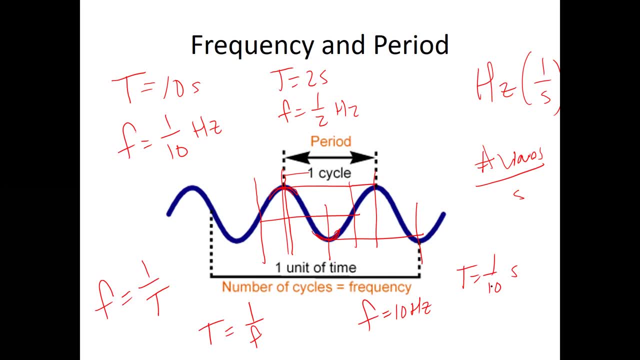 for a wave to pass by Because, well, its frequency is 10 hertz. That means 10 waves are passing by every second. So it only takes one tenth of a second for one wave to pass by. That's frequency and period. 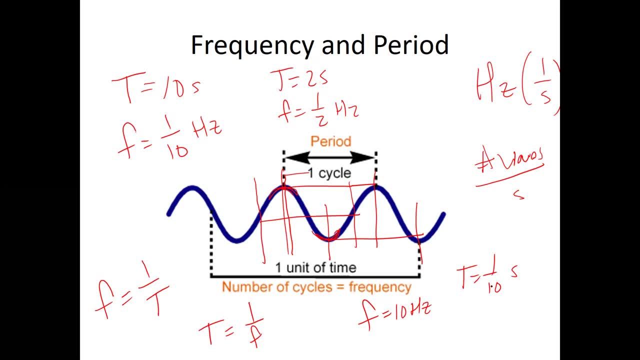 And so, as the higher the frequency is, the shorter the period, right, There's more waves passing by every second, So the amount of time it takes for one wave to pass by decreases. The smaller the frequency, the larger the period. 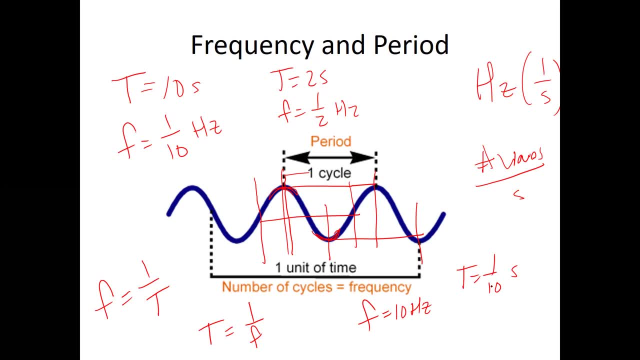 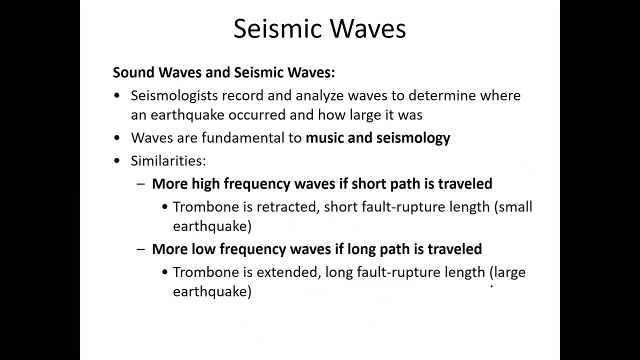 The fewer waves are passing by every second. that means it takes a longer amount of time for one wave to pass by. So these attributes of frequency and period, they're applicable to any type of wave, not just seismic waves, sound waves, electromagnetic waves. 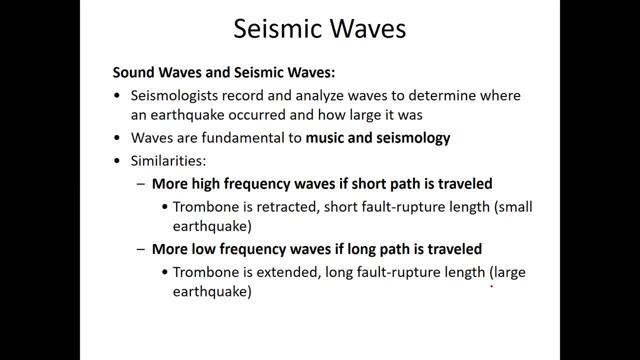 all types of waves And seismologists. they record and analyze these seismic waves to determine where an earthquake occurred and how large it was. So waves are fundamental to music and seismology. There's a lot of similarities between sound waves and seismic waves. 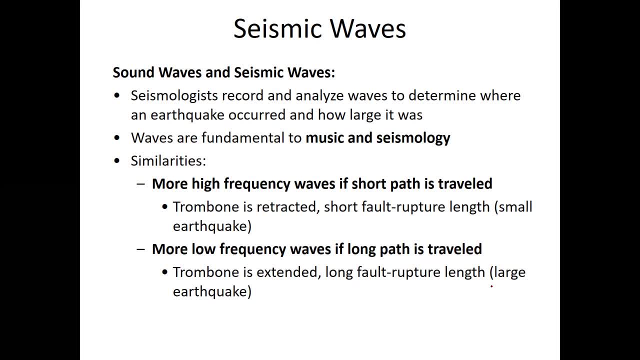 Similarities are the more high frequency wave if it's a short path travel. What does that mean? Well, imagine a trombone. As you play a trombone and you pull the slide out, what you're doing is you're increasing the length of the tube. 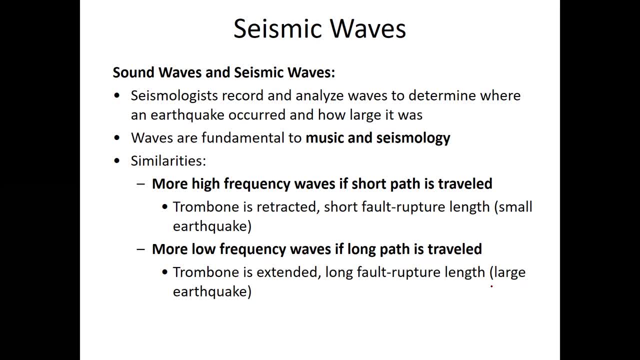 in which the sound can resonate, And so you're creating a longer resonance chamber which creates a longer period or lower frequency sound. So if you pull the slide out, it's lower frequency, longer period, where, if you pull the slide in, 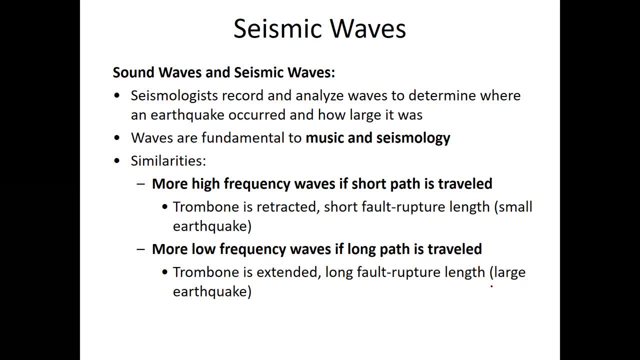 you're decreasing the chamber in which the length of chamber in which air can resonate, generate sound, And so that shorter resonance chamber creates waves that have higher frequency or smaller periods. Just like the string guitar: if you play a string open, the string of the entire length vibrates. 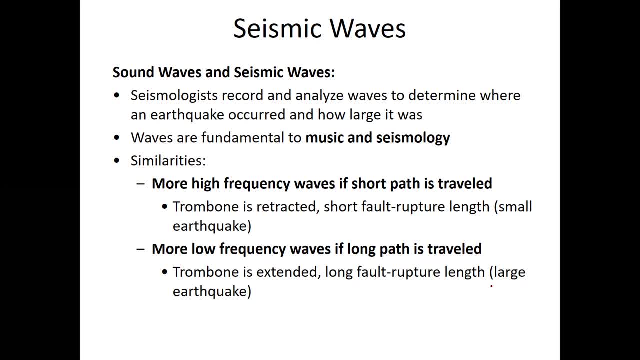 and it creates a sound of a particular frequency or period. But if you put your finger down on the fretboard, what you do is you effectively shorten the length of the string that's allowed to vibrate, And that shortened length causes it to vibrate faster. 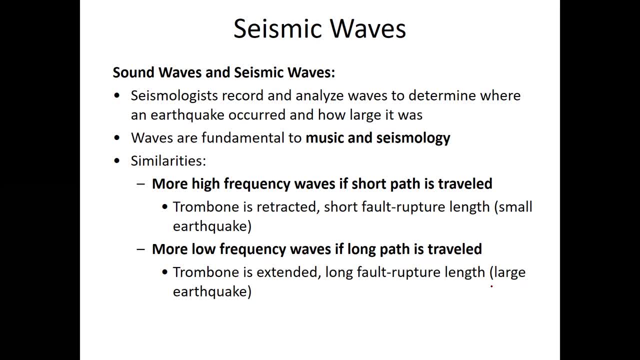 therefore generate a higher frequency, lower period sound. The same thing is true with seismic waves. So if there is a large segment of the fault that ruptures, it's very long, it'll generate very low frequency, large period waves. But if it's a very short segment, 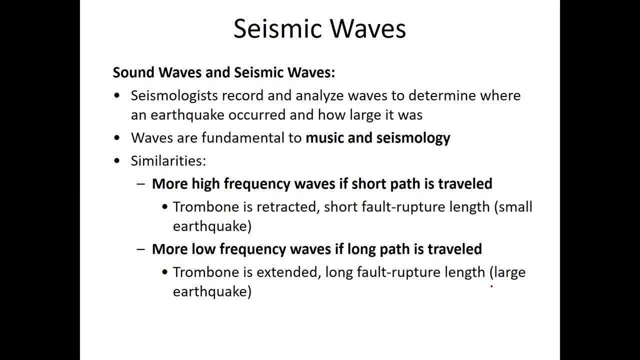 of the fault that ruptures, it'll generate very high frequency, So small period seismic waves. Now, often times in an earthquake, you'll have short segments rupture here, here, here and there, and long segments rupture in different parts. 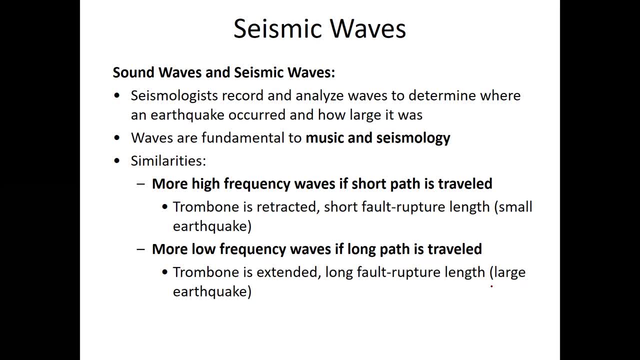 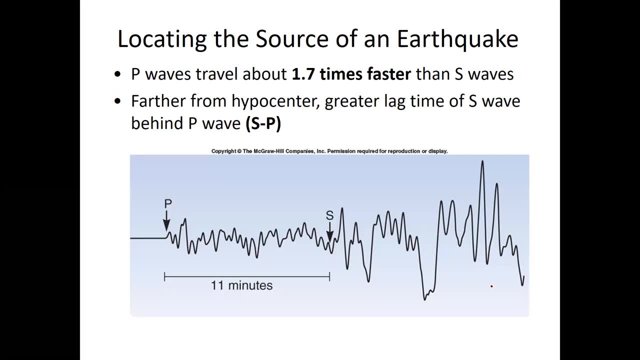 so you'll have combination being generated, But it's the same concept, And so how do we locate the source of an earthquake using seismic waves? Well, we know, between the two body waves, that P waves travel faster than S waves, On average. 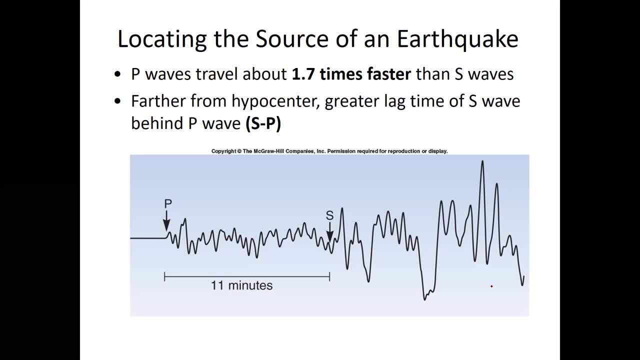 P waves travel about 1.7 times faster than S waves, And so, since they both begin from the earthquake, these P and S waves and travel away from the earthquake. the further you are from the earthquake, the more distance the P wave gains on the S wave. 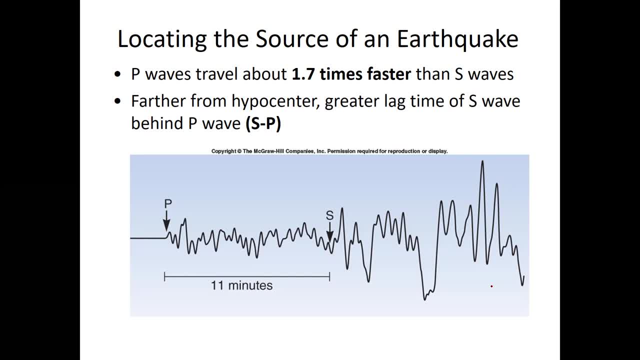 And therefore, if you're recording these seismic waves, the further you are from the earthquake, the longer the period of time between the P and the S wave arrival would occur, the further you are from the earthquake. This is called lag time, So one way of thinking about this is: 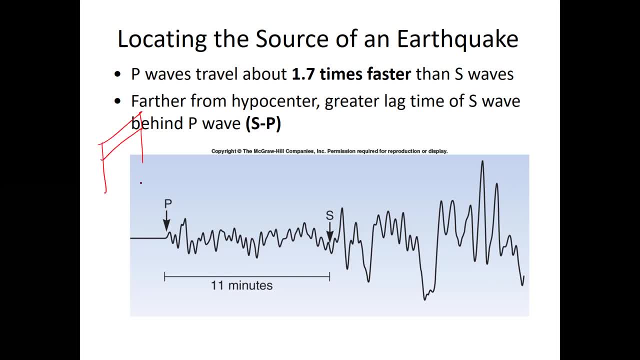 let's say you have a race right, Here's the starting line. You have two runners, runner P and runner S. You can guess which one's faster? right, The race starts. Both runners start from the same location. That is the earthquake. 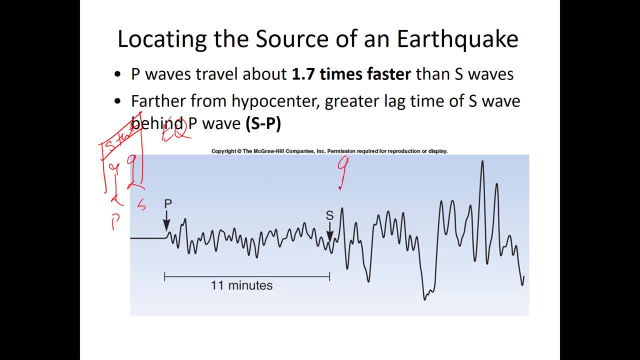 As they run the race, the runner P, which is faster, gets increasingly further and further ahead of runner S. So if we were to record the time at which they arrive, say, at this location, A runner P would arrive, and then, after some amount of time, 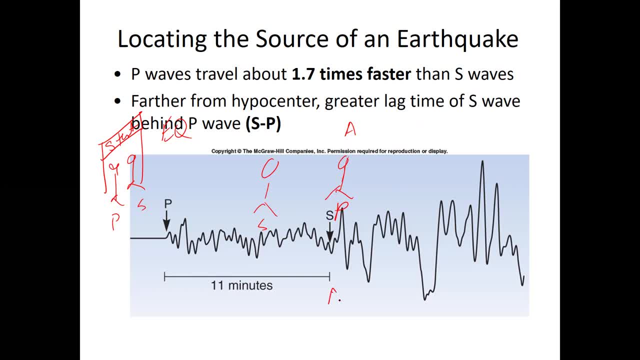 runner S would arrive, And let's call that delta T A, where delta T is the arrival time of the S wave, which is going to be larger. It takes more time for the S wave to get there, minus the arrival time of the P wave. 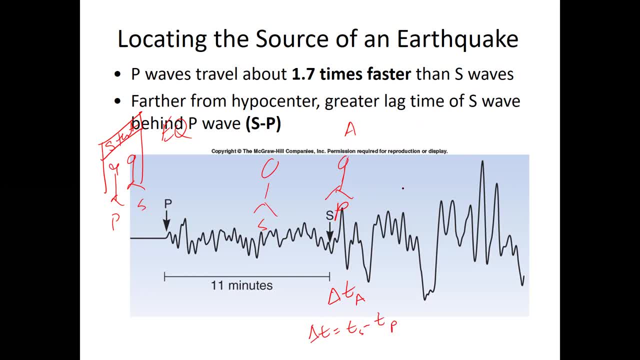 which is shorter because it gets there sooner Then location B. if we were to record the arrival times, the difference in time between the arrivals would be larger, because P would get here faster and then S would get here more slowly And because, by virtue of being further away, 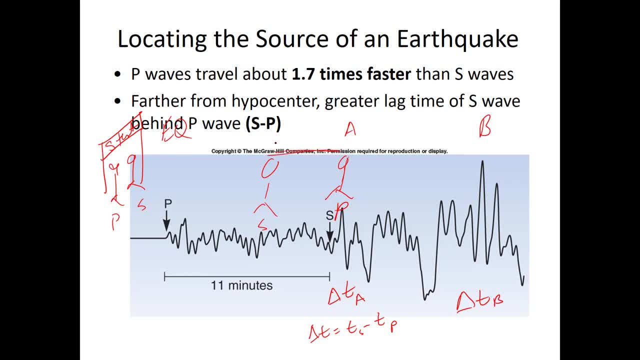 from the starting point. the delay time between the P and S wave, or runner's arrival at this location, would be larger, And so this delay time between the P and the S wave, it is a function of distance. Okay, So if we plot this against distance, 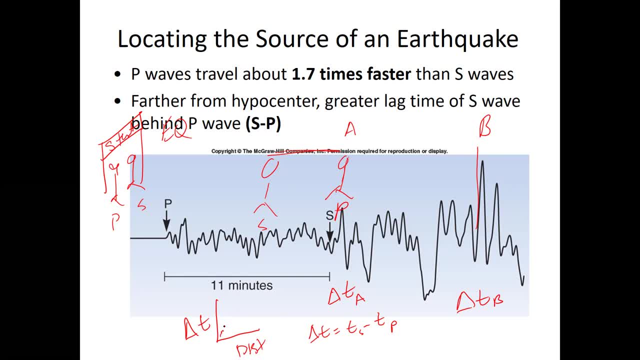 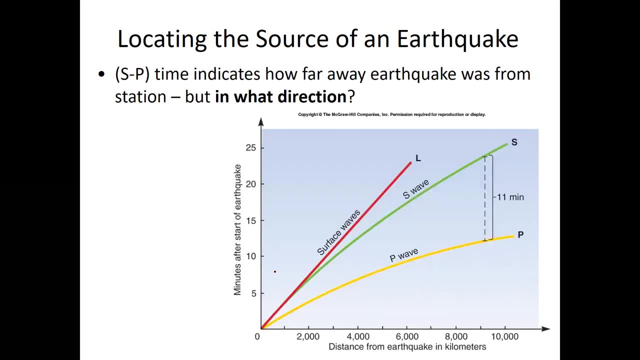 it would. it's not, it's not exactly a line. It goes something like that: Okay, So here we see, here is the minutes after the start of the earthquake. So this is time And this is distance from the earthquake. 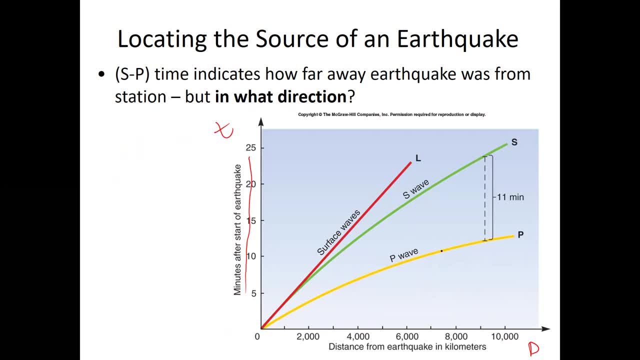 And the yellow line is the arrival time: how long it takes for the P wave to arrive at different distances away from the earthquake, While the green line is the arrival time of the S wave. how long it takes for the S wave to arrive at a particular distance. 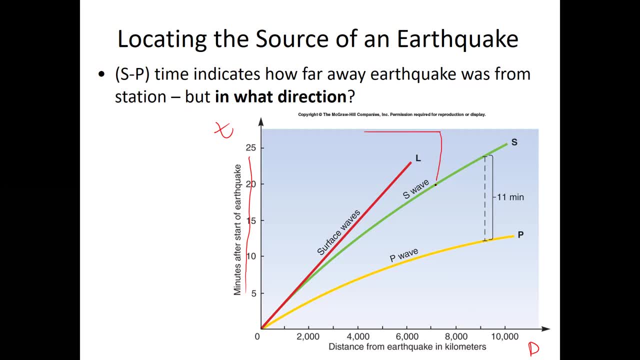 away from earthquake. So if you look at the P and the S arrivals at a particular distance, this is the delay time. So the P wave will arrive after 10 minutes at, say, 7,000 kilometers from the earthquake, But the S wave won't arrive. 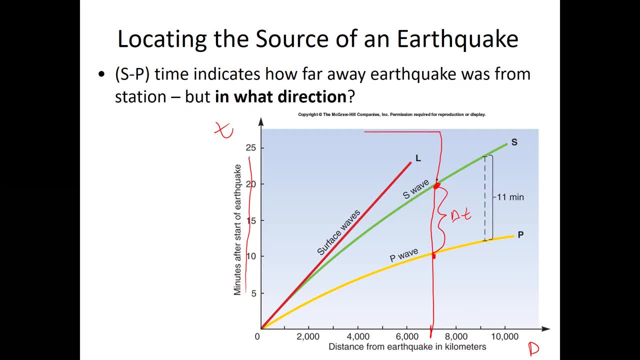 until close to 20 minutes. It'll take a 10 minute, take 10 additional minutes for the S wave to arrive, And the closer you are to the earthquake, the shorter that delay will be. And it gets shorter and shorter the closer to the earthquake. 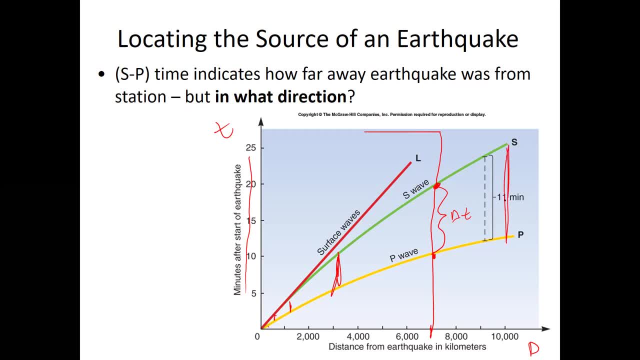 And the further you are from earthquake, the longer that delay gets. So if we can measure that delay time, that delta T, we can find how far away we are from the earthquake. That's only some of the information. Alright, let's say 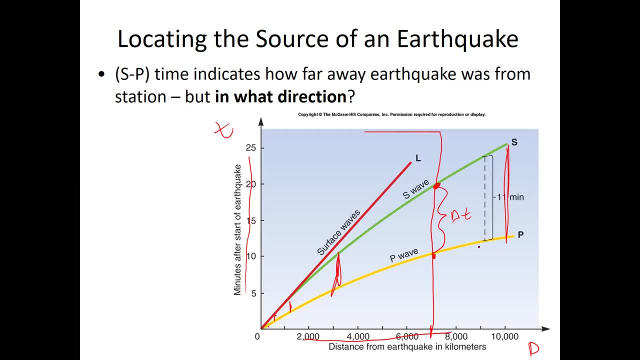 that, oh, you know, we recorded these seismic waves and we found that the S wave arrived 11 minutes after the P wave. Well, that corresponds to roughly 9,000 kilometers. The earthquake occurred 9,000 kilometers away from this location. 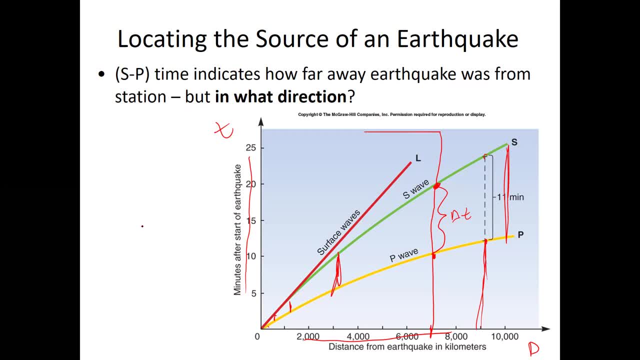 in which we recorded these seismic waves. So let's say, you know, this is where we recorded the seismic waves. Well now, the earthquake could have occurred anywhere along this circle, whose radius is 9,000 kilometers. So we have an idea. 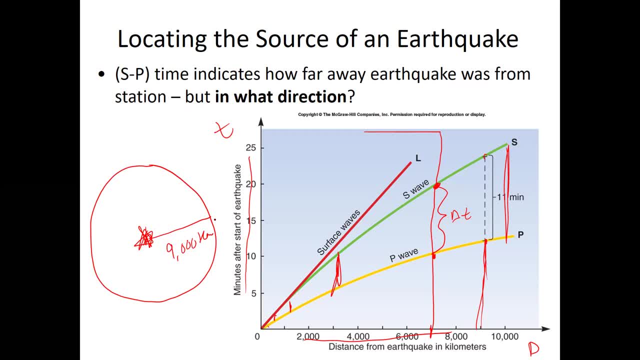 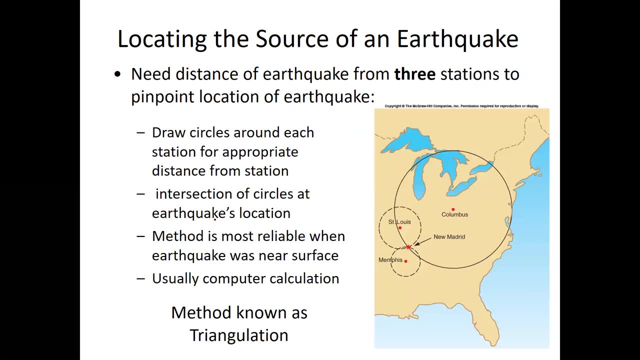 of where the earthquake could have occurred, anywhere along the circle, but we don't know exactly where. We need more information, And so what information do we need? Well, we need the same information from two more seismograms, So we record the seismic waves. 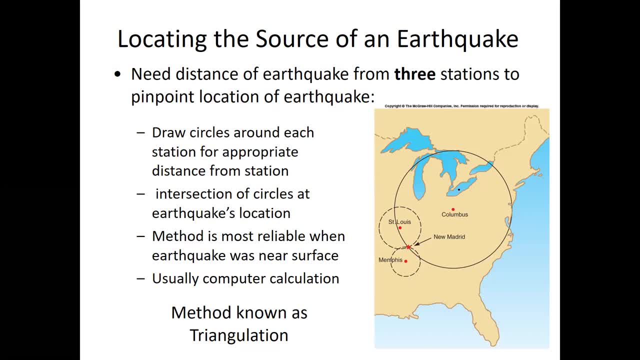 after an earthquake at three different locations. We measure the delay time between the P wave and the S wave. That gives us a corresponding distance. We plot a circle on the map with the appropriate radius And we do that for two other locations And we'll get three circles. 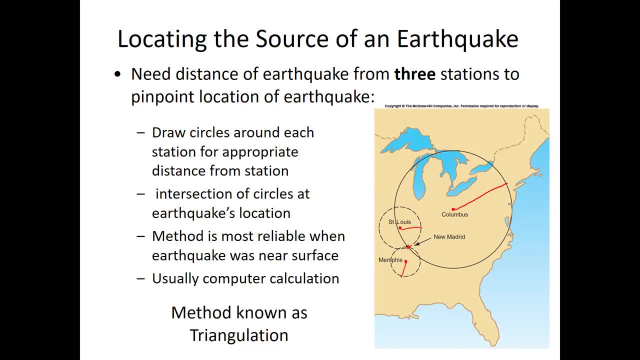 And those three circles will overlap at exactly one point, And that one point is the appropriate distance From all three locations and is therefore the location of the earthquake. If we just had two circles, we would have two potential locations. We don't have a unique solution. 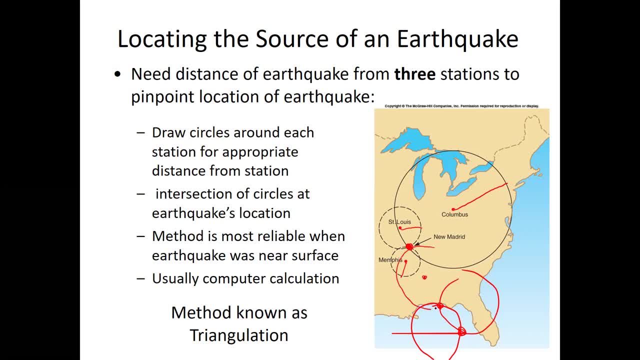 So you need three seismograms and three recordings to figure out where the earthquake occurred, And this gives us the epicenter as well. And this method is called triangulation. It's not something unique to seismology. This is how your phone's location. 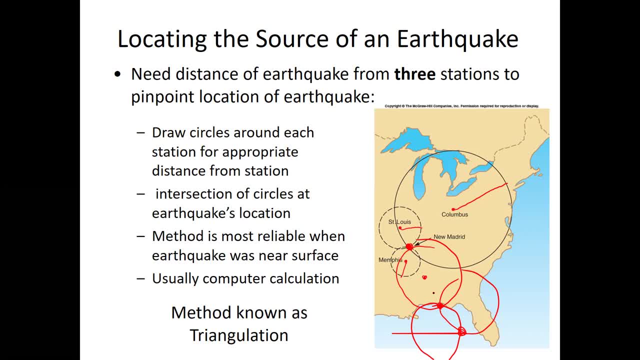 is determined without using GPS. It communicates with three different cell phone towers, And so the cell phone tower sends out a ping in the form of a radio wave in all directions. Your phone picks up that ping and sends a ping back to the cell phone tower. 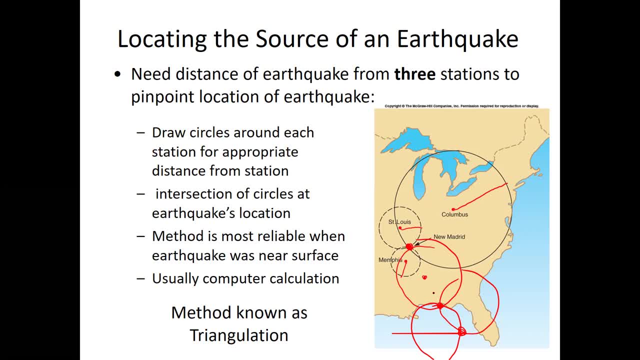 And what the cell phone tower does is: it pays attention to the amount of time it took between the transmission of that ping and the reception of the response, And, using the speed of light, and the amount of time between the departure and arrival of those pings. 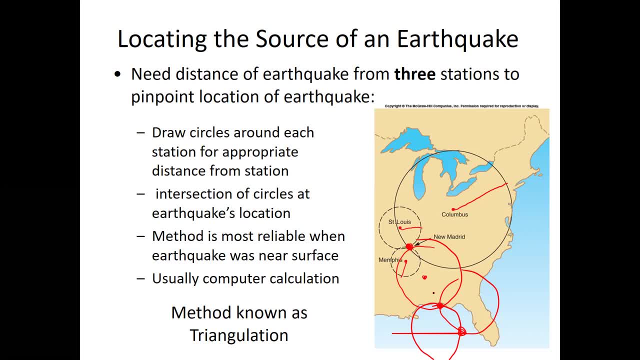 it can be calculated how far away your phone is from that tower, And so then you draw a circle around that tower of the appropriate distance, And you do the same thing for two more cell phone towers, And those three circles will overlap at one location. 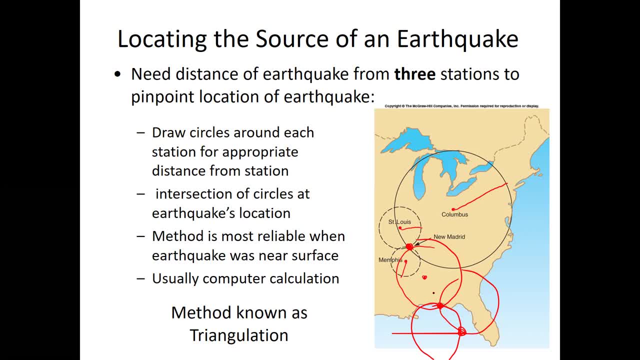 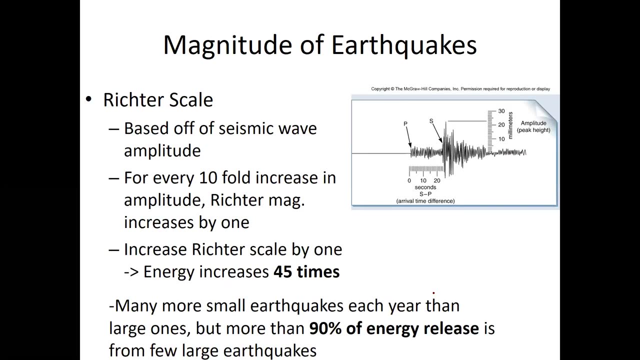 and that's the location of your cell phone. Now, GPS does the same thing, except you're communicating with satellites in space and not cell phone towers. But you still need at least three satellites in order to triangulate your location. And, by the way, 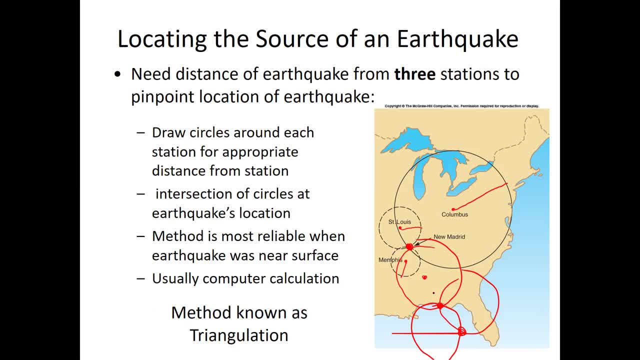 this process is all automated. So once an earthquake occurs, computers have been programmed to recognize p and s wave arrivals, They measure the delay time and they do this for a bunch of different locations or recording seismic waves, And they triangulate the location of an earthquake very quickly. 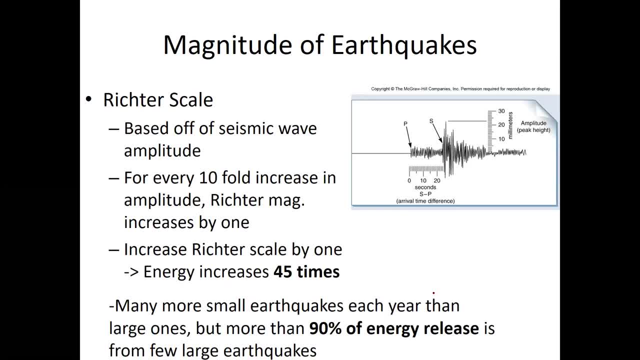 That's how we know where these earthquakes occurred so quickly after they actually happened. So next, looking at the magnitude of an earthquake, the seismic earthquake, we used to use what's called the Richter scale, And the Richter scale is based off. 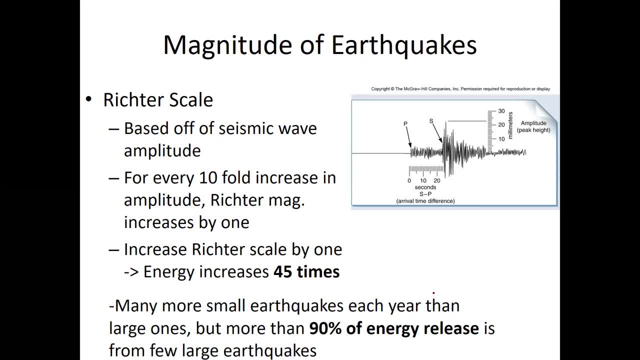 of the amplitude or the size of the seismic wave produced And according to the Richter scale, for every tenfold increase in amplitude or tenfold increase in the amount of shaking, the Richter magnitude would increase by one. And if we look at 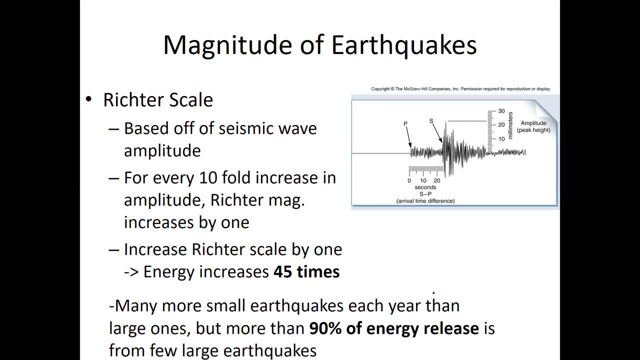 more simplified numbers. let's say we had shaking. that was one unit of shaking, So the ground moved up and down. one unit, one unit of distance. Let's say that's a magnitude one on the Richter scale. Well, magnitude two- earthquake on the Richter scale. 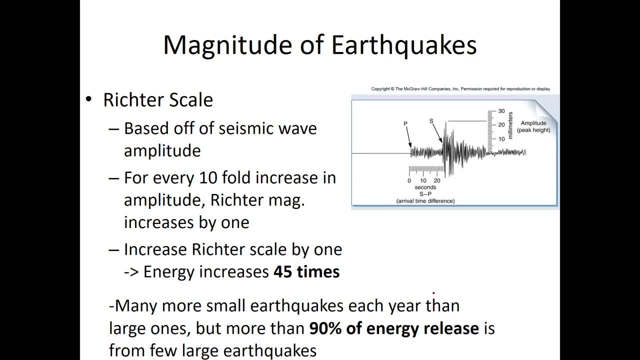 would be one in which the shaking moved the ground up and down ten units, And magnitude three on the Richter scale would be one where the ground moved up and down 100 units. So each increase of one on the Richter scale corresponds to a tenfold increase. 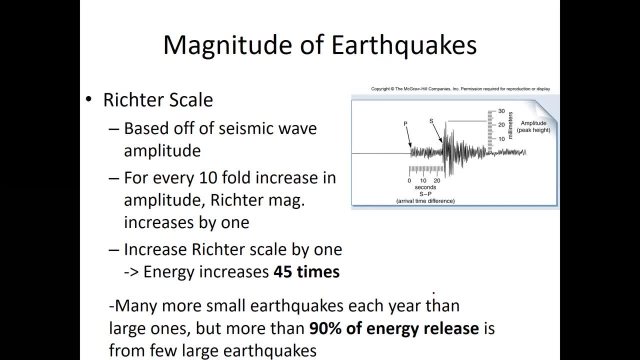 in the amount of shaking. As far as energy released by the earthquake, each increase on the Richter scale corresponds to roughly a 45-fold increase. So a magnitude three earthquake releases as much energy as roughly 45 magnitude twos And a magnitude four earthquake. 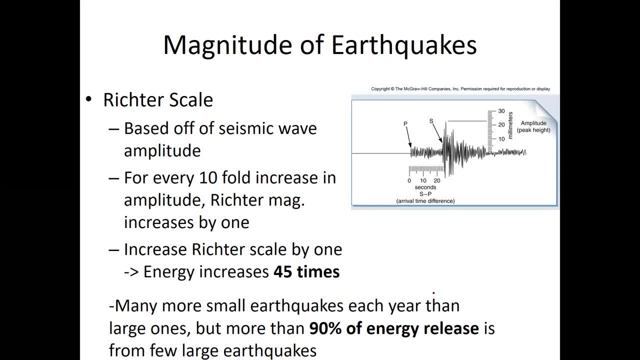 releases as much energy as roughly 45 magnitude three earthquakes or 45 squared magnitude two earthquakes. So there's many more smaller earthquakes each year than large ones, but more than 90% of all energy released by earthquakes is from the few large earthquakes each year. 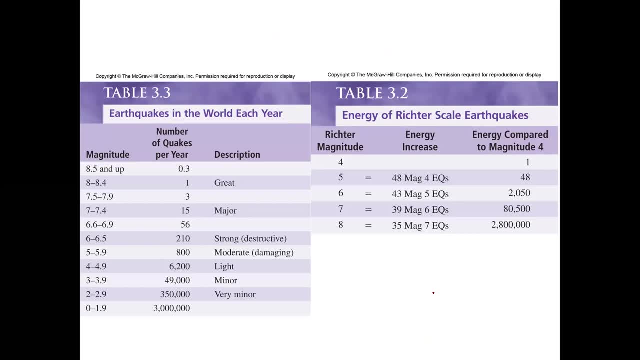 So there's a small number of earthquakes each year. These tables show us the frequency of earthquakes of different size, And so we have going from largest at the top- this is the table on the left- to smallest on the bottom, And so we see for. 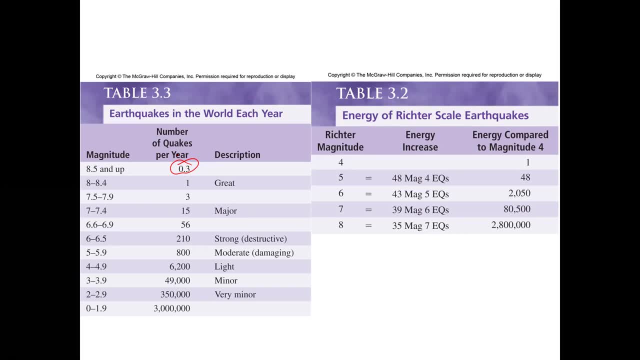 magnitude 8.5 and up, we have less than one a year- 0.3,. so what does this mean? That means that one of these earthquakes occurs roughly once every three years, because after three years, 0.3 adds up to 0.9,. 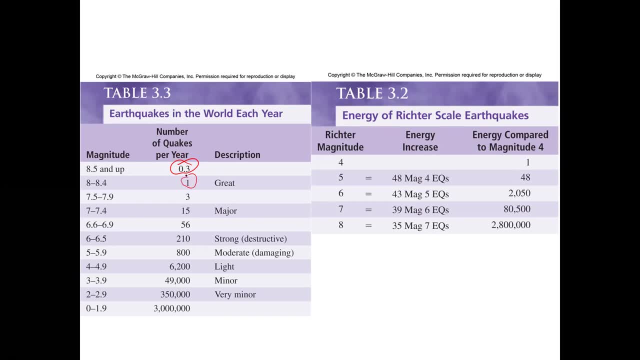 and that's close to one. We have, on average, one earthquake between the magnitudes of 8 and 8.4 each year: 3, 7.5 to 7.9,, 15, 7 to 7.4,. 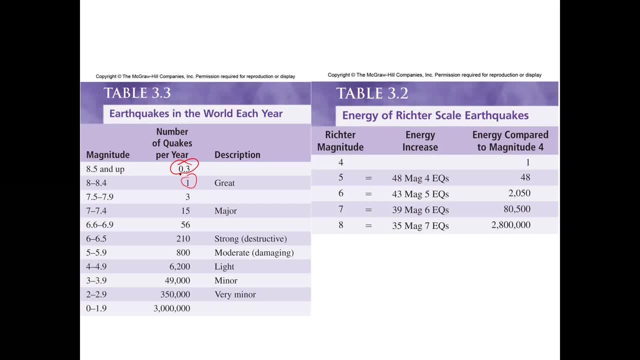 56 earthquakes between 6.6 and 6.9, and you can see the general trend, the frequency, the number of earthquakes per year increases as the magnitude decreases. So where there's three million earthquakes between 0 and 1.9.. 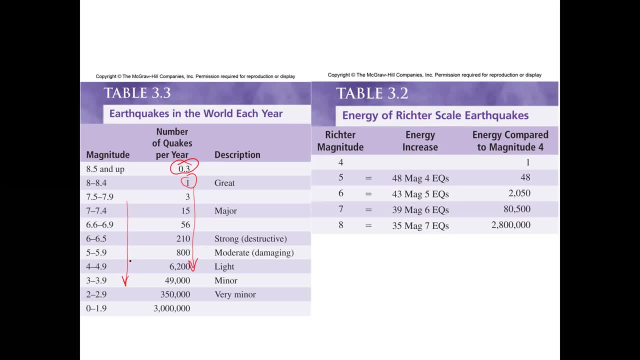 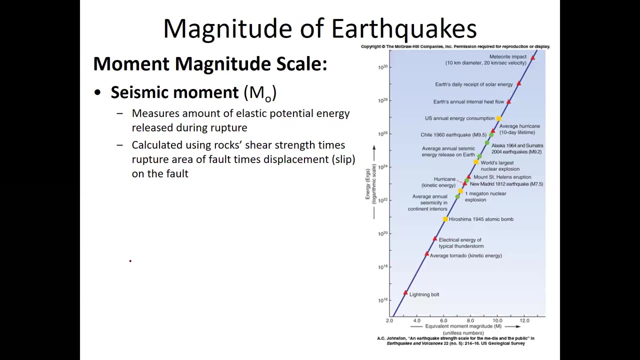 So, as we talked in our first lecture, this is that inverse relationship between magnitude and frequency. So, however, the shaking that results from an earthquake, the size of the seismic waves, is somewhat subjective and that's dependent to some extent on the material. 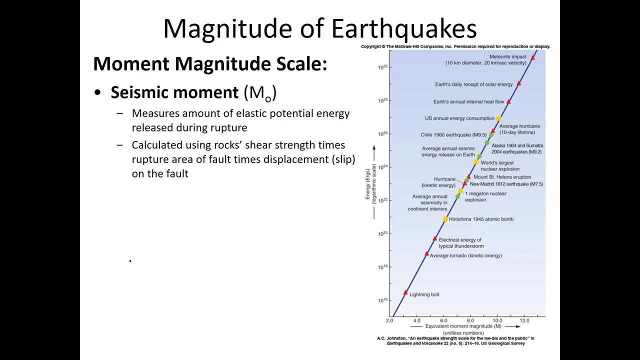 that the shaking is occurring and the seismic wave is traveling through, whether it be bedrock or loose unconsolidated material like sediment. So if you were to measure the size of the earthquake based upon the size of the seismic waves, that could be a subjective measurement. 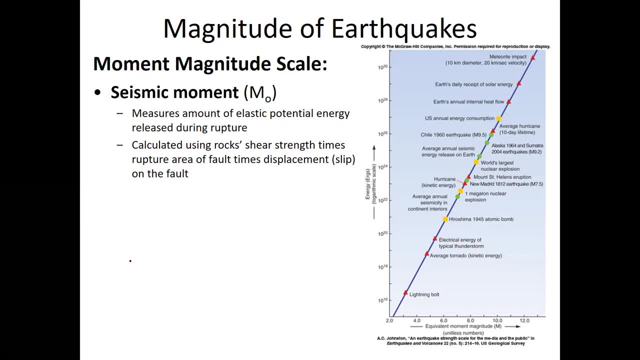 not objective, Not subjectivity. With that said, seismologists have adopted a new method of ranking or quantifying the size of an earthquake, and that's using what's called the moment magnitude scale, And so the moment magnitude scale is used by measuring the actual amount. 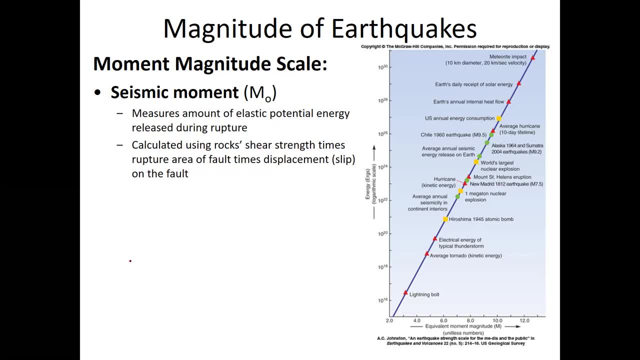 of elastic potential energy released during the rupture of your fault. That's calculated by using the rock's shear strength from the friction walls in the fault, multiplied by the rupture area of the fault and that multiplied by the slip, the distance that the fault slipped. 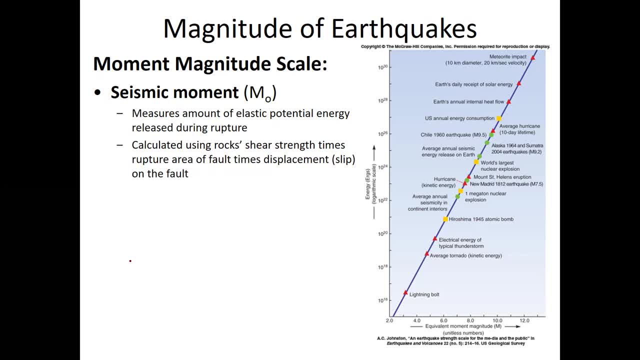 That gives us the moment magnitude. The moment magnitude scale loosely follows the Richter magnitude scale. What I mean by that is magnitude 3 earthquake, and the moment magnitude scale is roughly magnitude 3 and Richter scale, but they don't line up exactly. 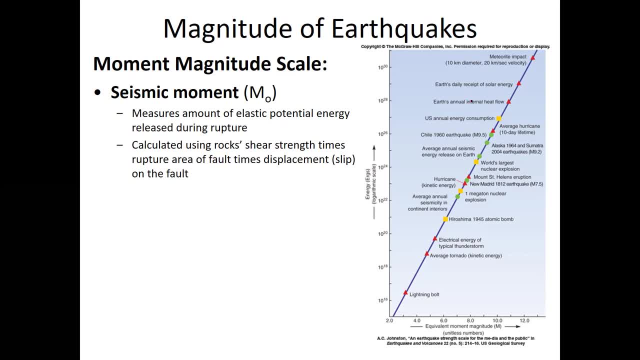 but they're close. This figure on the right shows us energy in units of ergs, which is a weird English unit of energy, and it's a logarithmic scale, so each tick is a tenfold increase. so this is 10 to the 16th. 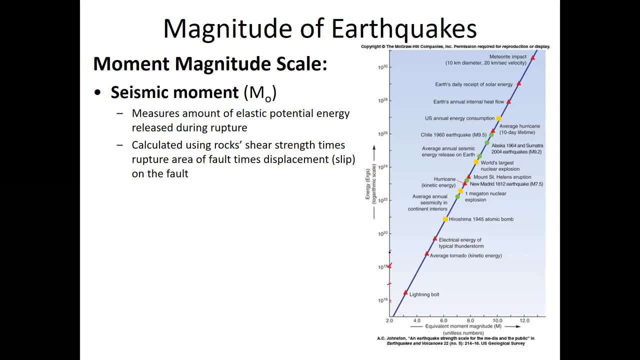 and this is 10 times that. so it's 10 times the 17th. this is 10 times that, 10 to the 18th, so each of these is a tenfold increase and this is the equivalent moment magnitude. 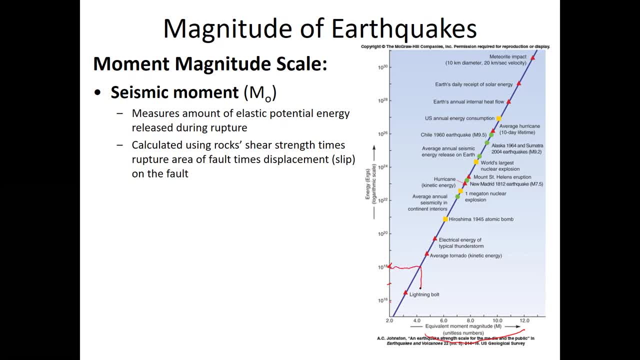 of an earthquake And magnitude 4 earthquake releases as much energy approximately releases 10 to the 18 ergs. But what's interesting is we can see earthquakes are plotted as these, these notable earthquakes are plotted as these green circles and other events are plotted. 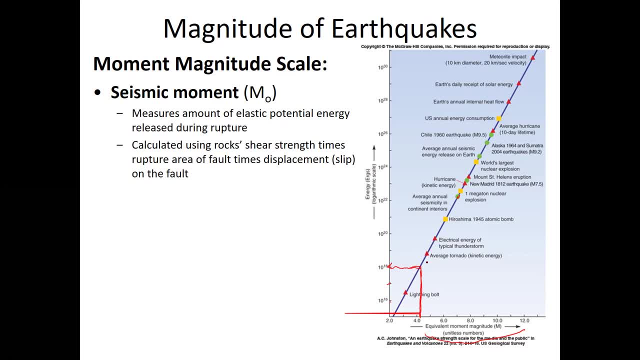 as triangles or squares. A large tornado releases as much energy as roughly a 5.0 earthquake. The Hiroshima bomb dropped in 1945 releases as much energy as approximately a magnitude 6 earthquake. A hurricane releases as much energy as a 7 and change earthquake. 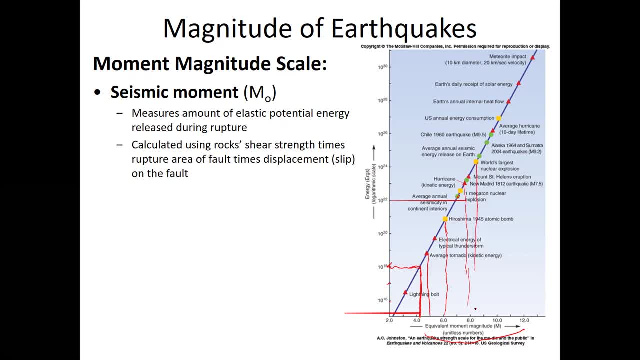 So the world's largest nuclear explosion was a little bit larger than 8.0.. Here is the largest earthquake ever recorded, a magnitude 9.5, occurred off the coast of Chile in 1960.. This is the amount of energy released by a hurricane. 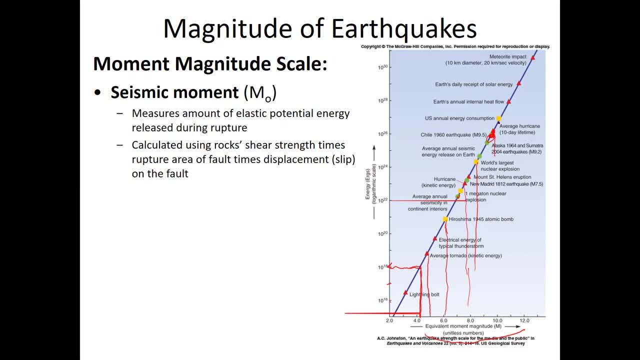 average hurricane over the course of 10 days. This is annual US energy consumption, which is about the same amount of energy that a magnitude 10 earthquake would produce. Just to note that a magnitude 10 earthquake is theoretically impossible, There is no fault long enough. 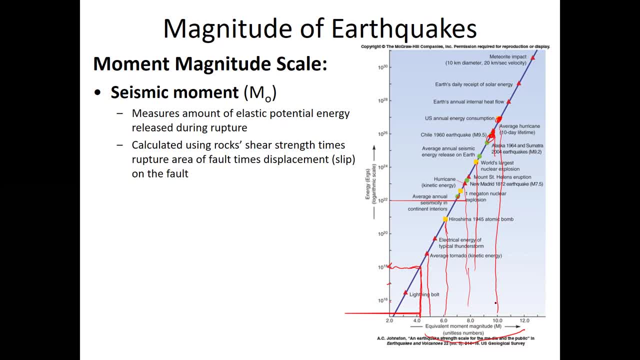 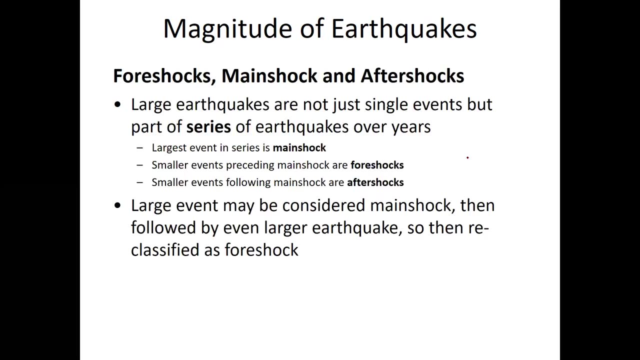 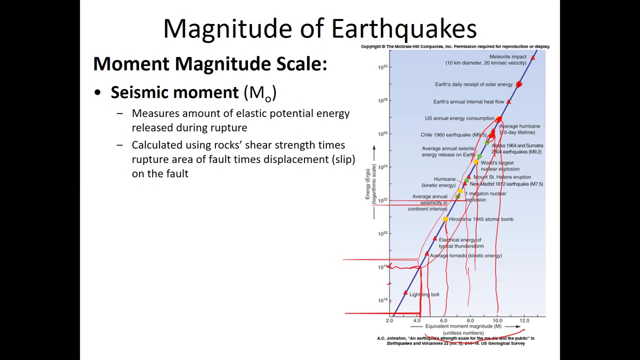 that could rupture. that would generate a magnitude 10 earthquake. So this allows us to compare earthquake magnitude and energy release to other energetic processes. You can see the Earth's daily energy is extremely large. There's so much energy we receive from the Sun. 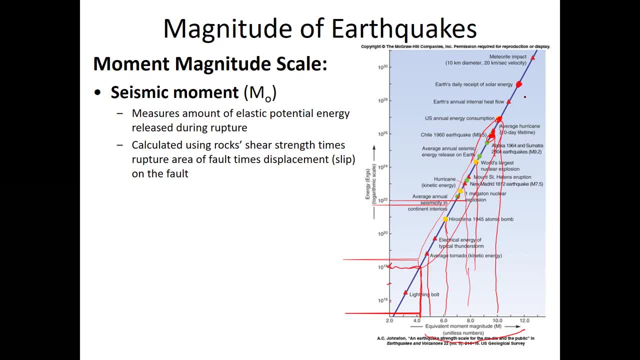 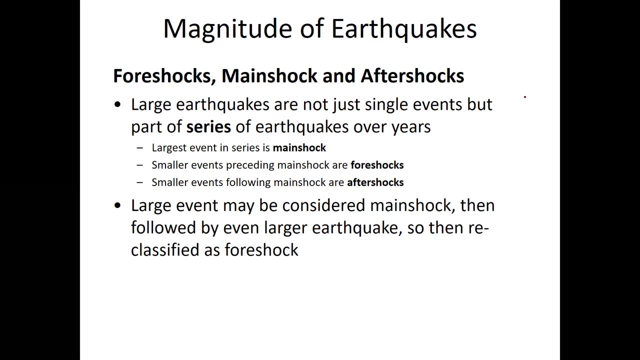 More energy that's released than a hurricane over the course of 10 days. So that's why there's so much potential in using the Sun's energy for our own energy needs. So, looking at continuing, looking at magnitude, earthquakes and foreshocks- 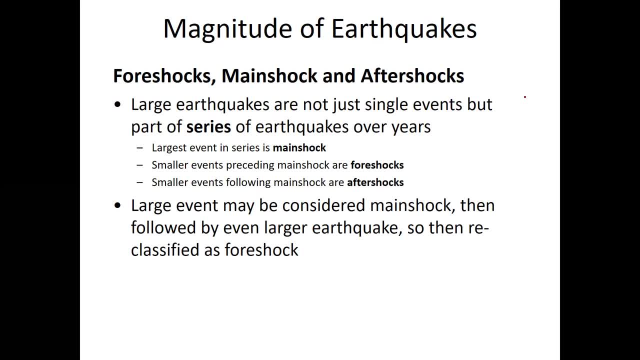 the main earthquake and aftershocks. There's a series of earthquakes that occur over some period of time: weeks, months or years. The largest earthquake in a series is the main shock or the main earthquake. Smaller ones precede foreshocks. 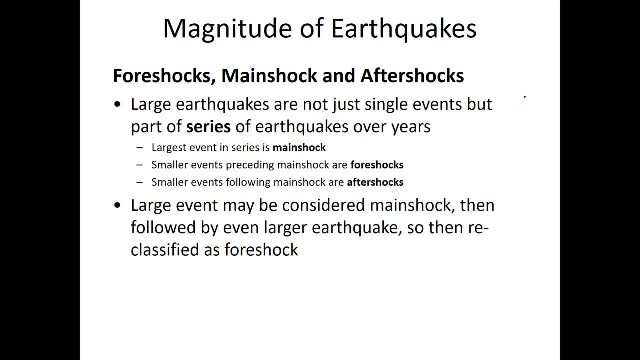 Smaller ones follow it aftershocks. A larger event may be considered a main shock. However, if it's followed by an even larger earthquake, then that originally categorized main shock is now recategorized or reclassified as a foreshock, as classified as the main shock. 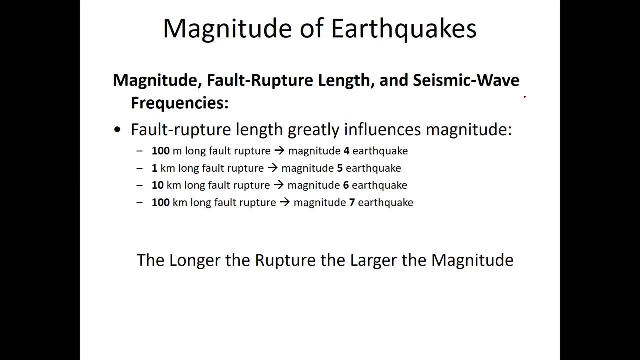 Now the magnitude of the earthquake is proportional to the length of the fault, How long of the segment of the fault ruptured during the earthquake. So a 100 meter long segment of the fault ruptures, it generates roughly a magnitude 4 earthquake. 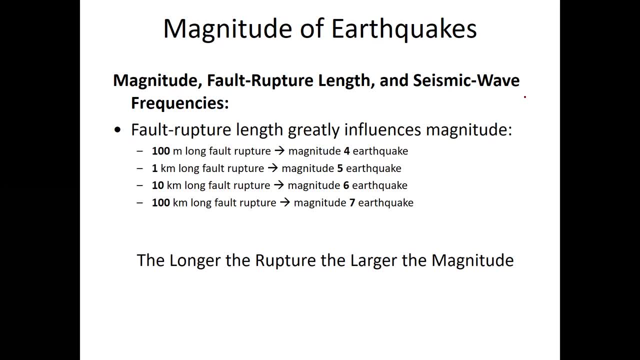 Multiply that by 10, so 1,000 meters or a kilometer long section of the fault ruptures. that generates roughly a magnitude 5.. Multiply that by 10, a 10 kilometer long segment of the fault ruptures. 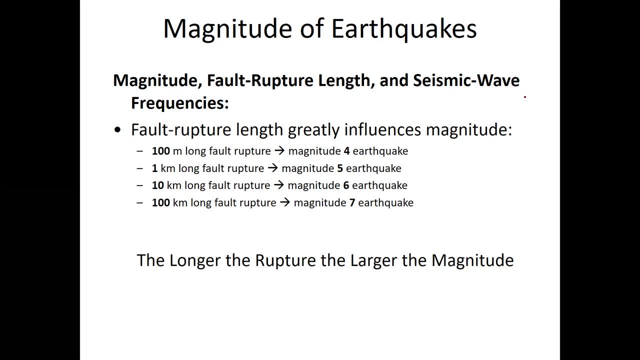 generates a magnitude 6.. Multiply that by 10, a 100 kilometer long segment of the fault ruptures roughly magnitude 7 earthquake. So we need 1,000 kilometers fault roughly to generate magnitude 8, and even bigger. 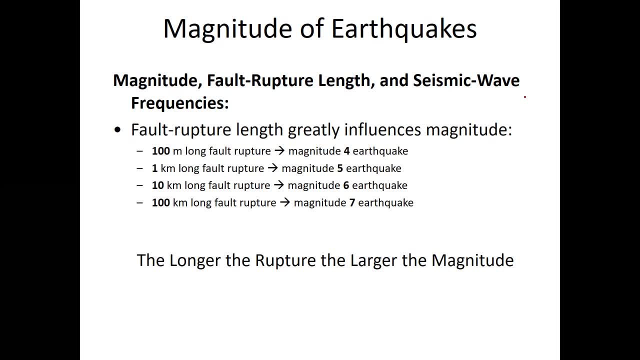 for 9.. So we would need a- you know, basically 100,000 kilometers of fault to rupture to generate a magnitude 10 earthquake, and that's just not possible because there's no faults on Earth that are that long. 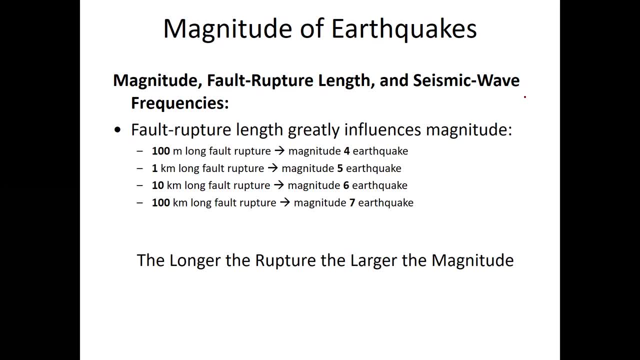 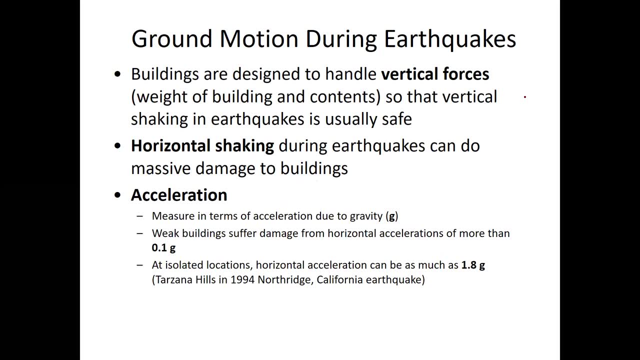 or that large. In general, the longer the segment of the fault ruptures, the larger the earthquake. Now, looking at ground motion during an earthquake. when we build buildings- at least for most of history and in most areas we build buildings- 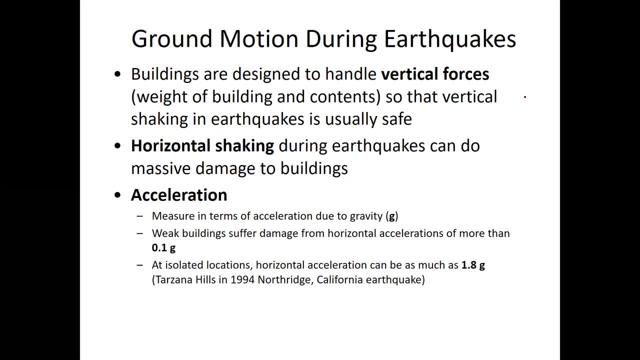 to handle vertical forces, so forces acting straight down, those forces being the weight of the building and its contents. Okay, so if the building is shaking vertically up and down, the structure is usually safe. However, if the ground moves horizontally, 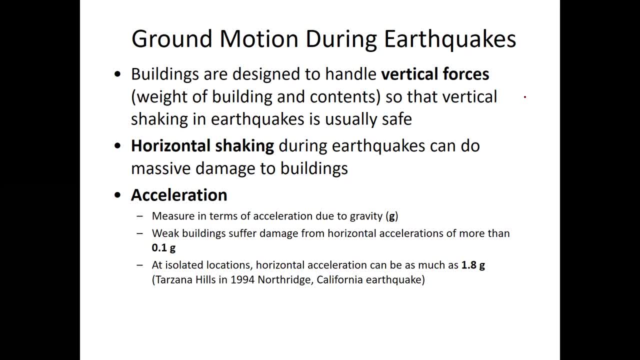 side by side. it generates horizontal forces on the building which most buildings aren't built to withstand, so that can do massive damage to buildings. It's not just the motion itself. The ground could move a lot and cause little damage to the building. 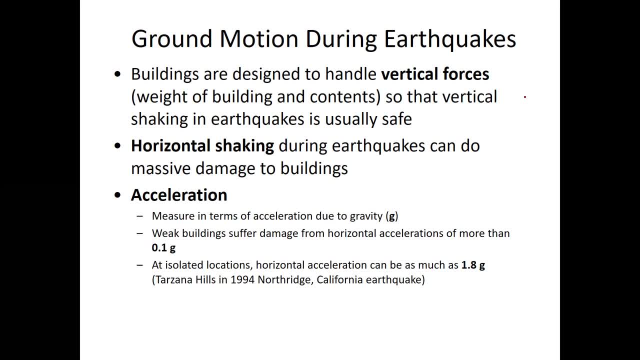 if it's moving very slowly. What's the most damaging part of the motion is the acceleration, which the acceleration is how rapidly the ground changes speed or direction. So if the ground is shaking back and forth very rapidly, that's a large acceleration. 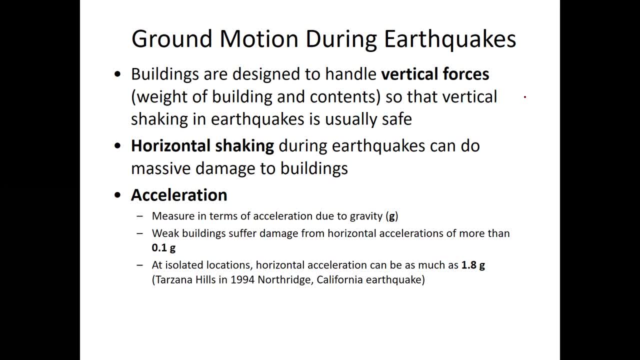 When we measure the acceleration of ground motion during an earthquake in factors of the acceleration of gravity or g, we measure the acceleration of ground motion during an earthquake. So a building will suffer weak buildings will suffer damage from horizontal accelerations of more than one-tenth. 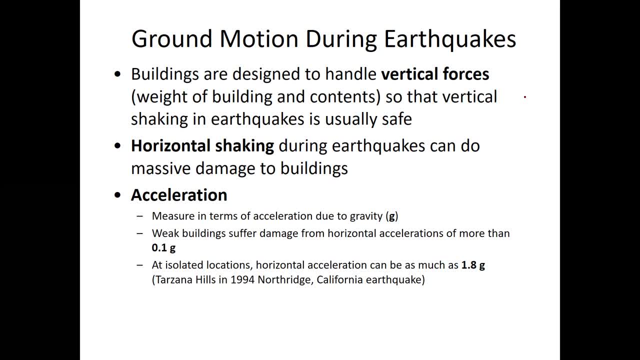 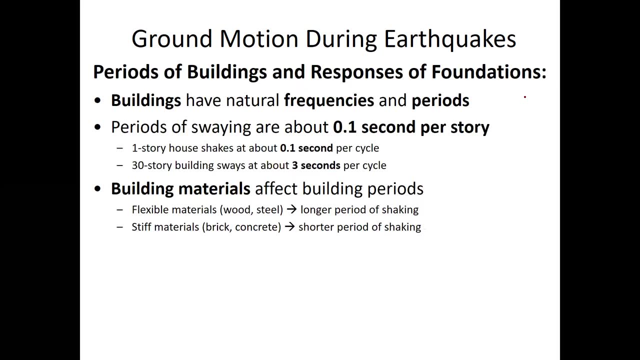 of that due to gravity, so 0.1 g. At isolated locations after large earthquakes, horizontal accelerations have been measured up to 1.8 g. So that's almost twice the acceleration due to gravity. So periods of buildings and the response: 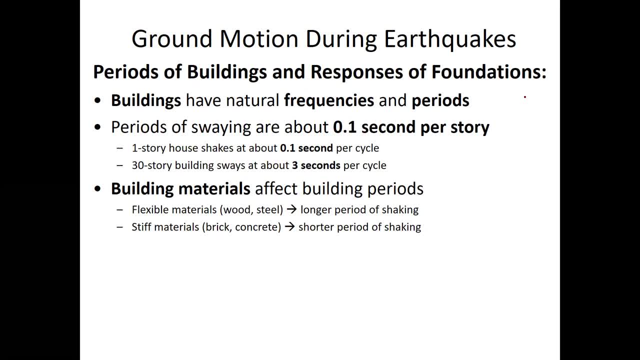 of their foundations are important to keep in mind too. So all objects that have finite mass, I should say all solids that have finite mass. they have natural frequencies in which they like to oscillate, And we know this. this is how we make. 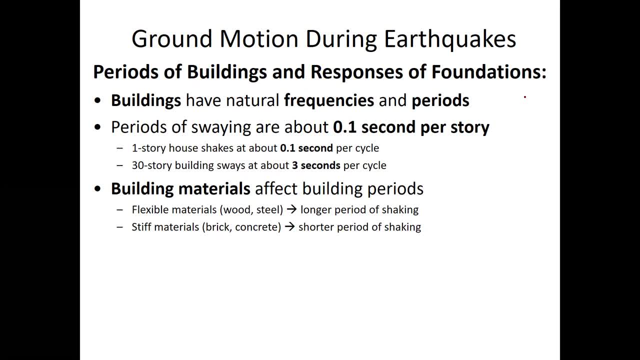 musical instruments, right, You know, strings of different lengths vibrate at different natural frequencies. And what else If we have? if we fill glasses up to different heights of water and we tap the glass, we generate different frequencies, And so 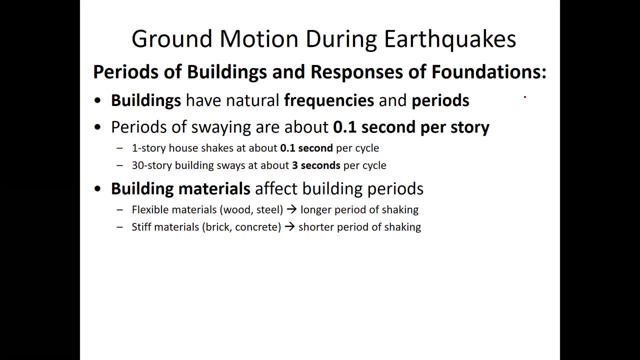 for objects that are long, like a building, is, say, if it's a tall building, its frequency is roughly a function of its height or its length, Just like the frequency at which a string vibrates is partly a function of its length, And so buildings. 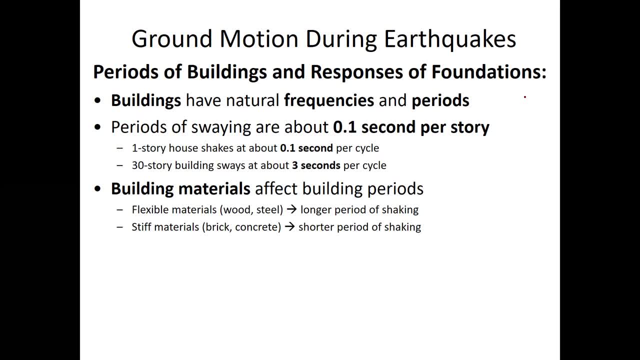 like all other objects, have natural frequencies or periods at which they want to oscillate, right, If you strike, if you pluck a guitar string, it has a particular frequency at which it wants to vibrate, Just like if you. if the ground begins to shake a building, 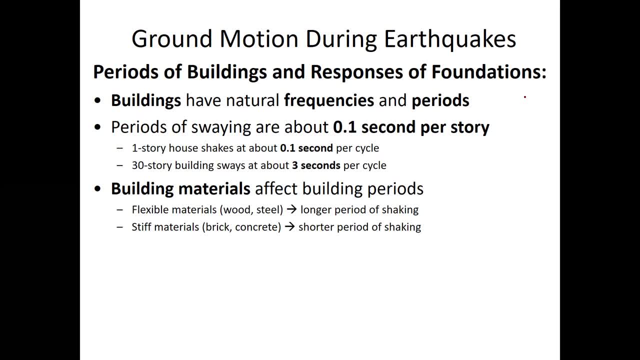 a building wants to oscillate or shake at a particular frequency or period. In general, the natural periods at which a building wants to sway or oscillate is about one tenth of a second per story. In other words, if you had a ten story tall building. 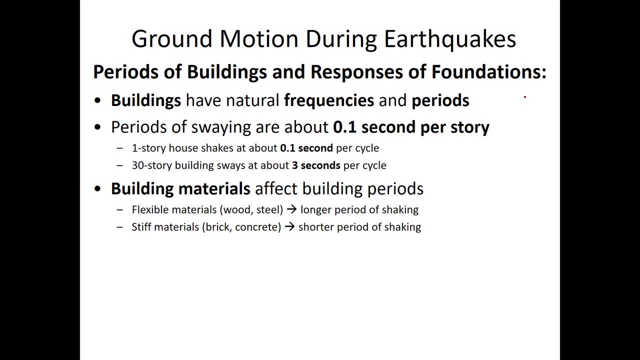 and the ground was moving, it would sway back and forth. It'll take about one second for it to make one complete oscillation. So if this is a building and it sways, it sways back and forth this way. it would take one second. 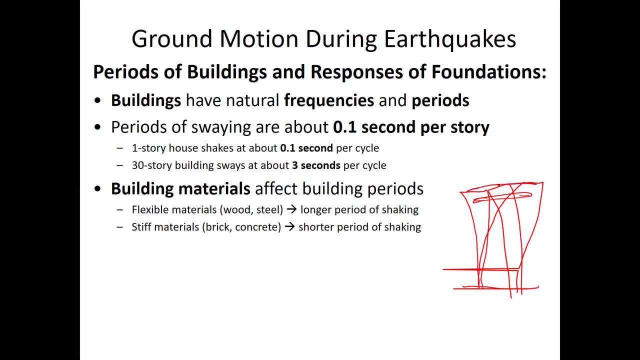 for it to go from here there, here and then back. So it's ten stories tall. If it was 20 stories tall it would take about three seconds. So a one story house. it shakes at about 1.1 second. 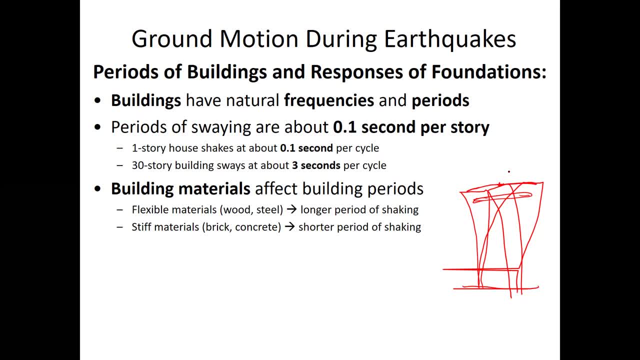 per cycle. So that means it has a period of 0.1 seconds, which is one tenth, or a frequency of ten seconds. It shakes back and forth ten times every second. On the other hand, a 30 story building sways. 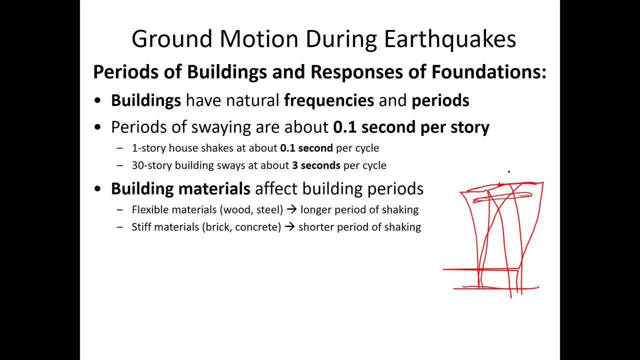 at about three seconds per cycle, So as a period of three seconds, and therefore it has a frequency of 0.33 or one third hertz. So the building height influences the frequency or period at which the building wants to oscillate. Also the building materials. 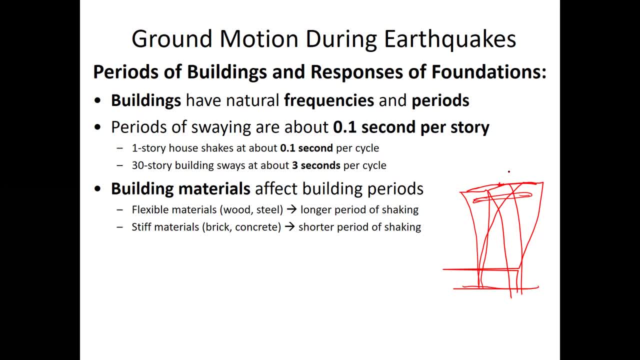 influence it as well. Flexible materials such as wood or steel. they have longer periods of shaking. So if something's flexible, it doesn't oscillate as quickly. It has a slower frequency of oscillation Where more stiff, rigid materials. 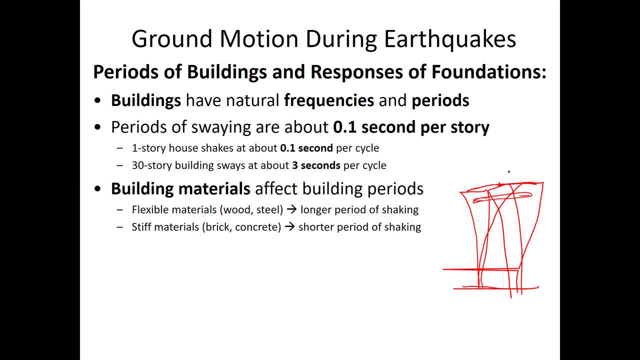 like brick or concrete. they have higher frequencies at which they want to oscillate or shake at, Just like, if you imagine, I steal a rod that's very thin and kind of flimsy and if you strike it it oscillates or shakes. 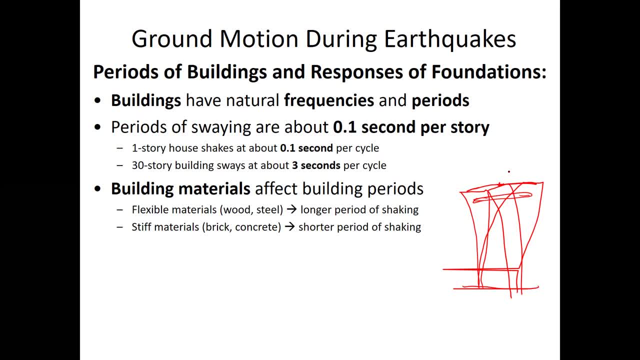 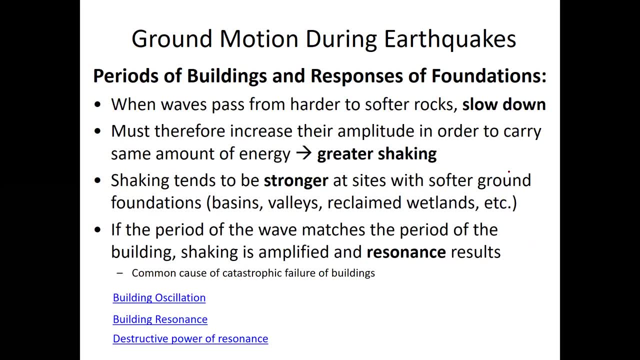 at a lower frequency, Where, if it's thicker, more rigid, it's not as flexible You strike it. it'll oscillate at a shorter period or higher frequency. So why we're talking about the frequency or period at which the building wants to shake. 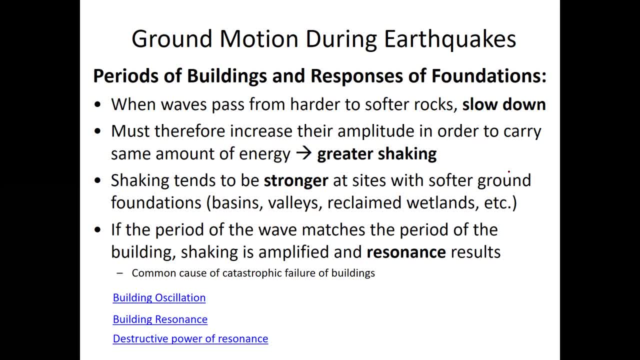 is because it's important that those frequencies or periods at which the ground shakes, the frequency or period at which the ground is shaking doesn't match the frequency or period at which the building wants to shake or oscillate. So when waves- seismic waves- pass from 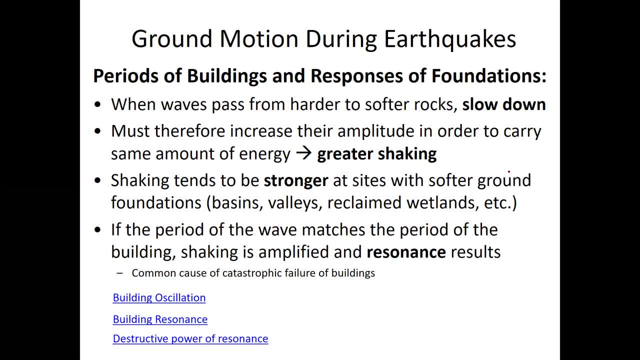 harder rock to softer rock, they slow down And, in order to carry the same amount of energy per unit time, their amplitude has to increase, which results in greater shaking. So if, as you'll find, the shaking due to seismic waves, 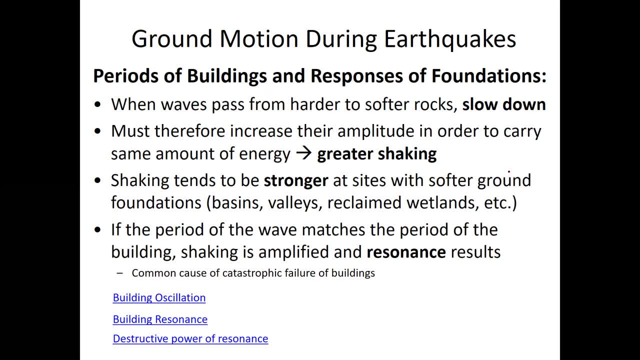 is larger. in softer rocks or unconsolidated material like sediment, sand, gravel, silt, the shaking is amplified. In consolidated, harder material like bedrock, shaking is smaller. It's somewhat diminished, So shaking tends to be stronger at sites. 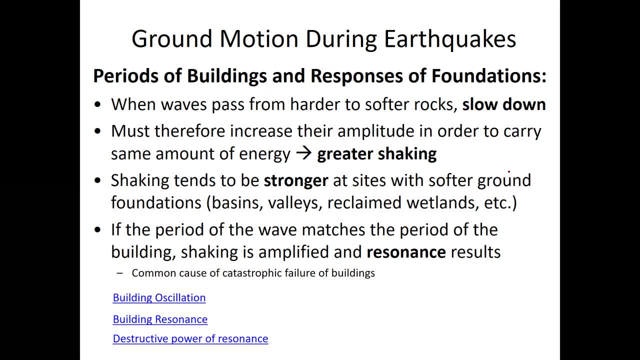 with lower ground foundations and we find those softer grounds in lower elevations where sediments accumulate- basins, valleys, reclaimed wetlands, etc. And if the period of the wave traveling through these materials matches the period of the building, the shaking is amplified. 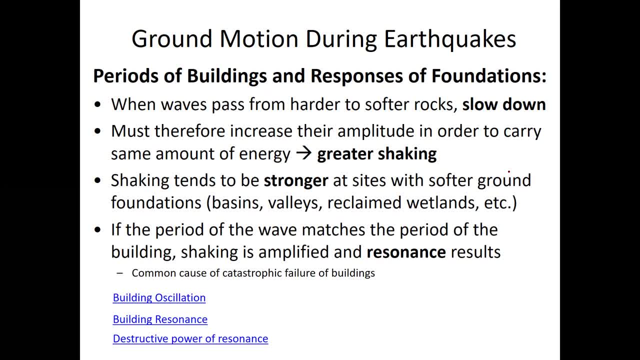 in the building and a process known as resonance occurs, And resonance is a common cause of catastrophic failure of buildings. I'll leave these three links here. These videos are in a supplemental video folder for this chapter which you should check out. So it shows buildings in Tokyo. 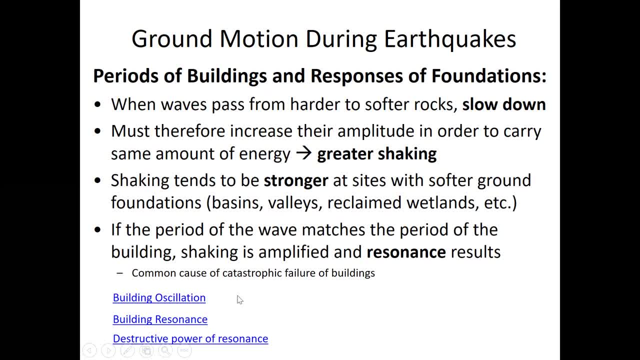 oscillating back and forth after an earthquake. So you can see this process of buildings oscillating, You can see building resonance, where there's three different mock structures, model structures, on a platform that's shaking back and forth by an actuator And the frequency 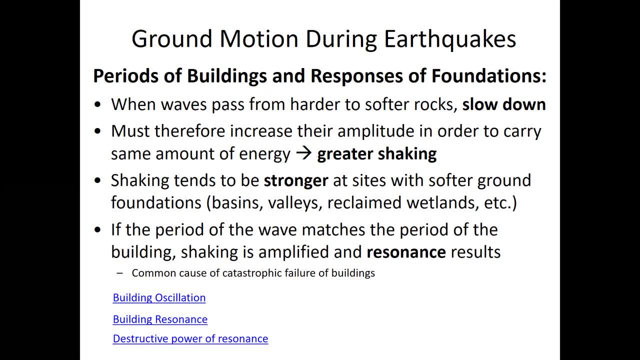 of shaking is dialed up and, as it's dialed up, you can see that the frequency of shaking resonates or matches the frequency at which buildings which I forgot to mention, all three of them are three different heights, which they want to. 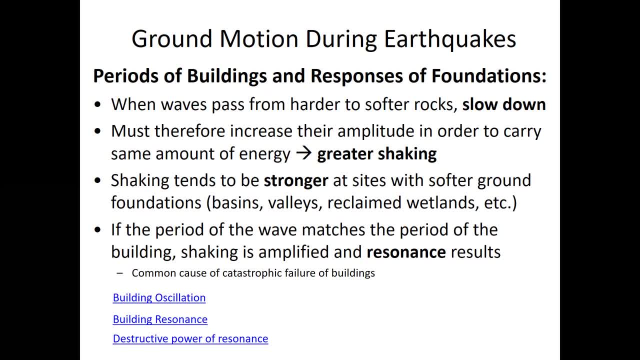 want to shake And you can see it's fairly dramatic when the platform shaking of the platform is resonating with the building. The shaking of the building, the oscillating of the building, is amplified in what's called resonance In the final video. 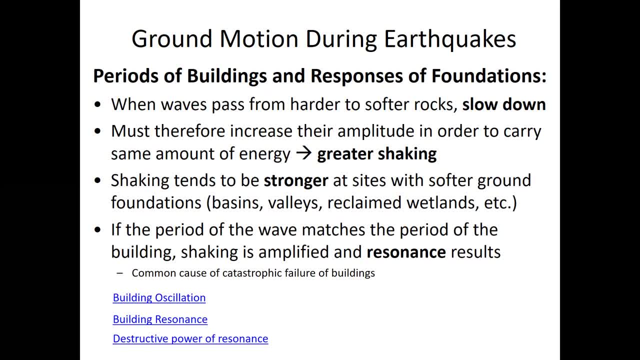 it shows the destructive power resonance, how the wind resonating with the Tacoma Narrows Bridge in Tacoma, Washington, caused the resonance and caused the bridge to bridge, oscillations to amplify and eventually caused it to fail. So I encourage you to check out those videos. 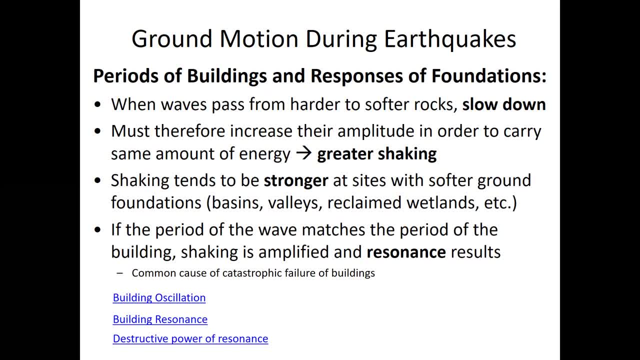 But basically, simplistically, you can imagine. you can get an idea of what resonance is by thinking about pushing a child on the swing. The child swings at a particular frequency. How many swings per second? or are they swinging at a particular period? 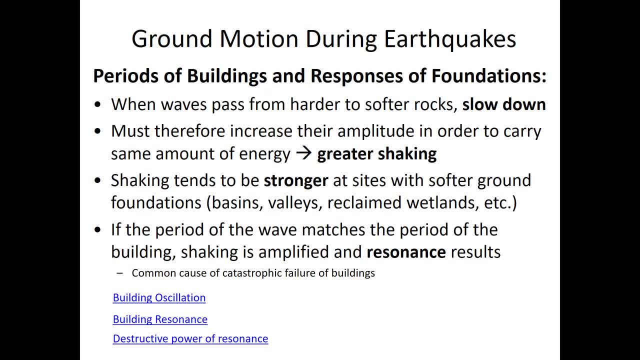 How long it takes for them to make one oscillation. In order to make them swing higher, you have to push them at a frequency that matches the frequency at which they are swinging, Or at a period that matches the frequency at which they are swinging. 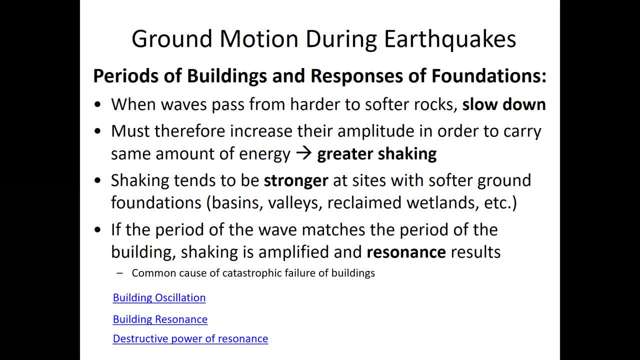 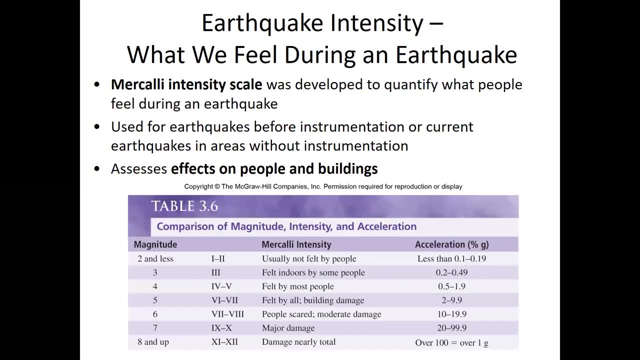 And if you push them at the same frequency, what happens is they swing higher and higher and higher, Because your pushing is resonating with their oscillating And that's resonance and causes the oscillation to increase in amplitude. So the earthquake intensity. 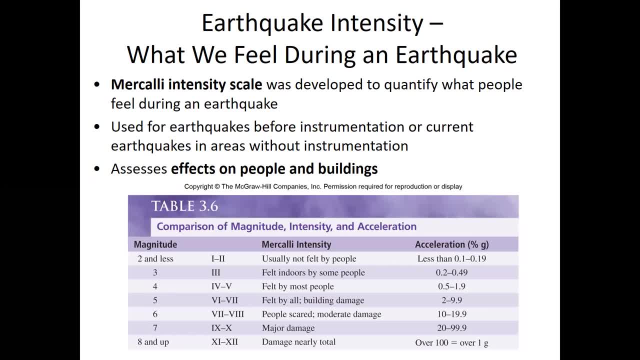 that's what we feel during an earthquake. It used to be well. it still is, but it primarily used to be indicated by the Merkelli intensity scale. This was developed to quantify what people feel during an earthquake. It's primarily used for earthquakes. 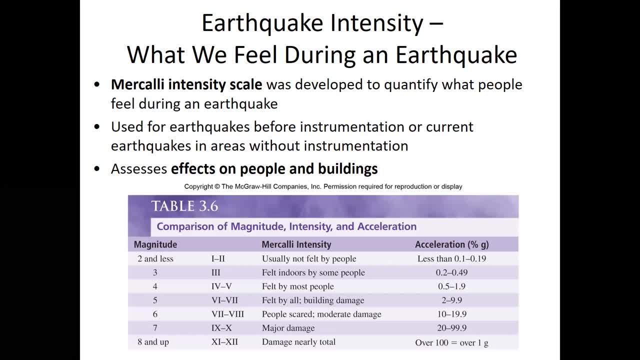 before instrumentation, before we had seismometers to measure seismic waves, And it's also used currently in areas where the earthquakes occur that we don't have instrumentation deployed And the Merkelli intensity scale. it assesses the effects on people and buildings. 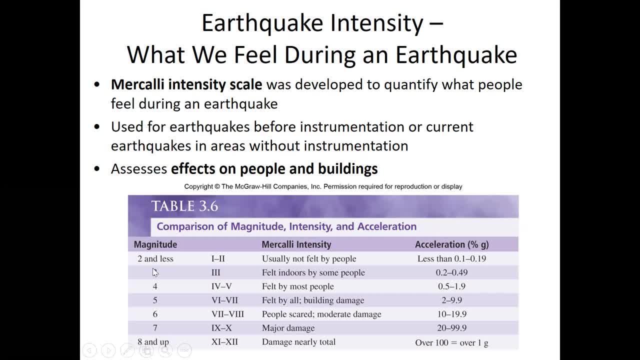 So this is the magnitude of the earthquake in the left hand column And this is the corresponding Merkelli intensity scale. It goes from one to two, three, four to five, six to seven, eight to nine- oh sorry, seven to eight. 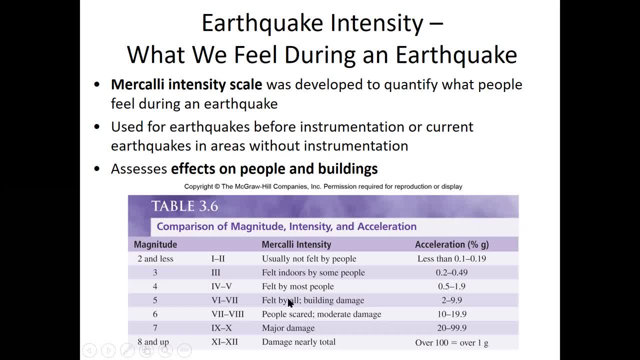 nine to ten and then 11 to 12.. And this is a description of what those intensities, what sort of impact they have. This is the corresponding acceleration as a percent of g, And so that's a 10 to 12. 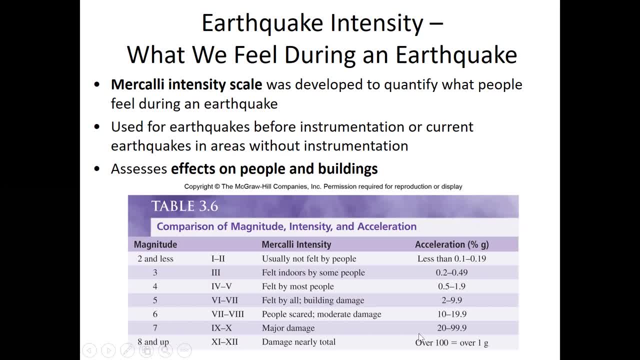 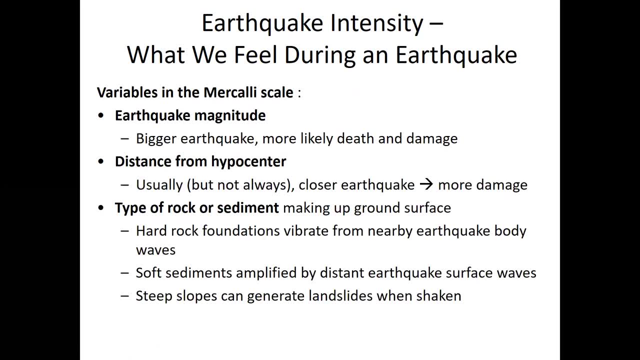 on a Merkelli intensity scale And that's where the acceleration is more than that due to gravity. So some variables in the Merkelli scale is the earthquake magnitude. The bigger the earthquake, the more likely there is to be death and damage. 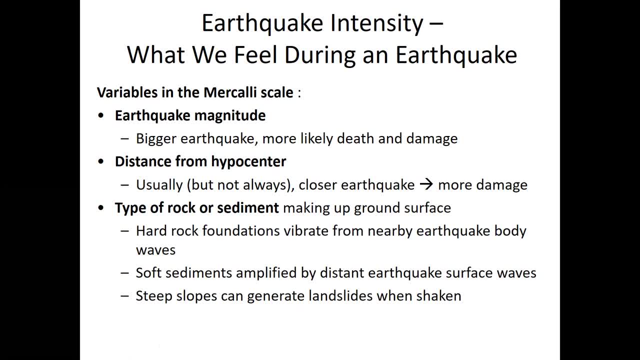 and therefore larger ranking on the Merkelli scale, Distance from the hypocenter, usually, but not always, or the Merkelli intensity scale And finally, the type of rock or sediment Making up the ground surface. Hard rock foundations vibrate. 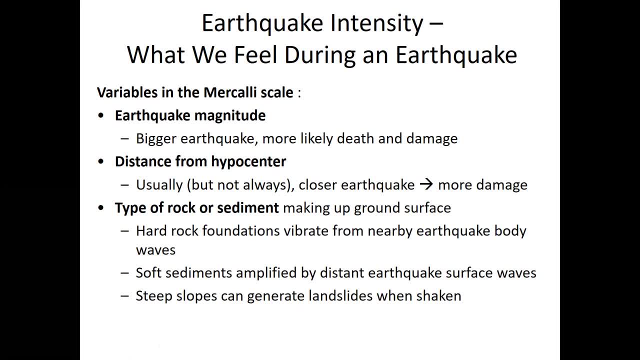 from nearby earthquake body waves, So the high frequency body waves. they tend to resonate with harder, more consolidated material bedrock, where soft sediments are amplified by rigid shore buildings And so steep slopes can generate landslides when shaken as well. 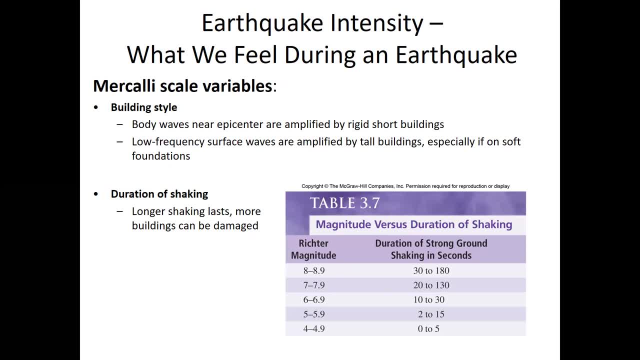 So more Merkelli scale variables. The building style. So body waves near the epicenter are amplified by rigid shore buildings Because, remember, body waves have higher frequencies and resonate with buildings that have higher natural frequencies, which are shorter, more rigid buildings. 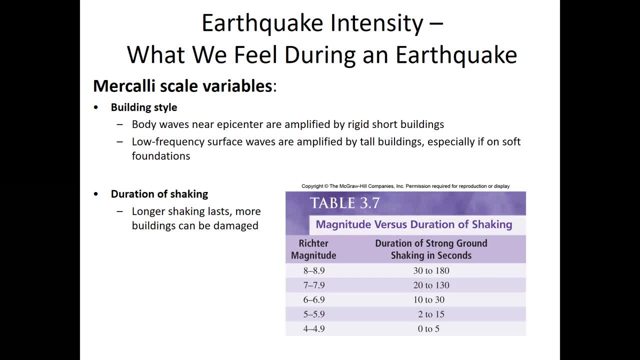 Where the lower frequency surface waves they're going to be amplified or resonate with tall buildings, especially if they're on soft foundations. So basically, the intensity of the shaking can be increased if close to the epicenter, So if we have short, rigid buildings. 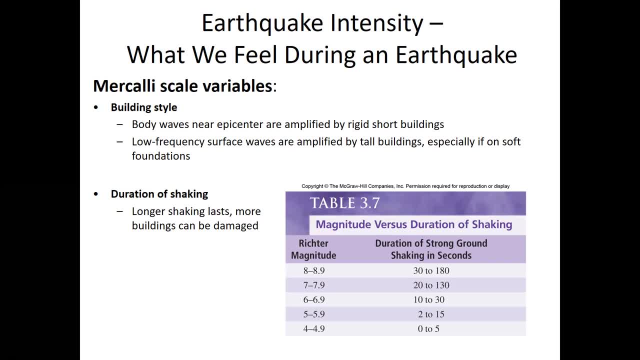 on solid rock close to the epicenter, that'll intensify the shaking more. And if we have tall buildings built on soft material further away from the earthquake, those surface waves will resonate with those buildings and intensify the shaking as well. Where, conversely, 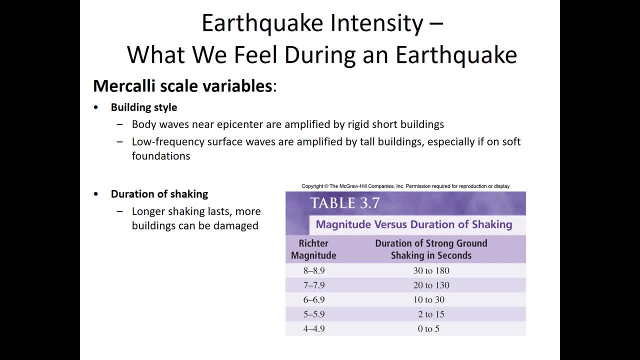 if we had tall, flexible buildings built on bedrock close to the earthquake, there'd be a lot of shaking in the building. And if we had short, rigid earthquakes built on soft materials far from the earthquake, the surface waves would not resonate with those buildings. 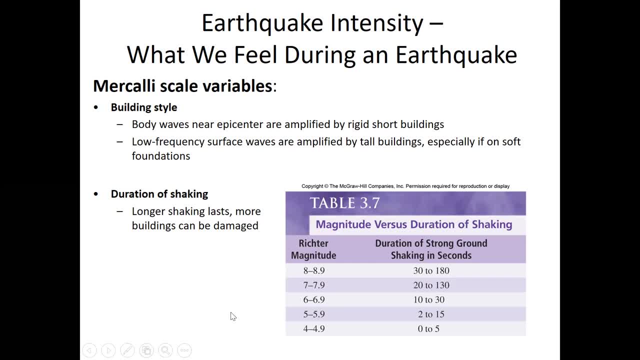 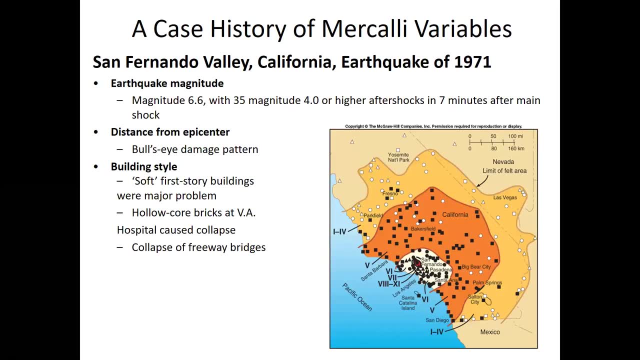 resulting in minimal shaking. And finally we have the duration of the shaking. Obviously, the longer the shaking lasts, the more buildings will be damaged. So here's a case history of these Markeli variables. This is the Markeli earthquake in 1971,. 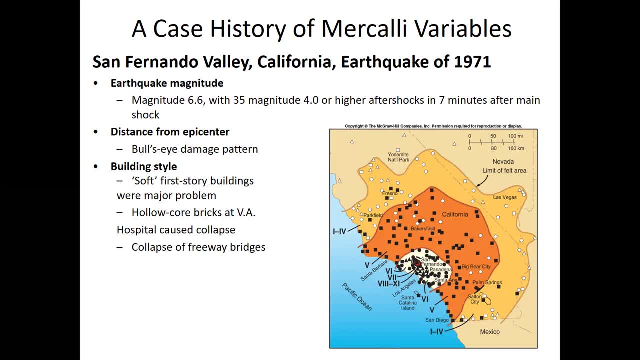 the San Fernando Valley. The earthquake was a magnitude 6.6, with a 35 magnitude 4 or higher aftershocks and 7 minutes after the main shock. And so you can see these colors represent the different Markeli scale rankings, So the highest. 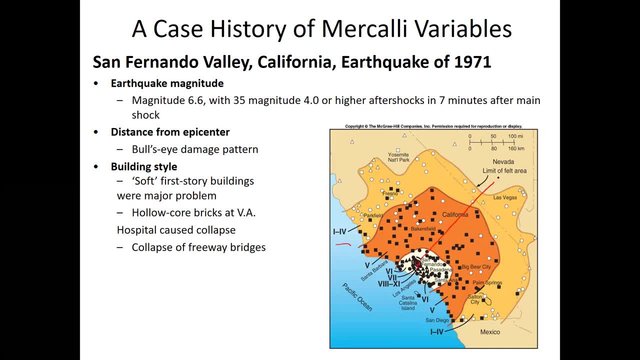 is in the center and as you move away, the Markeli intensity decreases, creating this bullseye damage pattern. Obviously, the shaking is the highest to center and it decreases with distance away. You can see there's these little tongues out here. These tongues are partly following. 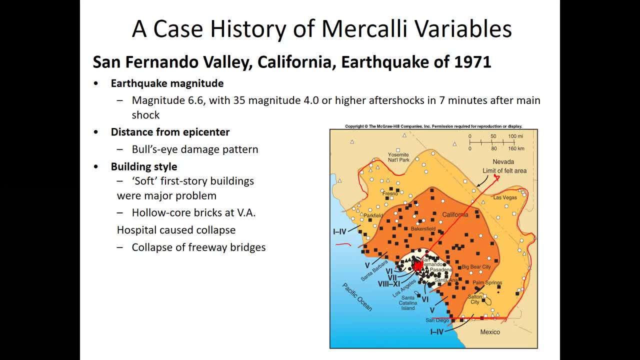 where there's people that make observations right Building style is a factor. as we said, soft first story buildings were a major problem. Hollow core bricks at the Veterans Affairs Hospital caused collapse and collapse of freeways and bridges were very destructive. So this soft first story. 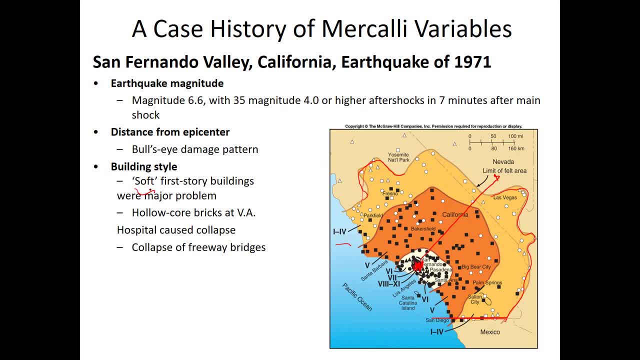 buildings, that's, buildings that basically have a garage as the first floor. So it's not a very sturdy forced floor and they're very susceptible to collapsing. And the hollow core bricks, gray cinder blocks, they're hollow, This Markeli scale. 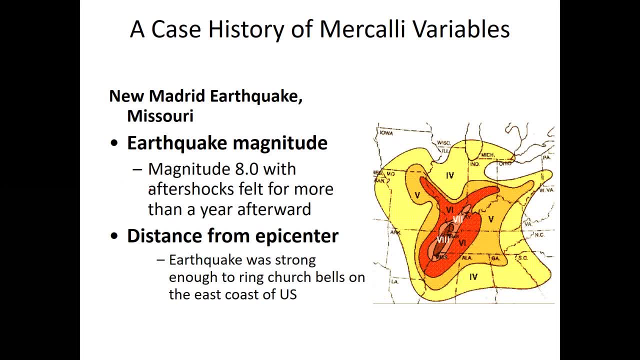 intensity map doesn't have the same symmetric bullseye shape as the last one. This is the New Madrid earthquake that occurred in Missouri near the turn of the year 1811-1812.. It was a 1928 earthquake and aftershocks were felt. 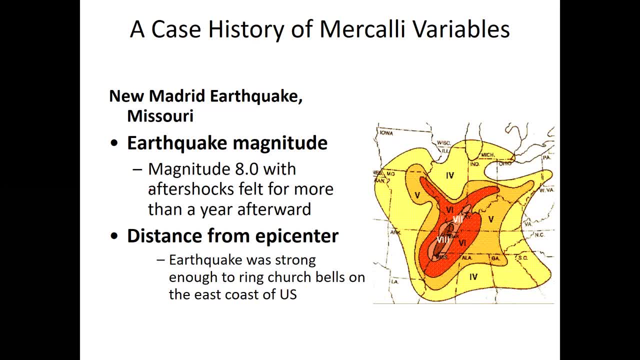 for more than a year afterwards. So the earthquake was strong enough to ring church bells on the east coast of the United States. But you see how the Markeli intensity scale the pattern, instead of being a symmetric circle bullseye, it kind of 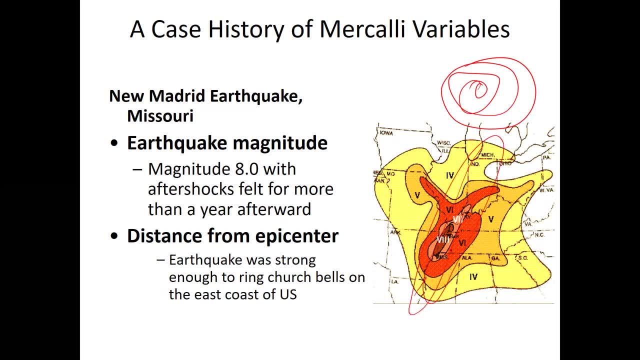 runs more oblong. Why is that? Because, remember, we said that soft sediments amplify the shaking And this this fault. it runs along Mississippi River, So this is the Mississippi River Valley, right here. So the Mississippi River runs along here and so the shaking. 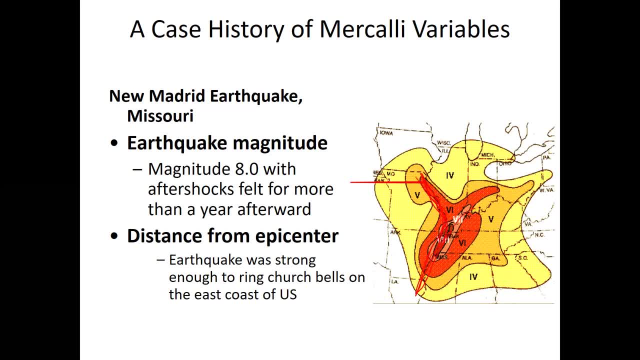 was amplified by these sediments in the Mississippi River. Then this is the Ohio River Valley And so the shaking it was intensified going up through the Ohio River Valley. So you can see how the shaking kind of reverberated through these soft sediments. 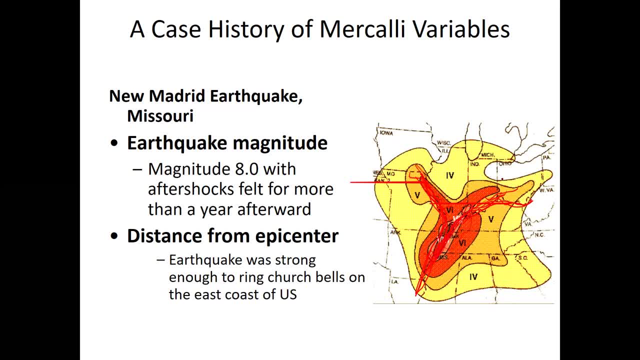 that are deposited in these by the rivers, in these valleys, And because the east coast of the United States isn't as fractured and mangled due to less recent tectonic activity, as compared to the west coast of the United States, the seismic energy can travel. 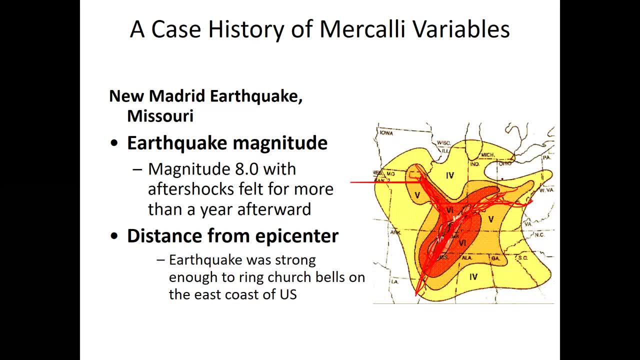 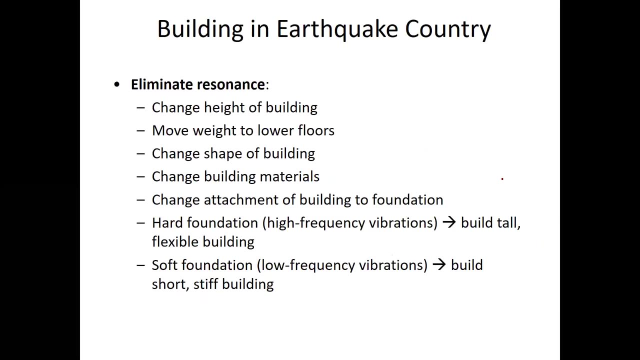 through the ground more coherently, without being scattered, so it can travel further, So it's not dissipating as much, And that's another reason why this earthquake was felt so much further away than the ones in California. So if we're going to build, 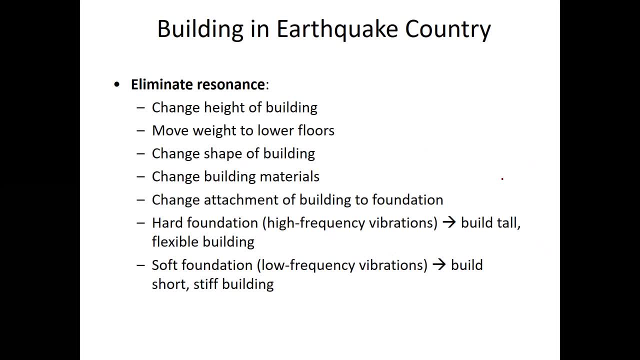 in a region that has a seismic hazard. when we build our buildings, we want to make sure that we're eliminating residents. We do not want the frequency at which the ground is shaking to match the frequency at which the building wants to shake. So how do we eliminate residents? 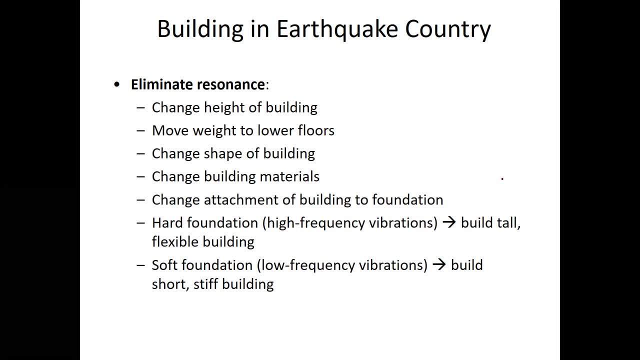 Well, we can change the height of the building. We know that surface waves- long-period surface waves- are amplified in soft materials. So if we're building in soft materials, like in sediments in a valley, we want to build short, rigid buildings. 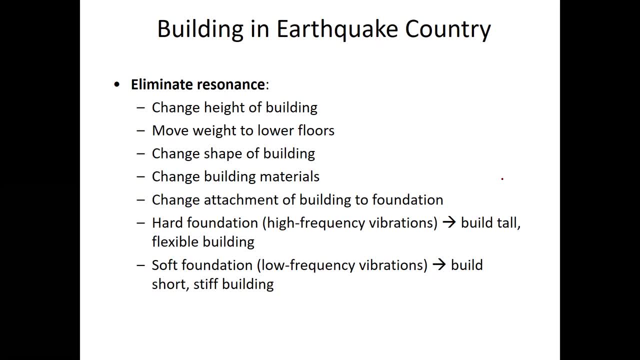 We know that high-frequency body waves are more prominent in in in harder consolidated materials like bedrock, And so we want to build taller, more flexible buildings. in the bedrock We can move the weight of the buildings, concentrate the weight towards the lower parts of the floor. 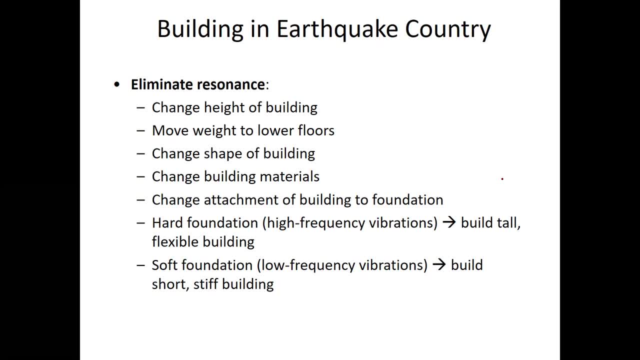 instead of higher in the building. The higher the weight is distributed in the building, the more it wants to shake, Change shapes of the buildings so they are broader at the bottom instead of just. you know, these rectangular objects, rectangular shapes, Change building materials. 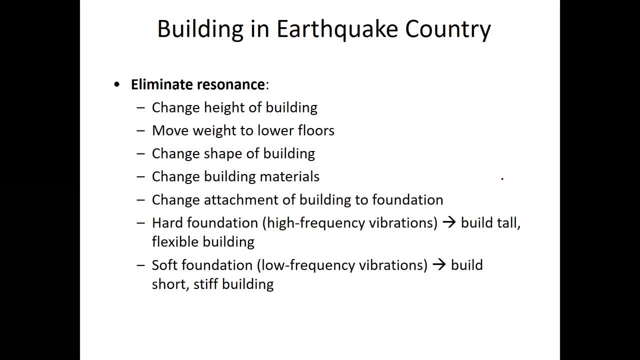 Flexible materials have more, give Wood and steel where concrete materials- brick, stone- they're not as forgiving. If they have any horizontal motion they can crack and be compromised and fail. Change the attachment of the building to the foundation. We'll talk about this in a little bit. This is called base isolation. 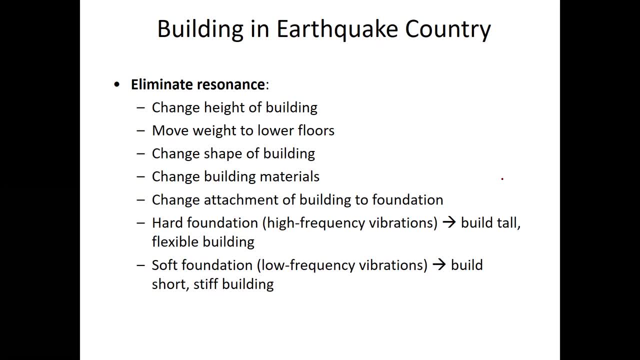 How to decouple the building from the ground so that the building doesn't necessarily, the base of the building doesn't necessarily have to shake at the same frequency which the ground is. And so, as I said earlier, if we have a hard foundation, we have 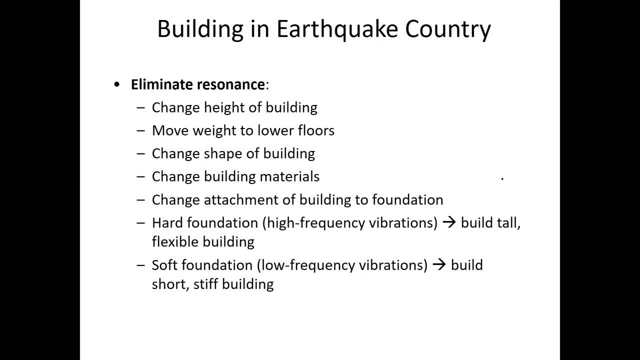 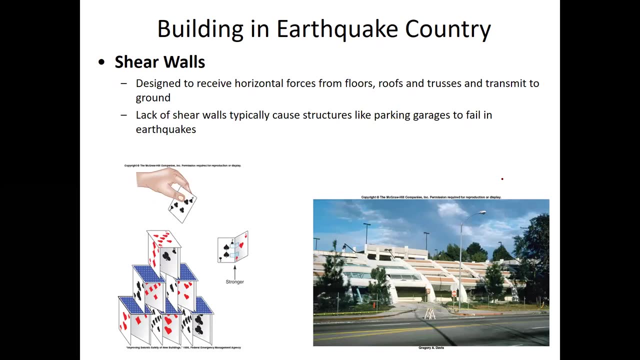 higher energy. higher frequency waves are going to be higher energy, so we want to build tall, flexible buildings. If we have soft foundations, such as sediments, the lower frequency vibrations are going to be more energetic. So we want to build tall, flexible buildings for buildings, to avoid resonance. 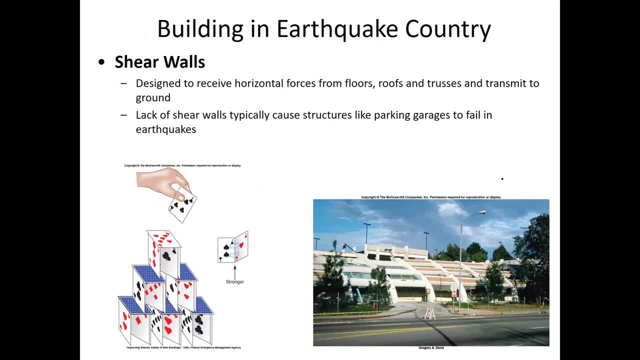 We could also build shear walls. So shear walls are designed. they're walls designed to be able to withstand horizontal forces on floors, roof trusses, and transmit those forces down into the ground. The lack of shear walls typically causes structures like parking garages to fail. 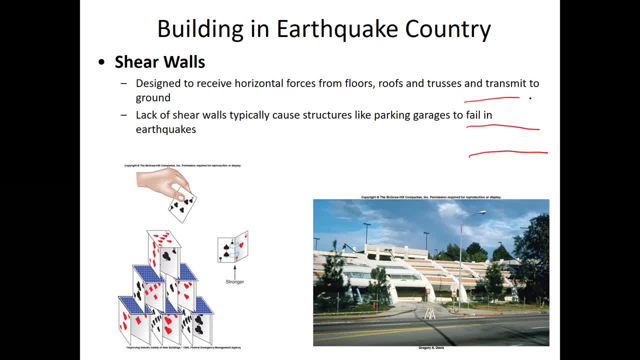 So a parking garage has these levels but they only have these pillars that support the vertical stresses. There's no shear walls or basically there's nothing to support horizontal stresses. So if you can build some way some horizontal supports in there that can support these horizontal stresses, 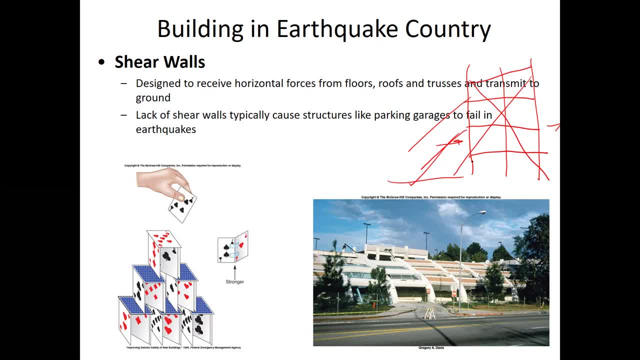 and transmit them down to the ground and prevent the building from collapsing. So here's a parking garage in California. You can see these angled members here are helping create horizontal strength. So it's almost like taking a house of cards which has no horizontal strength. a light breeze could blow it over. 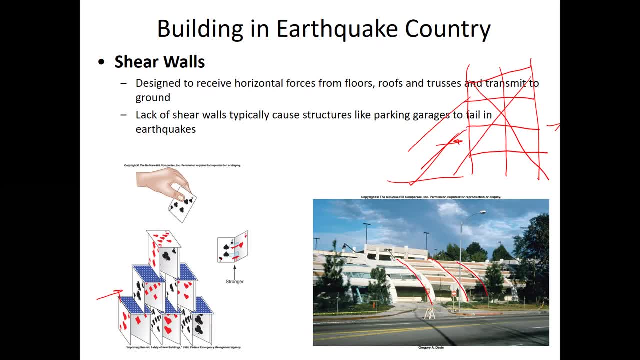 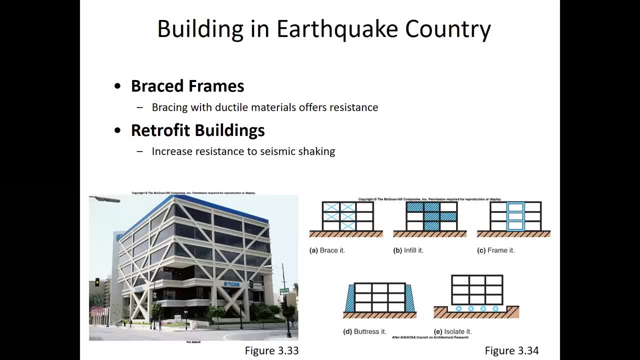 and just reinforcing the cards. adding some tape gives them some horizontal strength, So less likely to fail in the event of horizontal stress. So other ways we can create horizontal stresses is using braced frames, Cross bracing within the framing of the building or 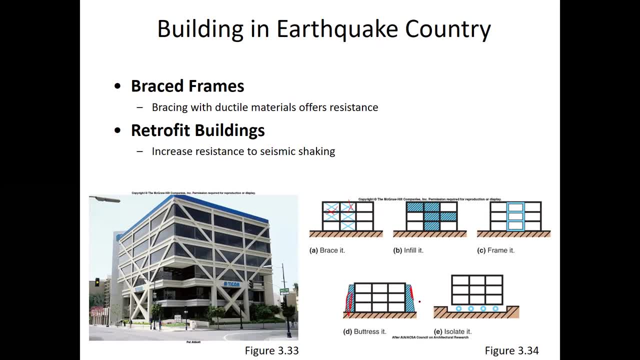 buttressing the building, or we can even isolate the building from the ground completely. This is called base isolation. So say, if we put the building on rollers, the ground is shaking back and forth. the ground doesn't necessarily have to shake as the same as the ground, since it's on. 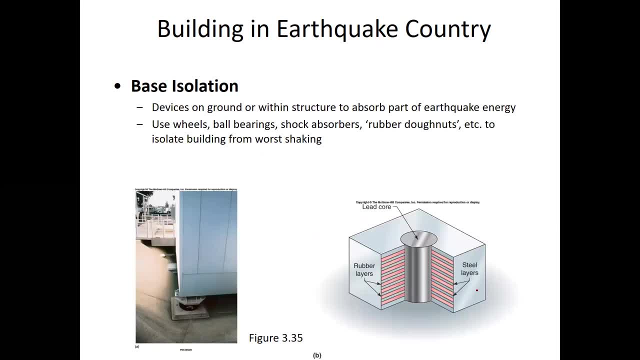 rollers, And there's different ways of base isolation, where you can put the building on pillars and those pillars then go down into the ground and are surrounded by these layers of rubber and steel So as the ground shakes, the energy is absorbed. it's kind of like a cushion. 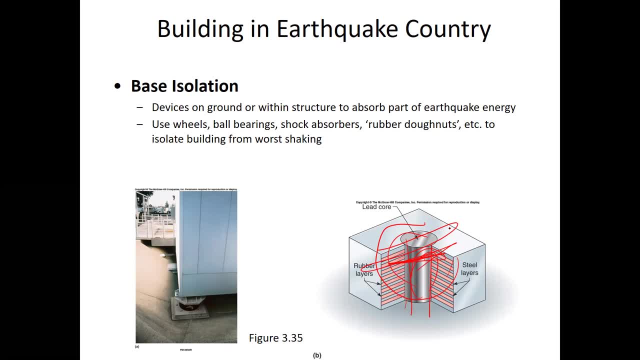 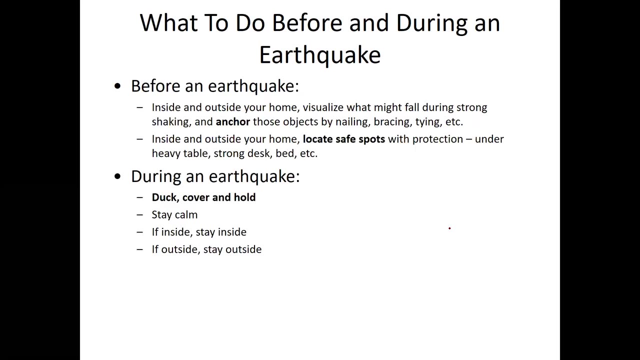 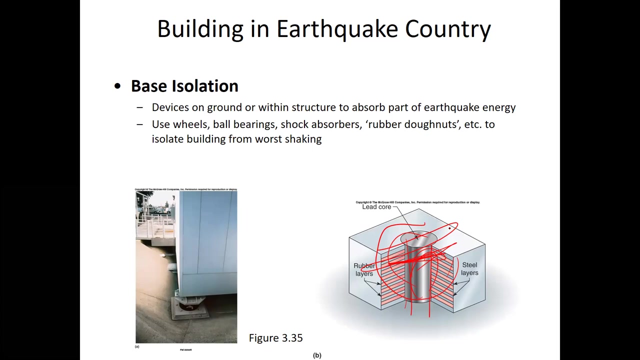 and it dampens the shaking, So not all the energy is transmitted up to the building, so the building does not shake with the same vigor as the ground. So these are all techniques which we can use to build buildings that are more resistant to collapse during the event of. 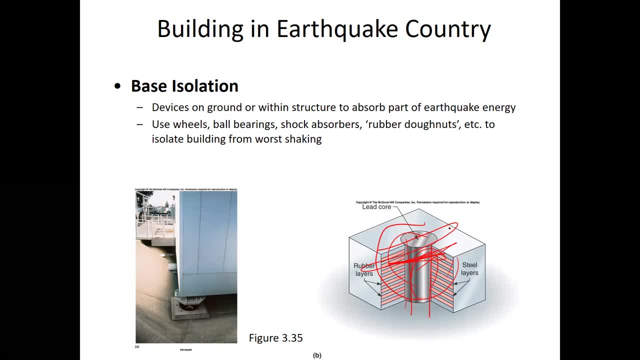 an earthquake and seismic waves traveling through the area And many regions of the of at least this country and other countries, developed countries. they have building codes In regions where there's seismic hazards, called seismic codes, in which buildings have to be built in order to withstand. 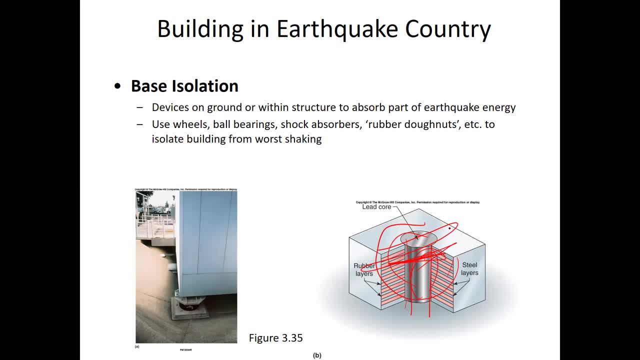 these horizontal stresses And existing buildings need to be retrofitted. That's why, whenever the 2010 Haitian earthquake occurred, it was so devastating to Haiti, because their infrastructure was not built to withstand horizontal shaking, so everything failed. Where, if that same size earthquake? 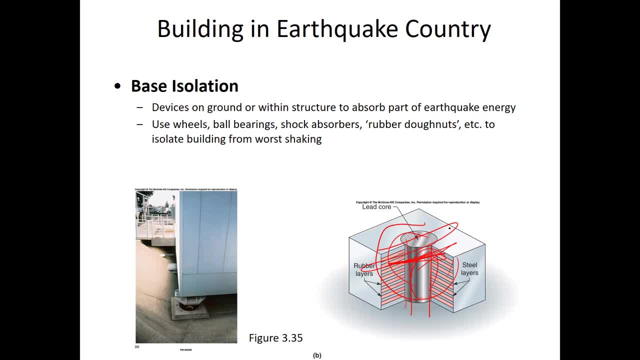 were to occur, say, in Tokyo or Santiago, Chile, or San Francisco, California, there would be much less damage because the infrastructure is built to withstand those horizontal forces and it's built to try to mitigate the amount of resonance. So that's an example of how 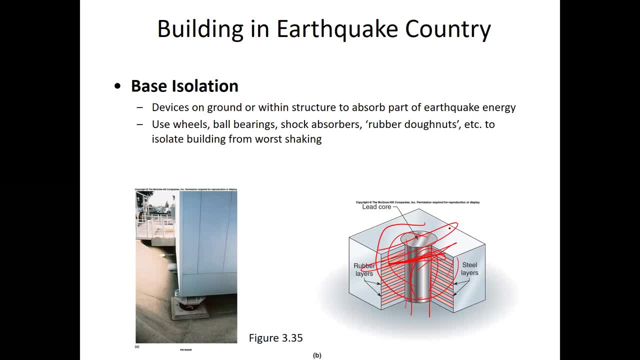 having the resources and having the government to make sure that the infrastructure is built in a way to mitigate the negative impacts of seismic waves on our infrastructure is important to save lives. One thing about earthquakes is that they themselves do not kill people. Imagine yourself standing in the middle. 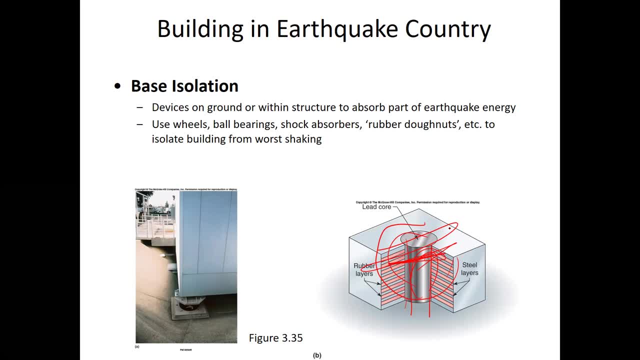 of a large, wide open field and an extremely large earthquake occurs. What is the worst thing that's going to happen to you? You're going to fall down. Maybe you sprain your wrist, At worst you break it. You're not going to perish, though. 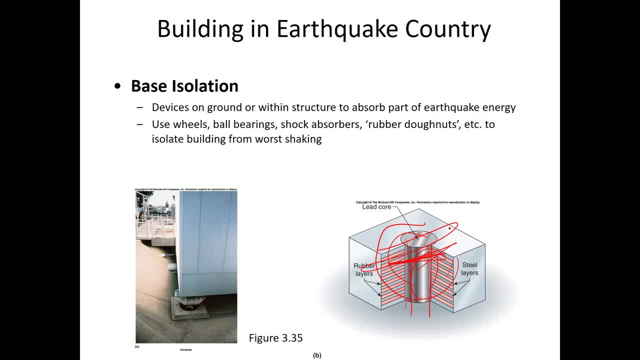 Your life is in no significant peril. What does kill people in the event of earthquakes? are buildings falling down, falling on their head? It's fires from gas lines breaking, electrical lines breaking, igniting the gas leaks. The fires cannot be fought. All the debris and rubble 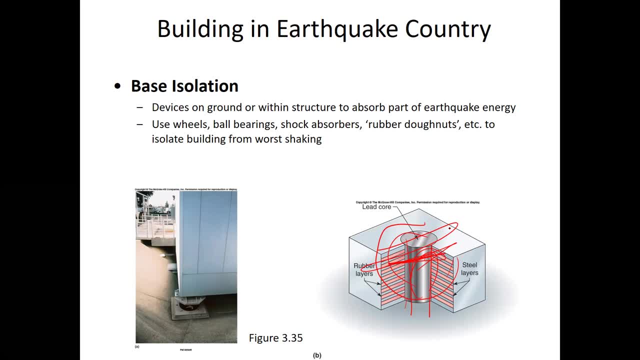 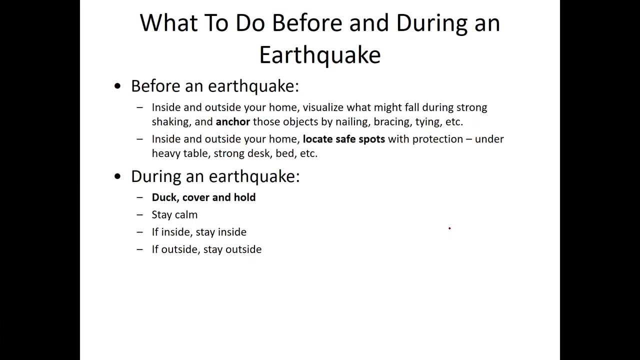 provide fuel from the fire. You have these widespread fires. It's the failure of infrastructure due to an earthquake that kills people. Once again, it's not earthquakes that kill people. it's the failure of infrastructure during an earthquake that kills people. If you find yourself, 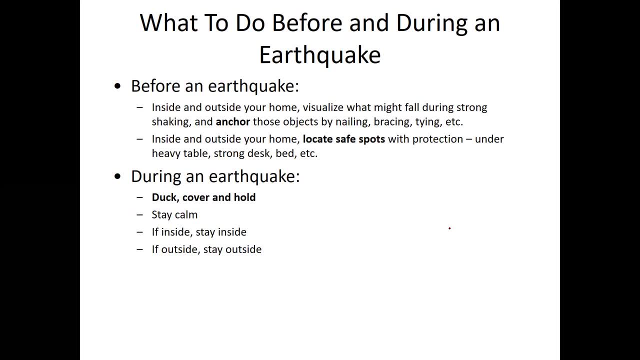 in a region that has a significant seismic hazard and you are unfortunate enough to experience a large earthquake- or let's say we're not there yet- say you could experience a large earthquake. what should you do prior to mitigate the effects of an earthquake Inside and outside your home? 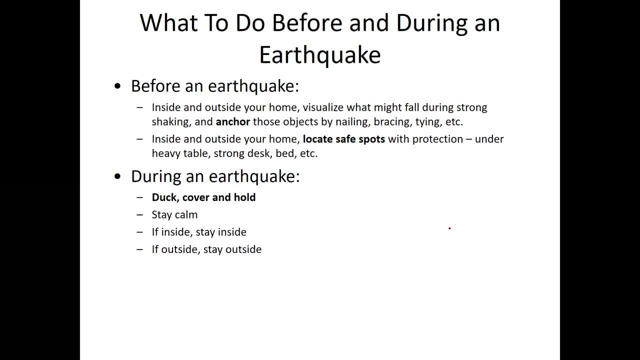 you should visualize what's going on If you're living on the east coast. often times when you buy furniture, I always find it found it odd whenever it comes with the anchoring supplies to anchor the bookcase or dresser to the wall. I mostly thought: 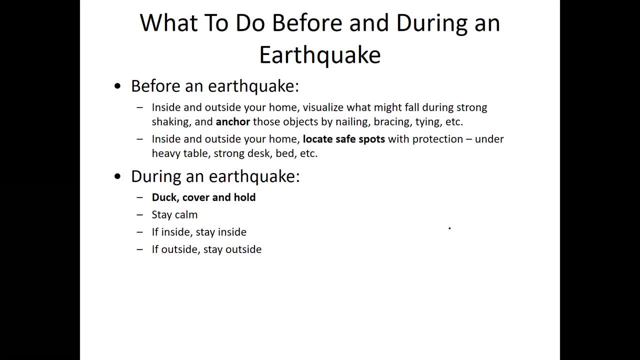 this is to prevent a child from pulling it down on themselves. They want to anchor their furniture to the wall, such as a bookshelf, a large, tall bookshelf- because they don't want that bookshelf to fall over on anyone in the event of an earthquake. 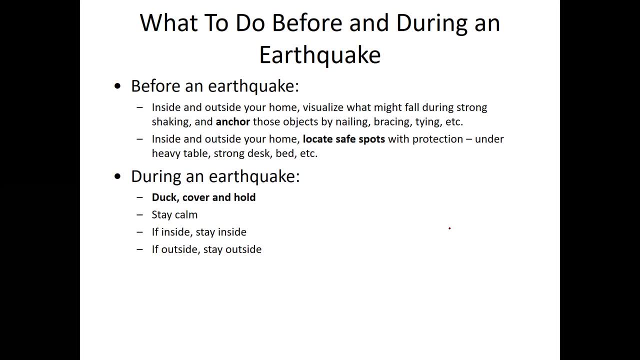 So they want to anchor it to the wall. Anything that's hanging overhead- light fixtures and so forth- I want to make sure that they are strongly anchored in safe spots with protection. So protection from what? Protection from falling objects? So you want to get under a heavy table. 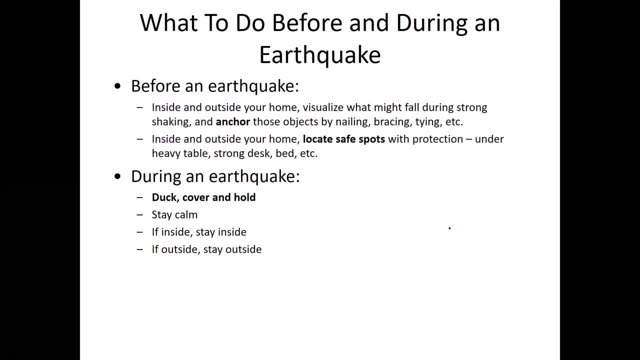 a strong desk under a bed in a doorway. If you are in a doorway, it's very hard for something to fall on you because you're in a doorway. You want to make sure you stay away from any overhead glass though, So that's before an earthquake. 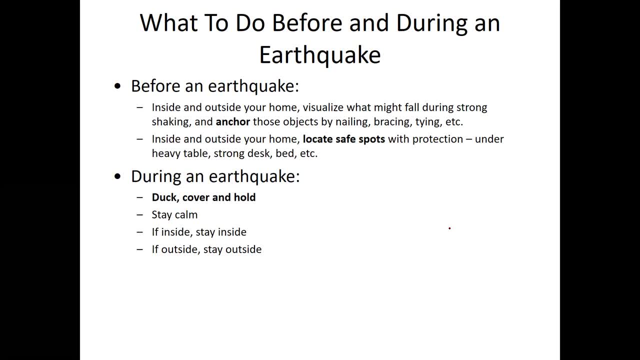 During an earthquake, you want to duck, cover and hold. Stay calm. If inside, stay inside. If outside, stay outside. Do not go into or out of a building, because it's on the outsides of buildings that often objects are falling from large heights. 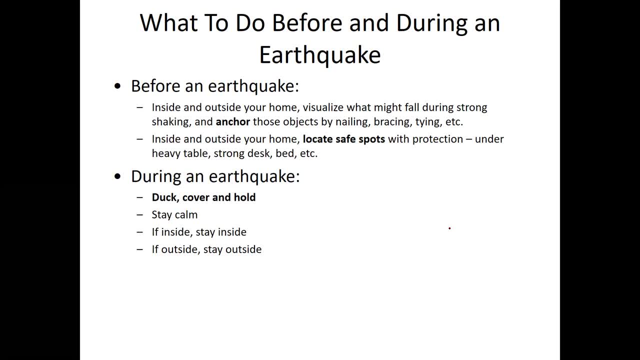 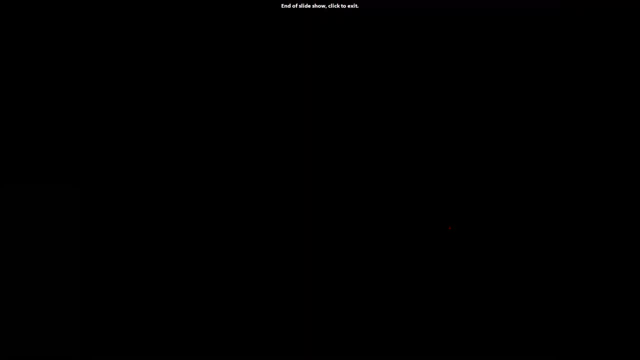 and are very deadly. So you have a greater chance of being struck by those objects as you're entering or leaving a building. That's why it's best to not enter a building or leave a building during an earthquake. So this concludes our lecture on 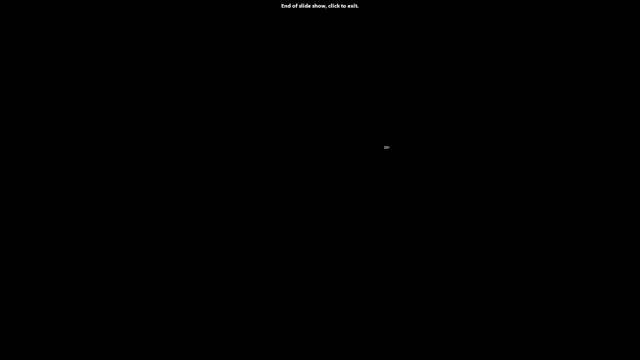 seismology. Thank you very much.